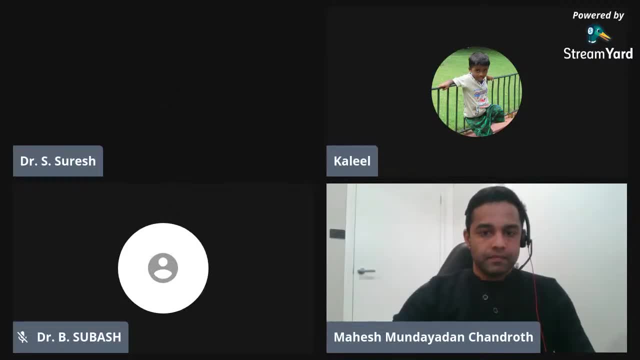 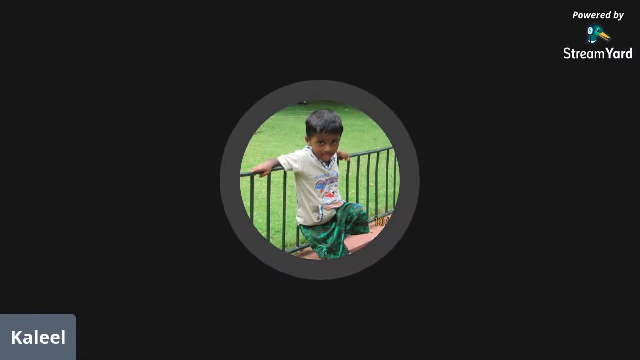 Good morning and warm greetings to all respected dignitaries, staff members, my supportive colleagues and dear participants. Good morning to all. I am Mr Kaleel Mohan Ibrahim, Assistant Professor at St Joseph College of Engineering, Chennai. First I welcome our Patrons. respected Chairman. 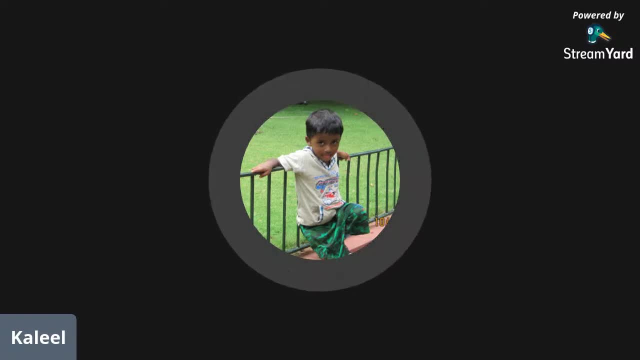 Dr B Babumandokaran, our Managing Director, Mrs S Desipriyav Director, Mr B Sasisekul, Principal, Dr Vatti Sesegriyarov, Dean of Research, Dr V Barodavattin and our Head. 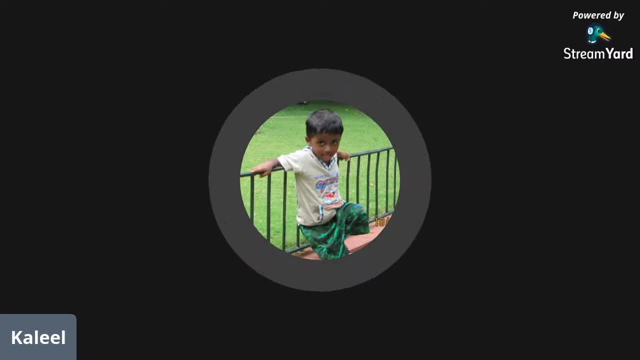 of the Department and Convenor, Dr V Nandini Devi. Most importantly, I welcome all the participants for the International webinar on Radiation in Medicines: Diagnostic Applications of Radiation, organized by Department of Science St Joseph College of Engineering, Chennai. 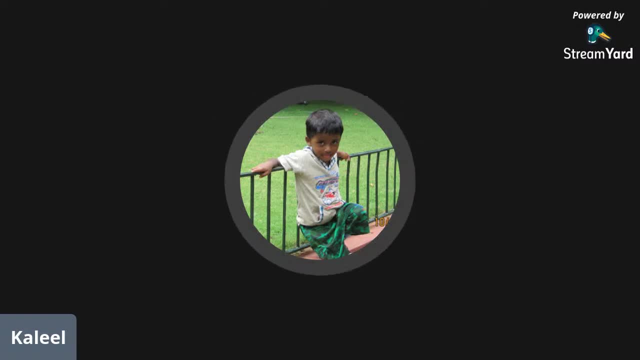 Foremost, we thank God Almighty for giving us this opportunity to conduct the event and make it a great success. A few words related to the webinar before commencing session. Radiation has been used to create visual images of the inner body to diagnose the medical 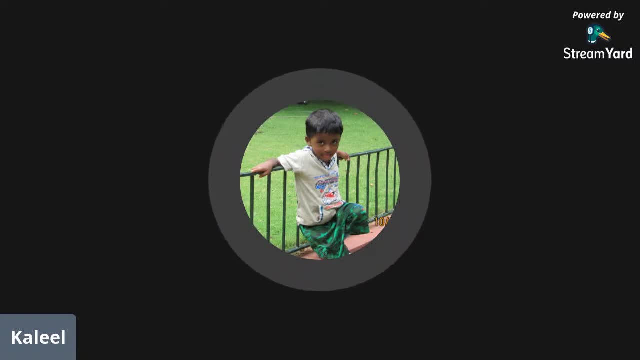 conditions. Medical procedures using radiation have saved more thousands of lives through the detection and the treatment of conditions ranging from hypothyroidism to all types of cancers. There are so many conferences, webinars, faculty development programs and workshops happening. Thank you. To enhance the clinical benefits of radiation. this is one such program, which is going to enlighten you with the knowledge of radiation application in medicine. using imaging tests, Radiations are used to diagnose and treat some medical conditions. We are going to learn how the radiations are used to diagnose and treat the diseases in this session With a. 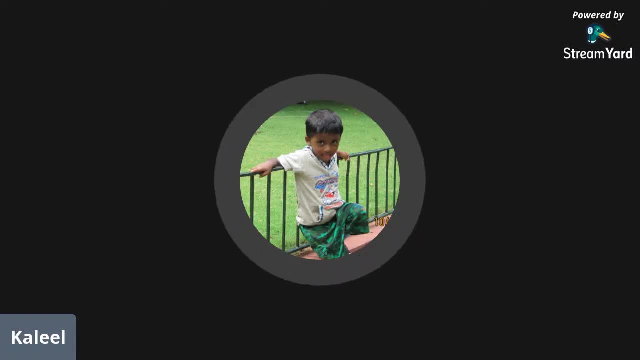 short note. I would like to thank Dr Vatti Sesegriyarov, Dean of Research, Dr V Barodavattin and Dr Amit Shah. I would like to call upon Dr B Subhas, Ascent Professor, St Joseph's College of Engineering. 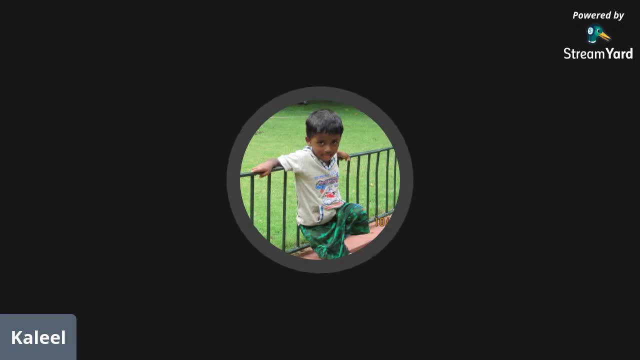 to introduce our guest of honor of our webinar. Thank you all for the support and participation. Have a great day. Thank you, sir. Thank you, sir. Good morning to all, all the respected dignitaries, staff members, my dear colleagues and enthusiastic participants. Welcome to the International Webinar on Radiation. 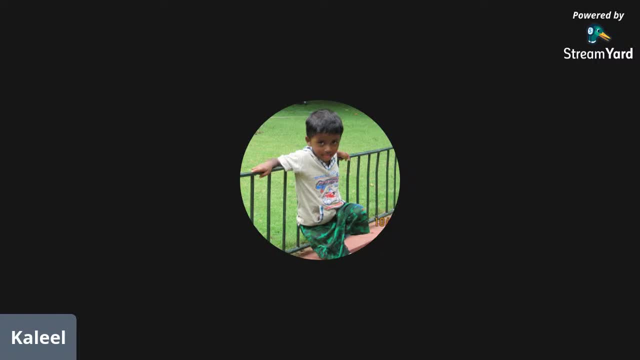 in Medicine: Diagnostic Applications of Radiation organized by Department of Science St Joseph's College of Engineering, Chennai. Radiation can be considered as the trigger for the development of radiation. Radiation can be considered as the trigger for the development of radiation. Radiation can be considered. 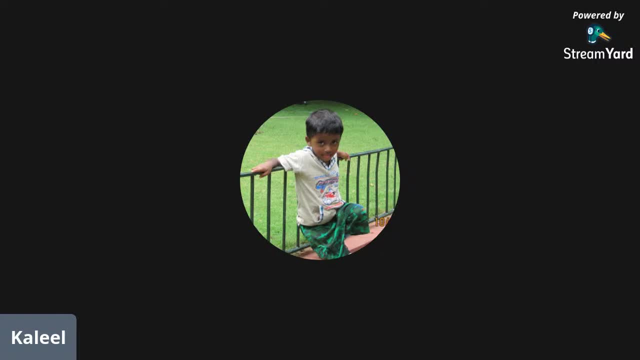 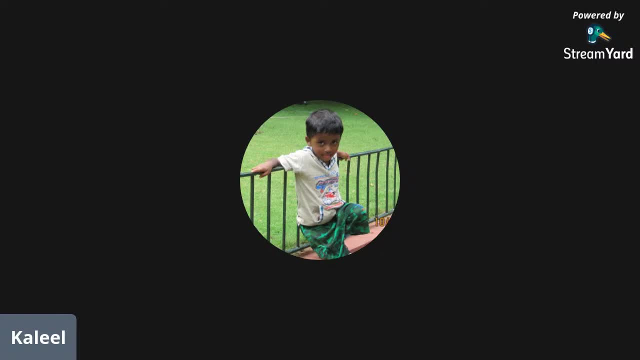 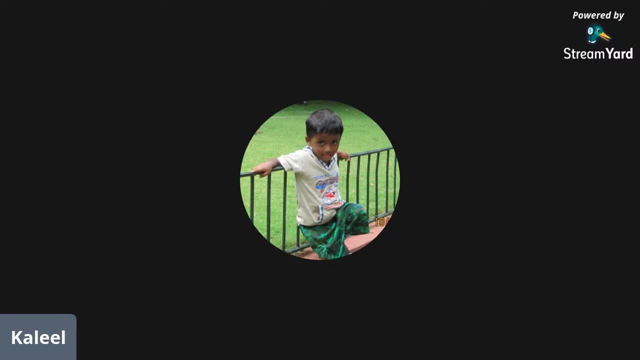 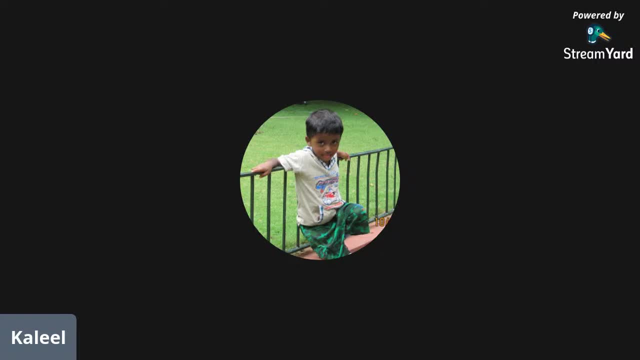 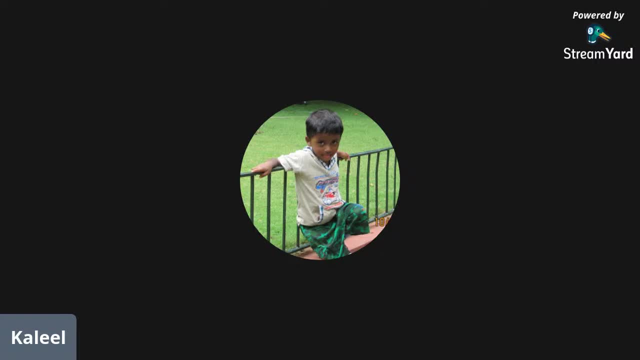 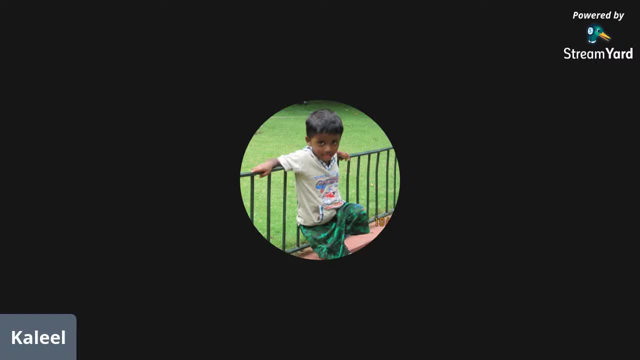 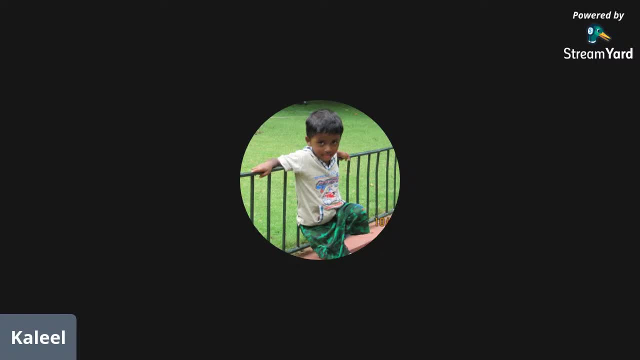 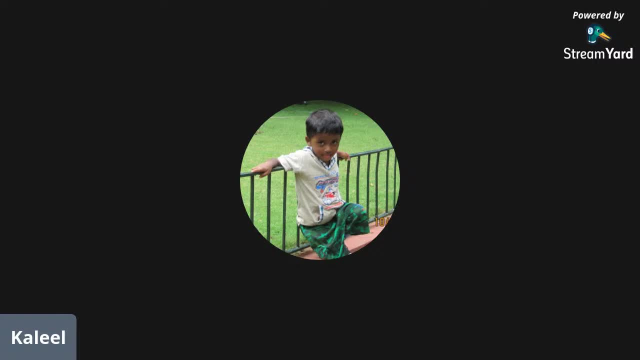 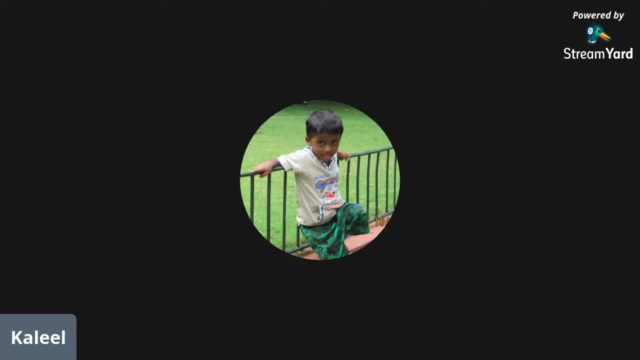 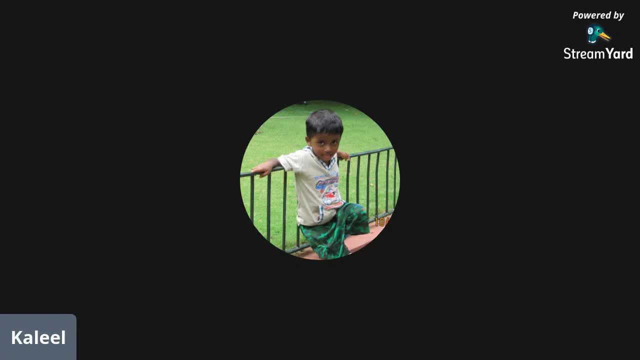 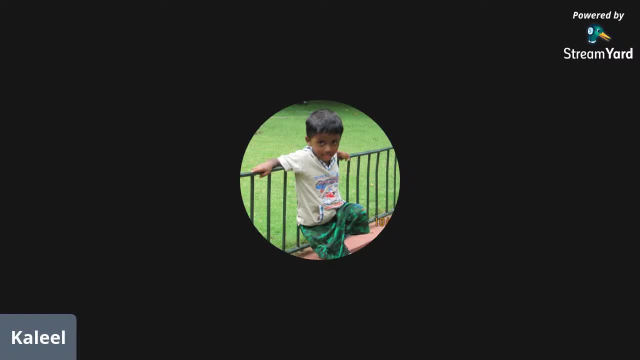 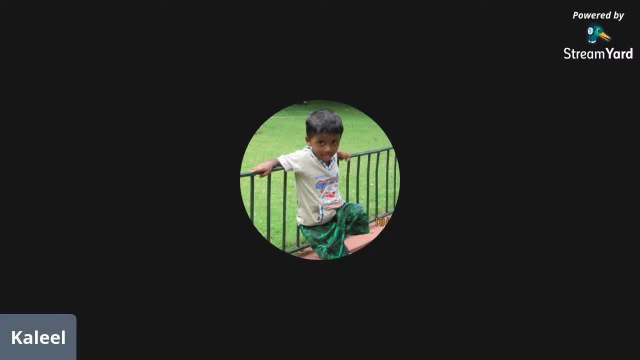 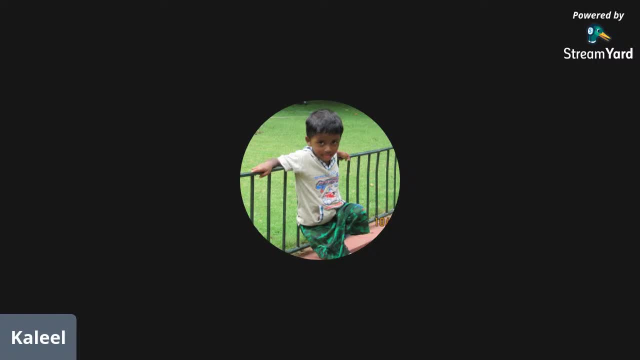 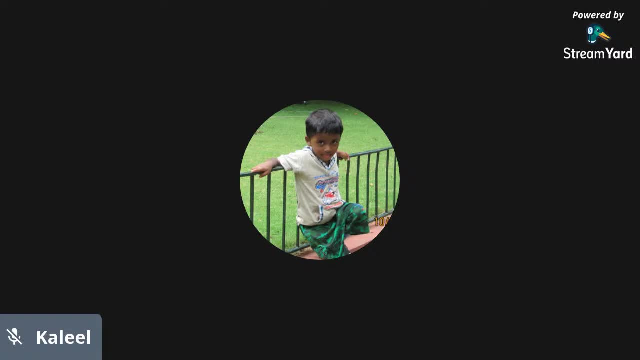 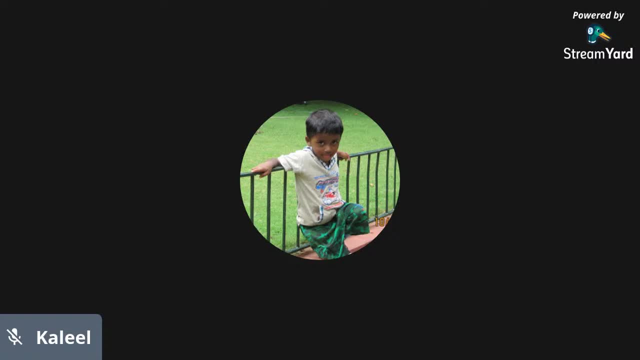 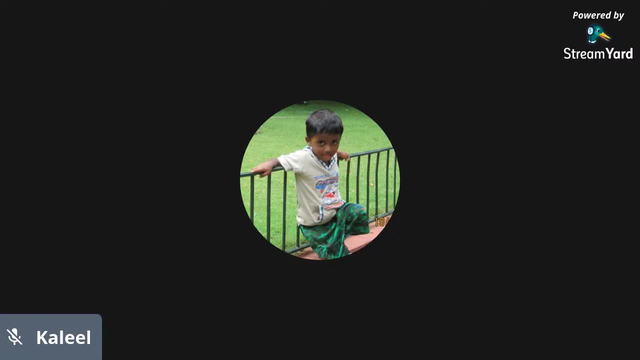 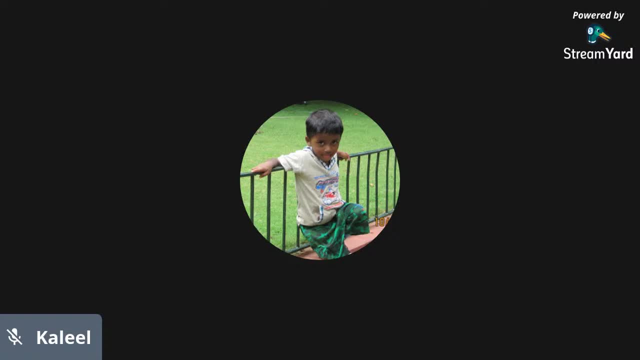 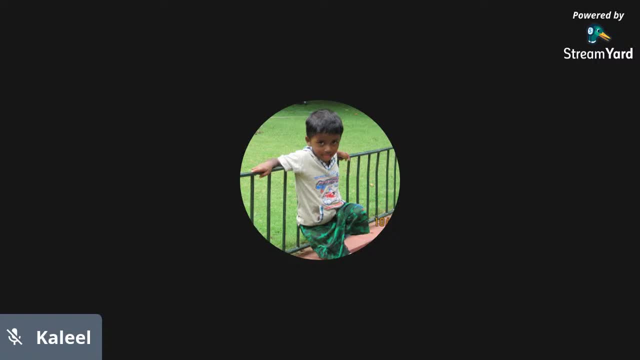 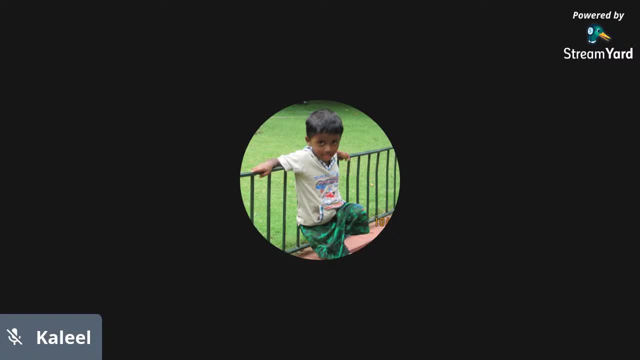 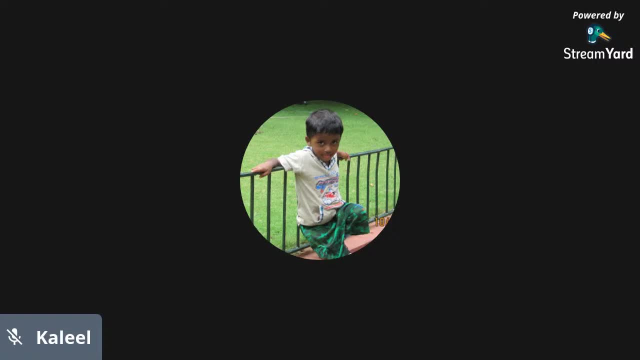 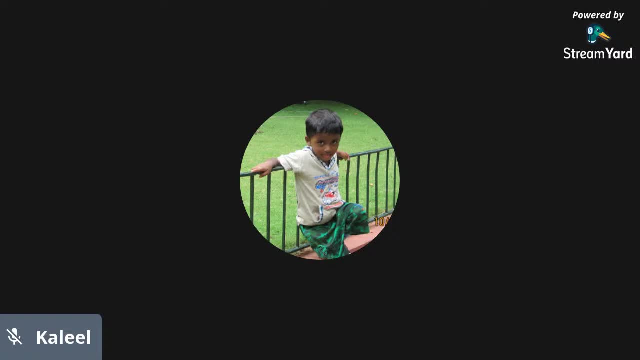 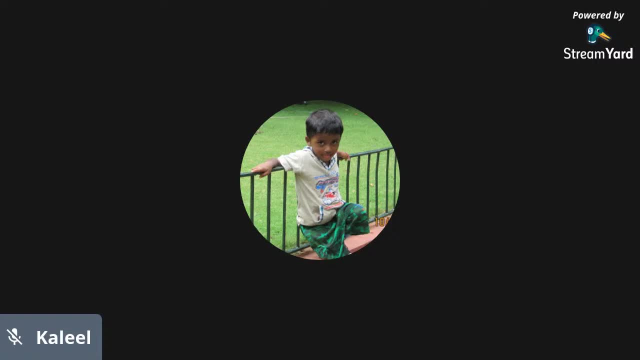 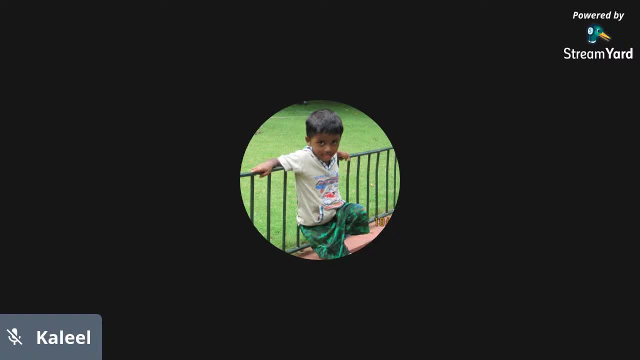 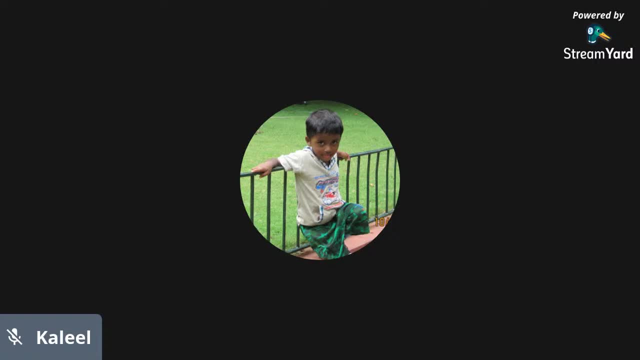 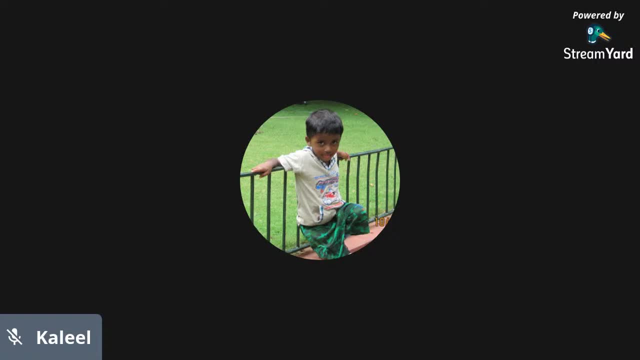 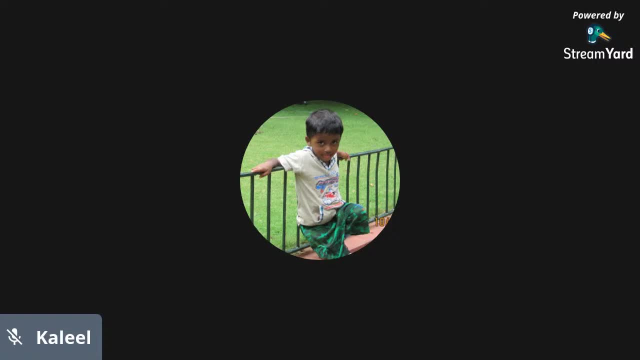 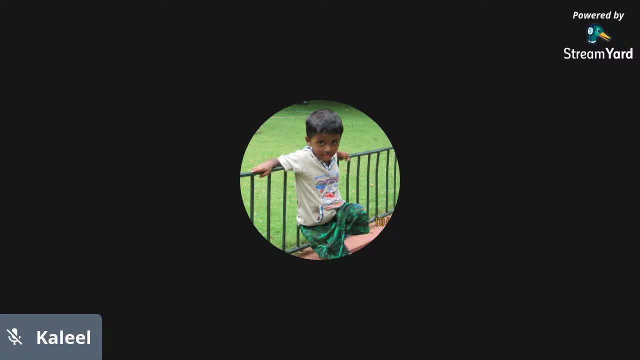 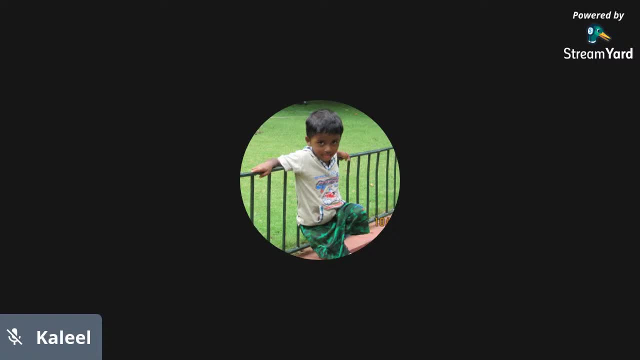 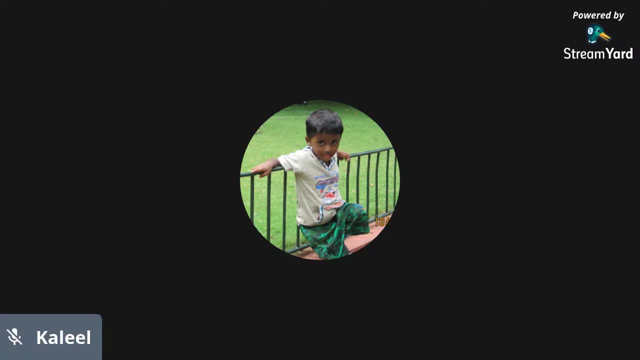 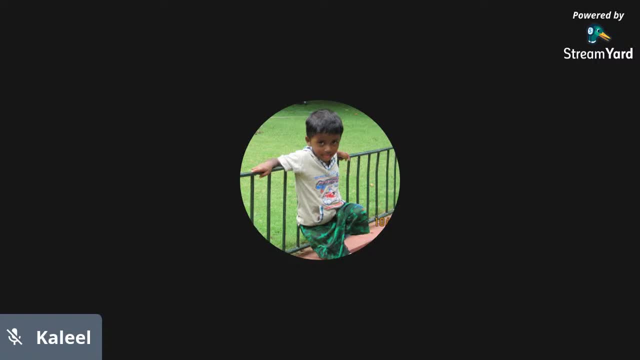 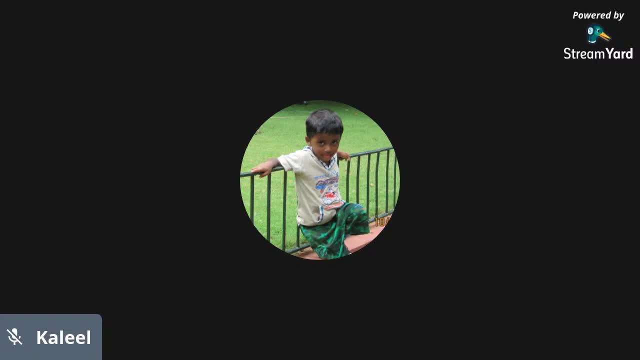 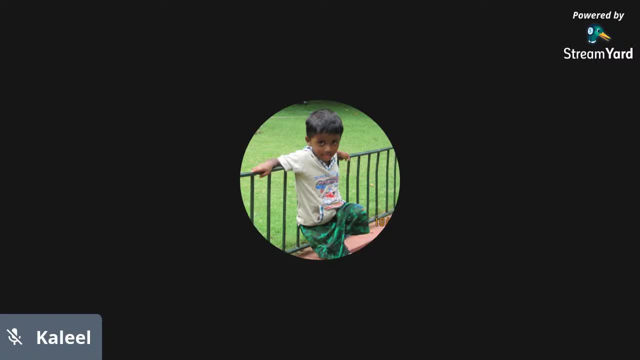 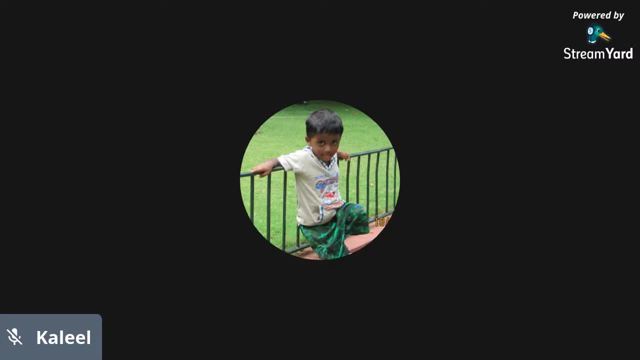 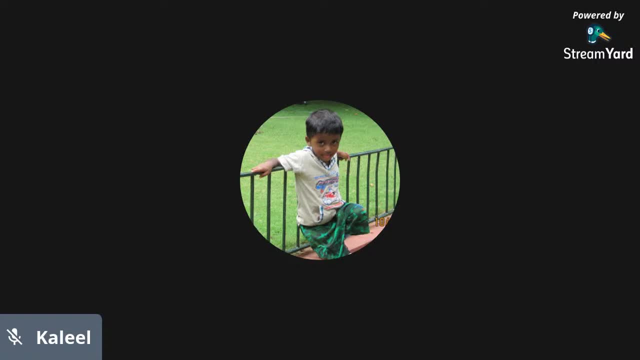 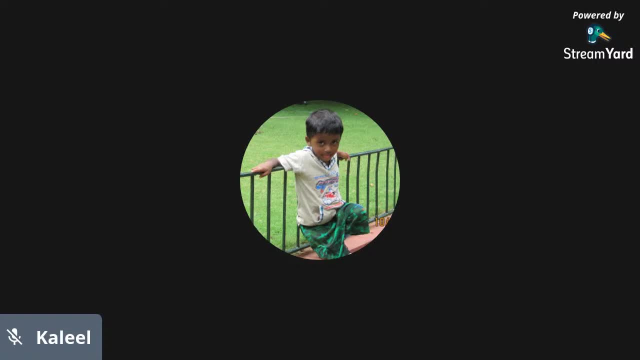 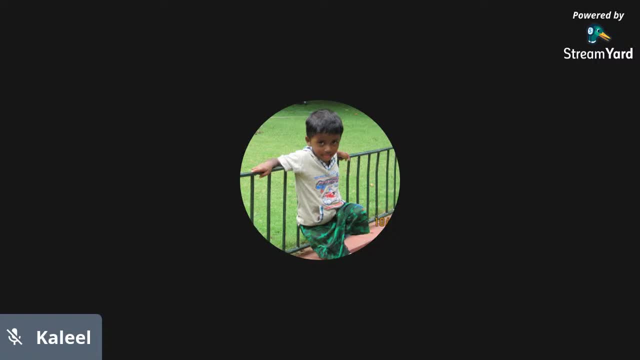 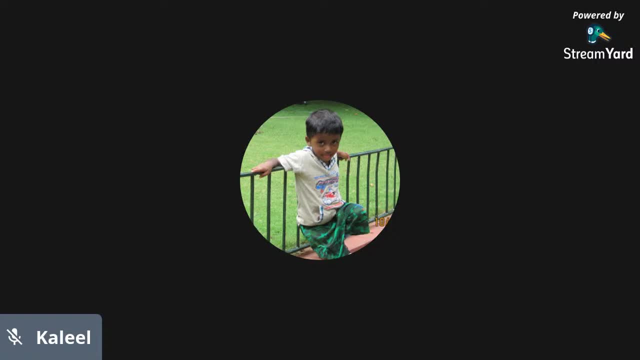 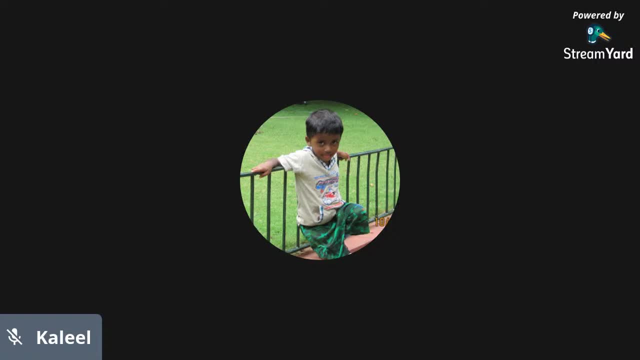 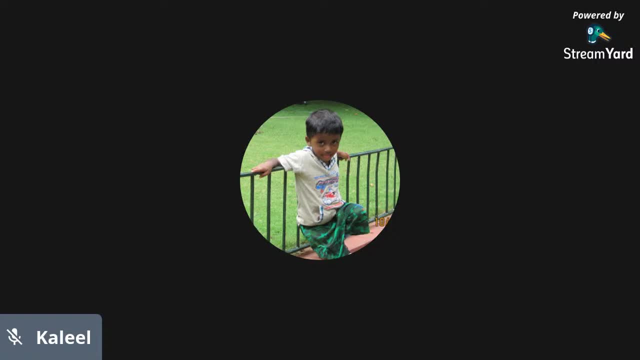 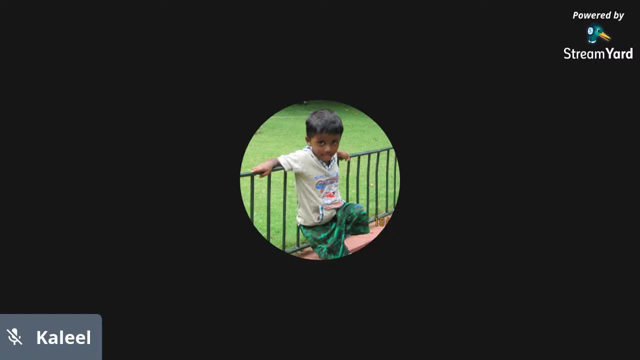 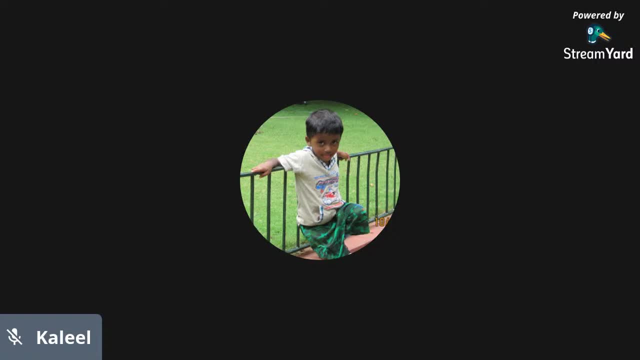 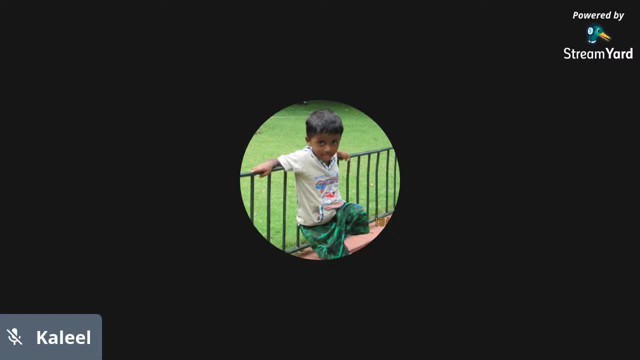 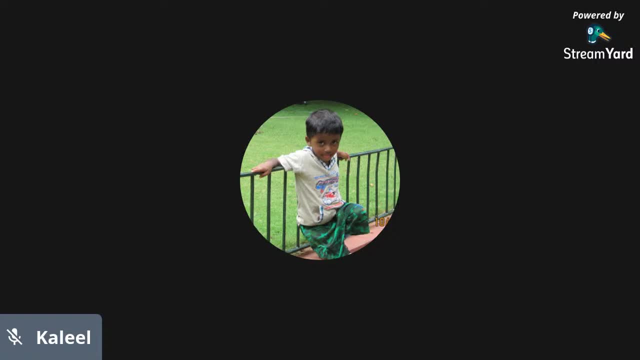 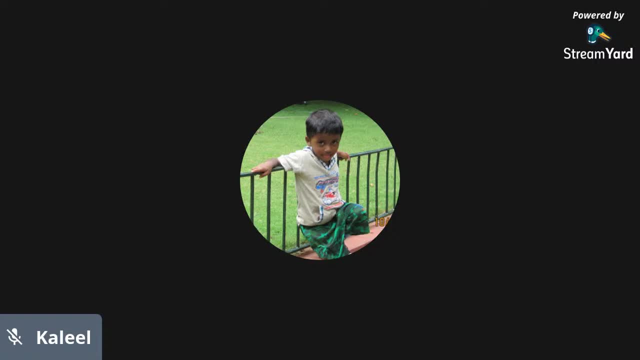 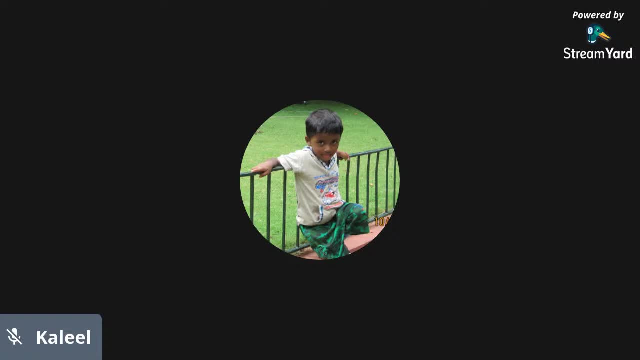 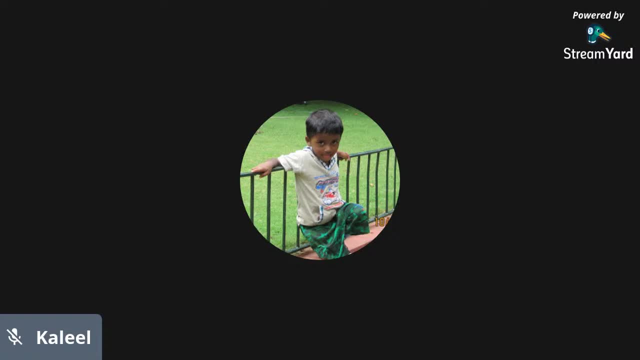 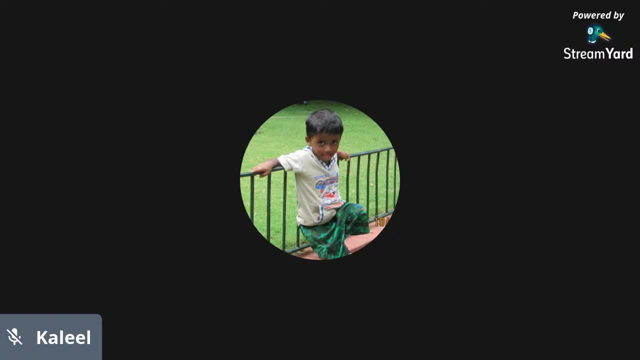 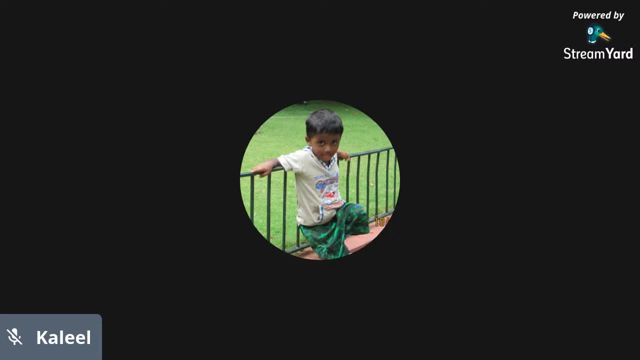 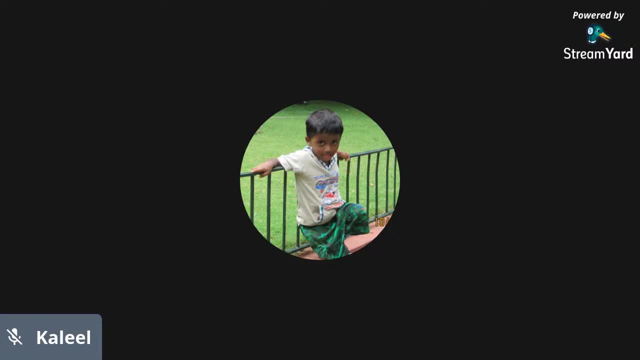 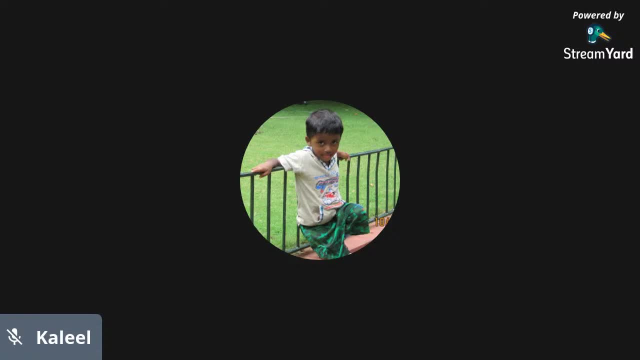 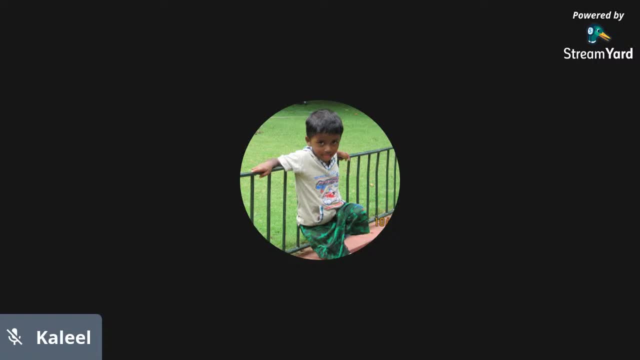 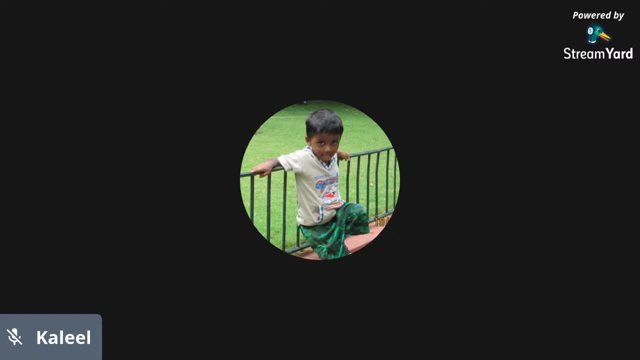 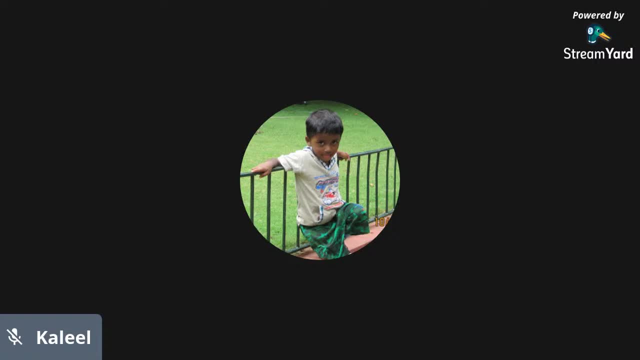 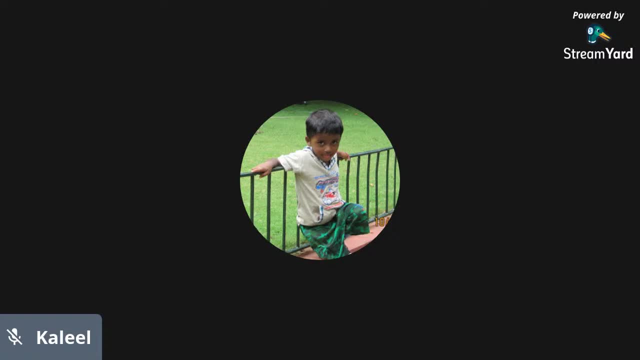 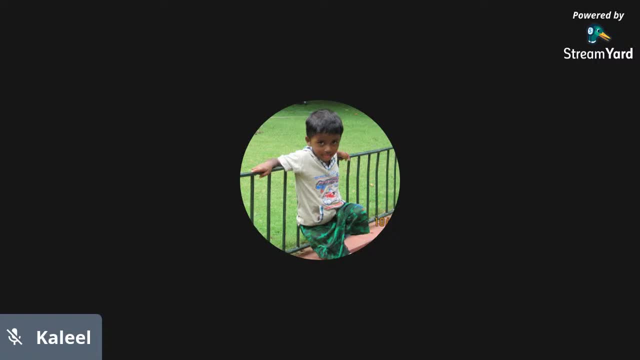 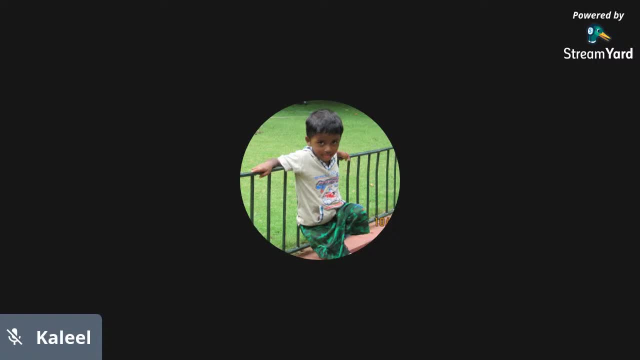 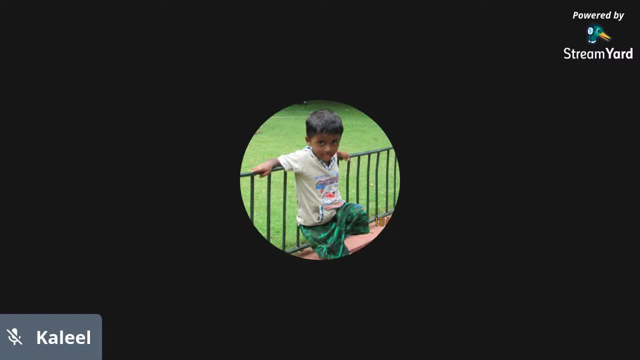 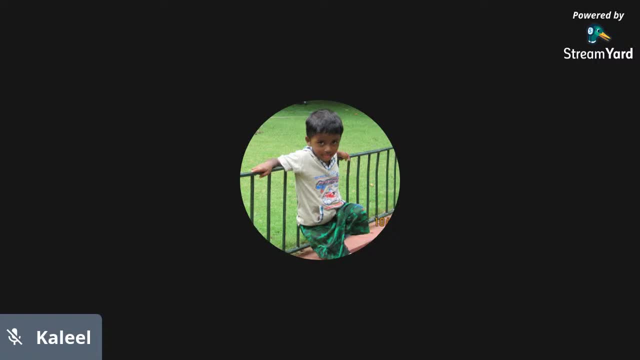 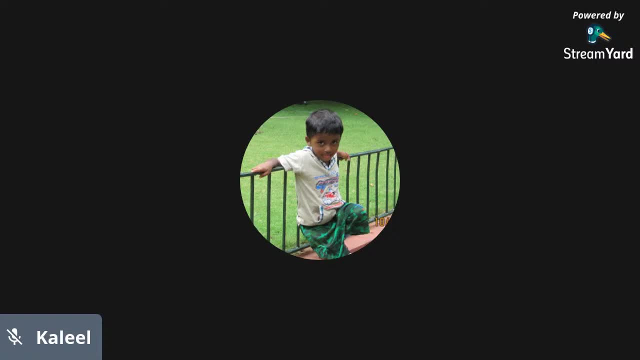 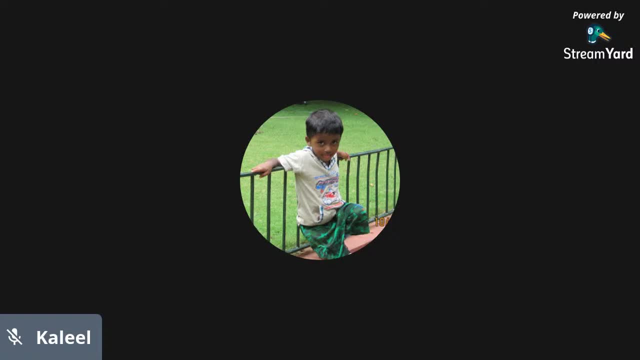 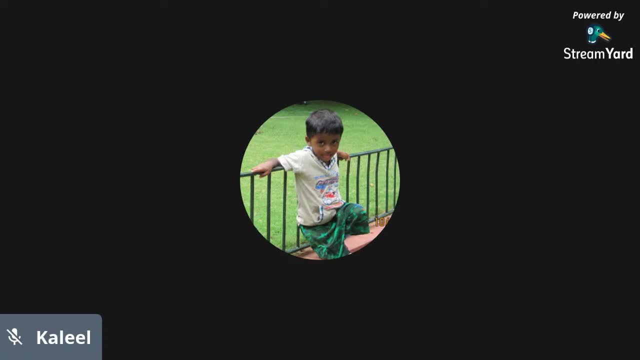 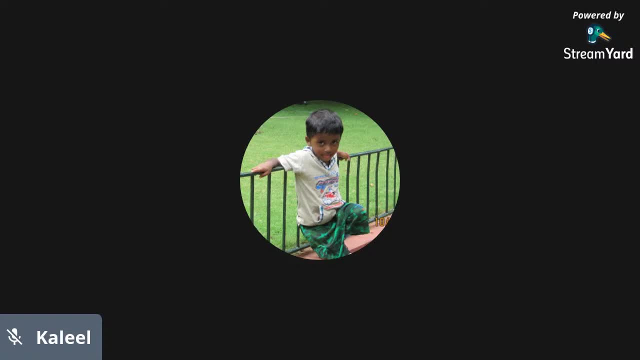 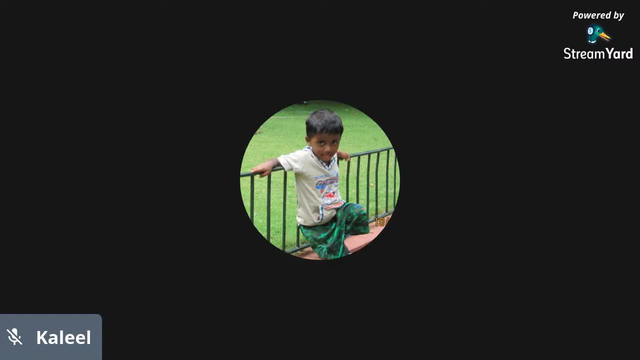 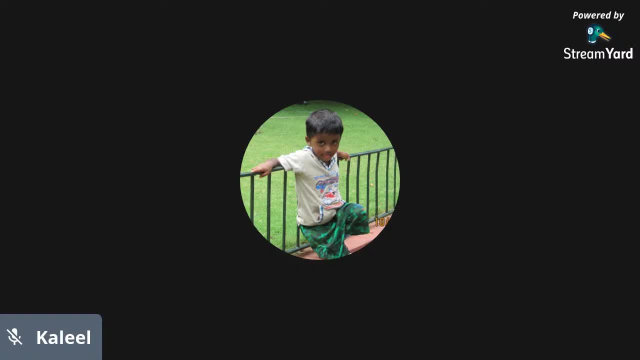 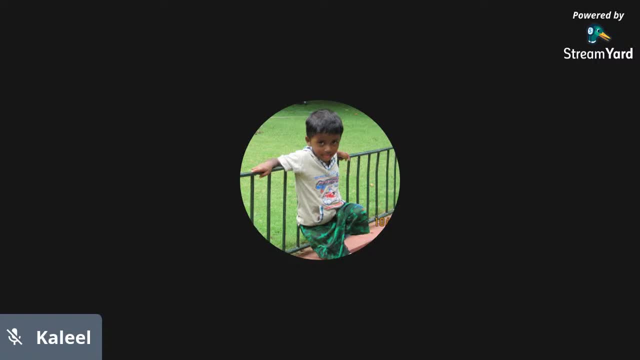 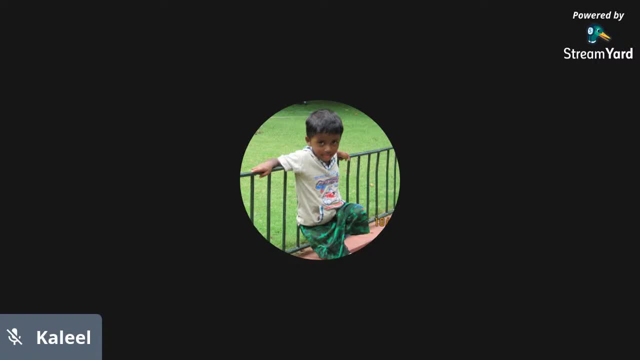 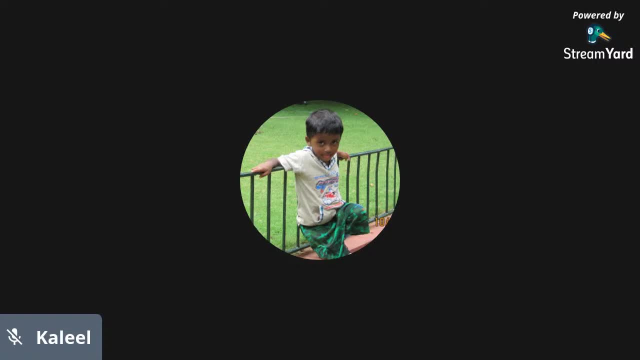 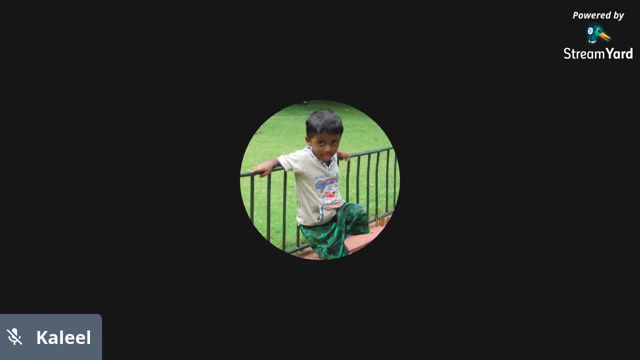 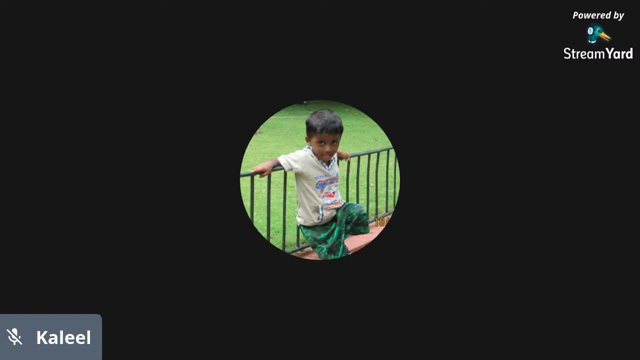 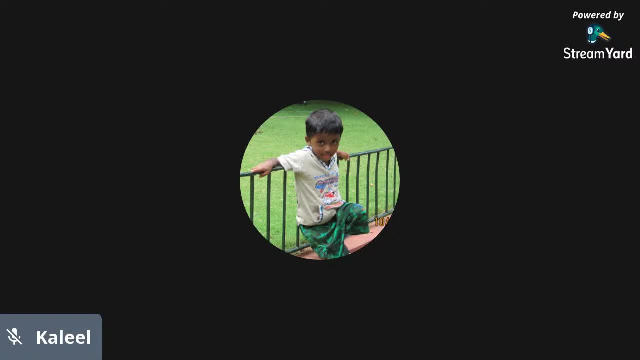 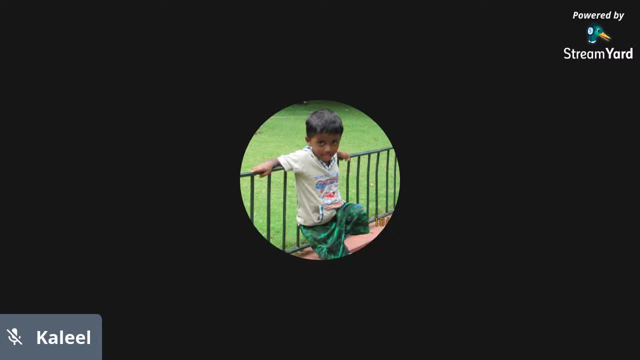 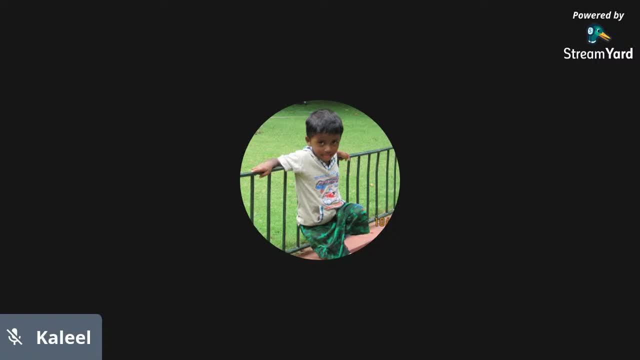 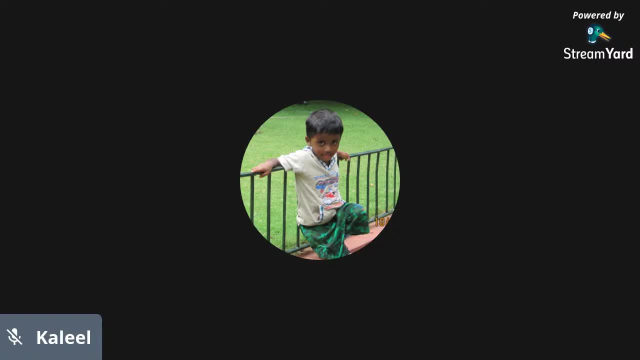 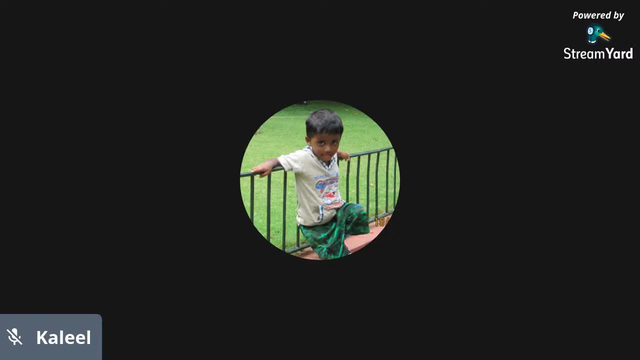 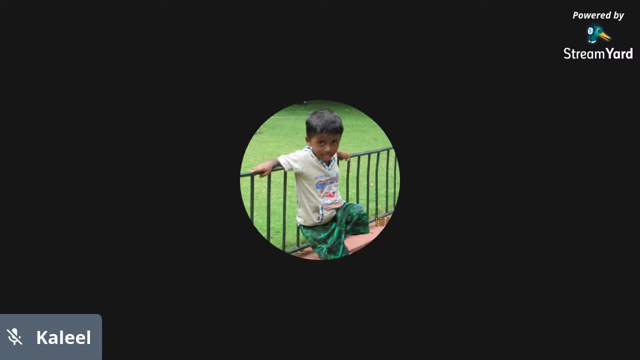 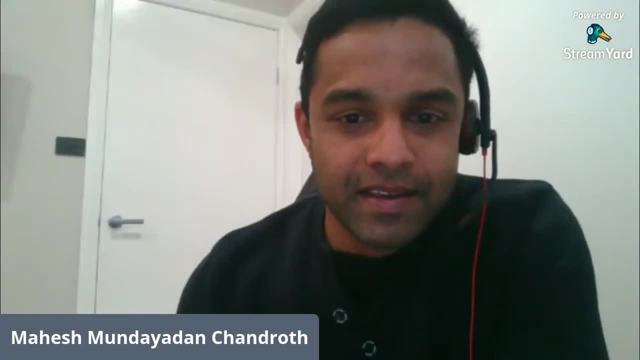 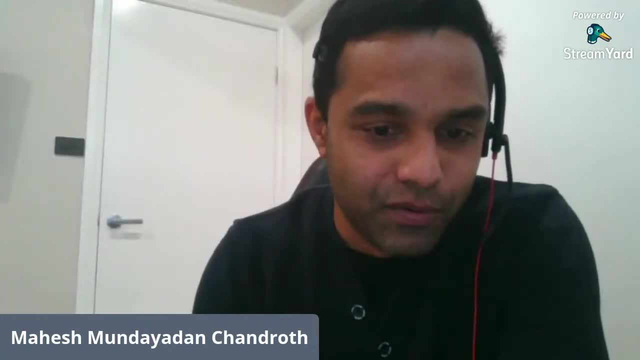 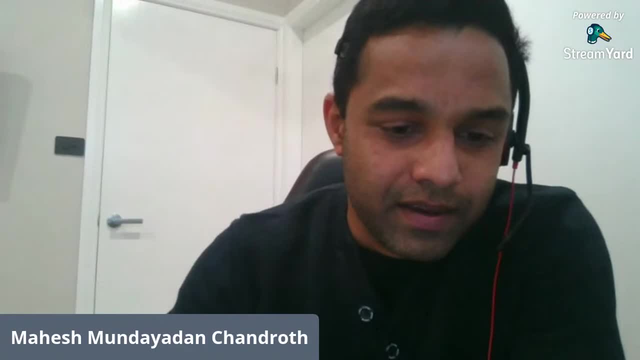 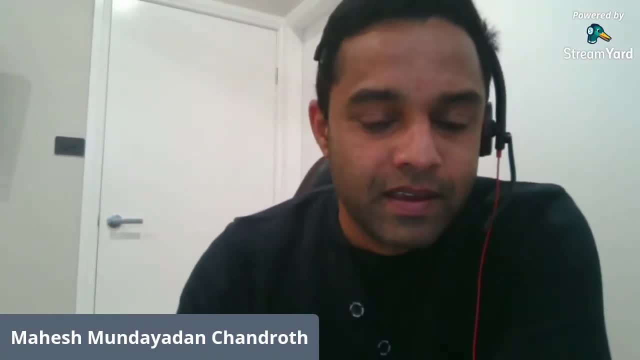 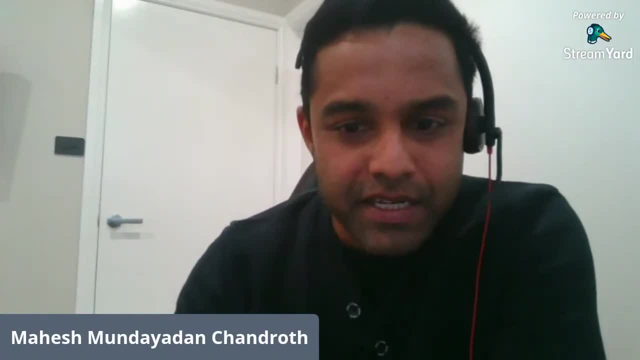 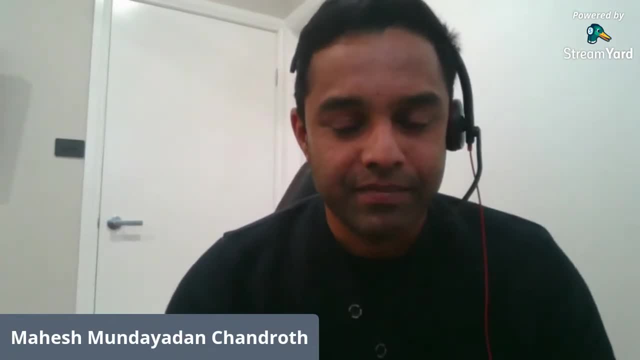 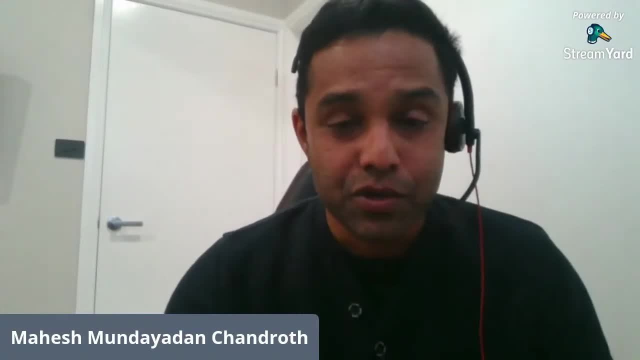 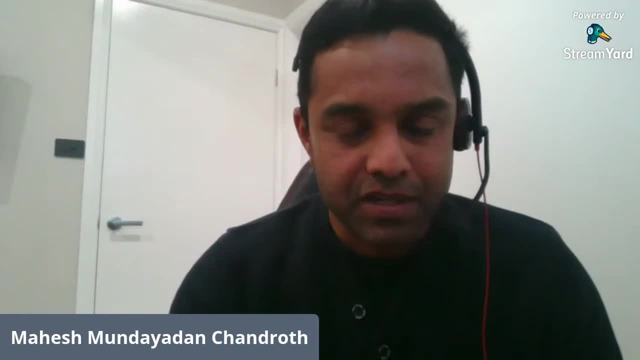 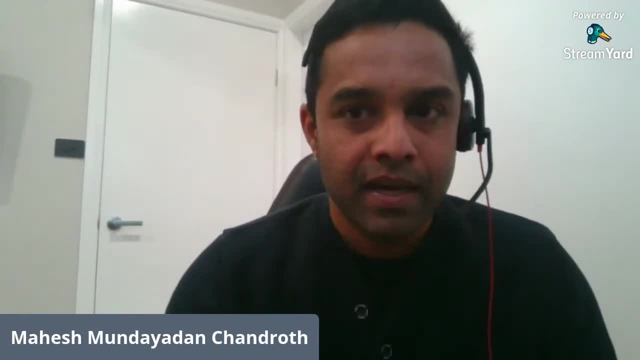 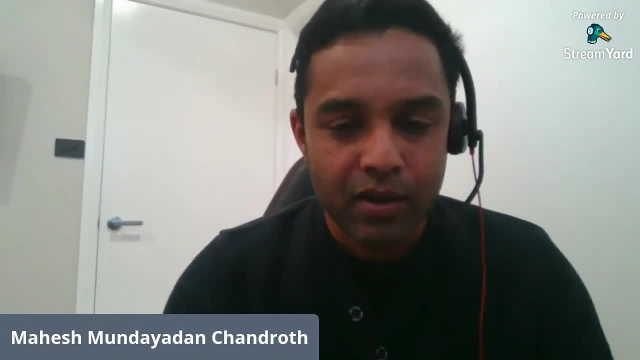 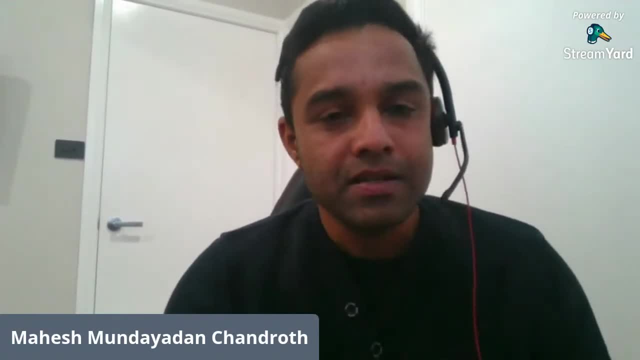 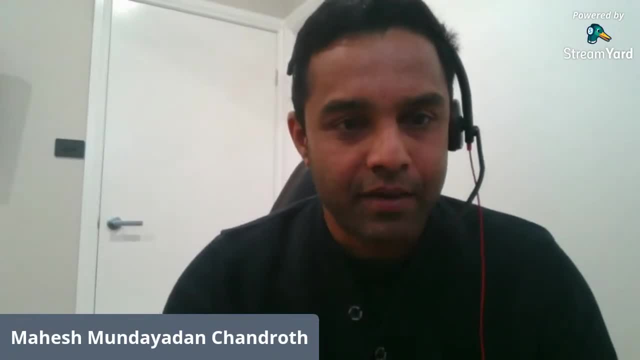 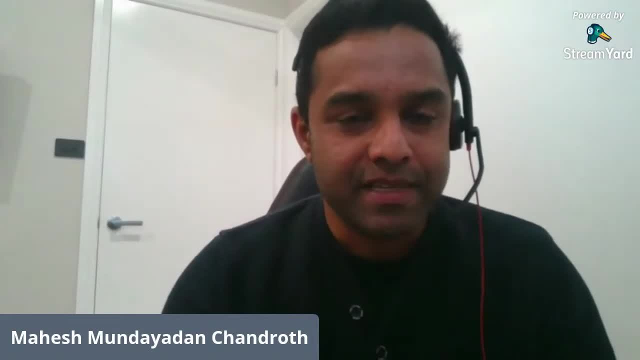 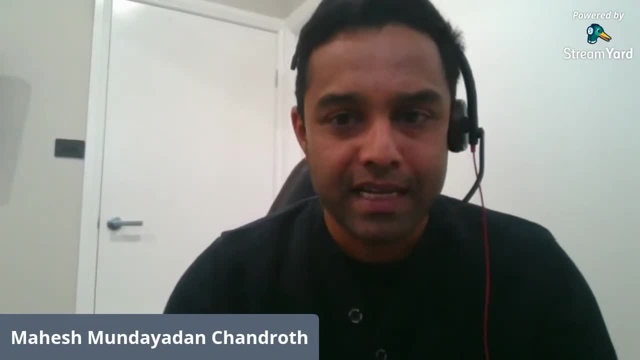 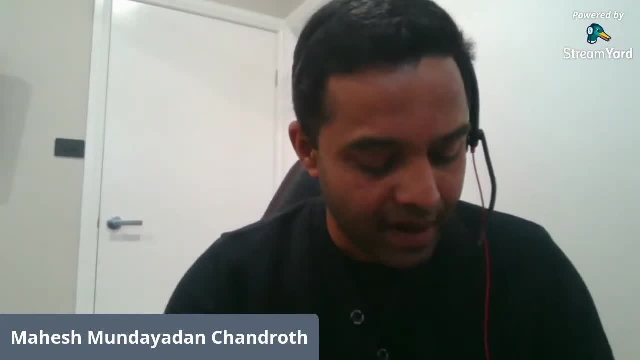 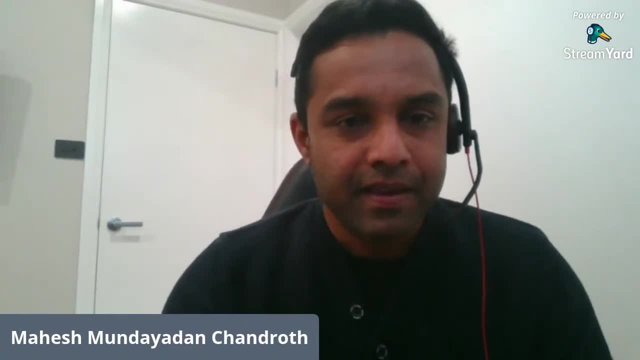 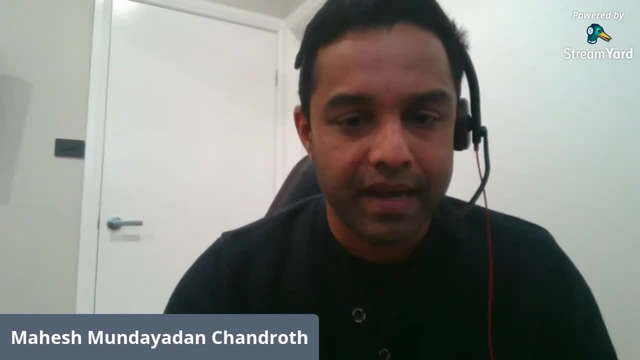 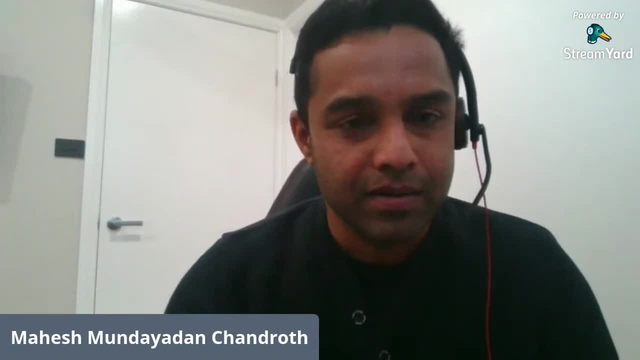 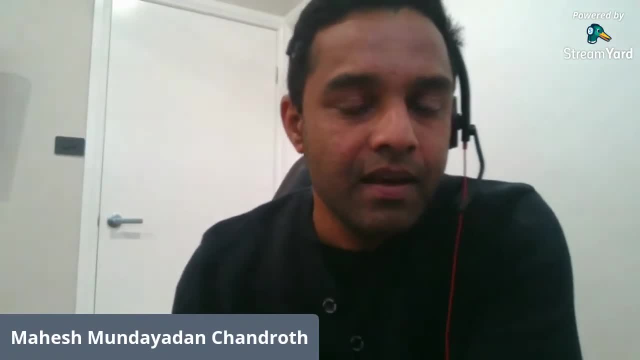 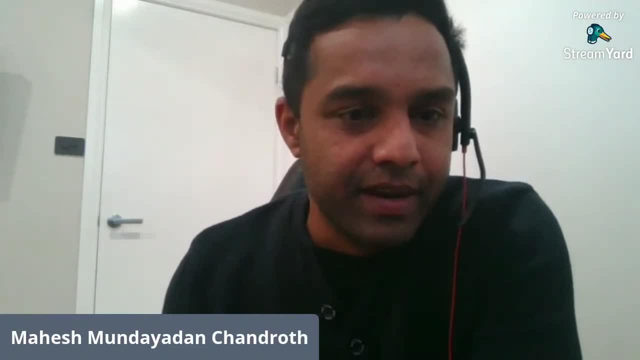 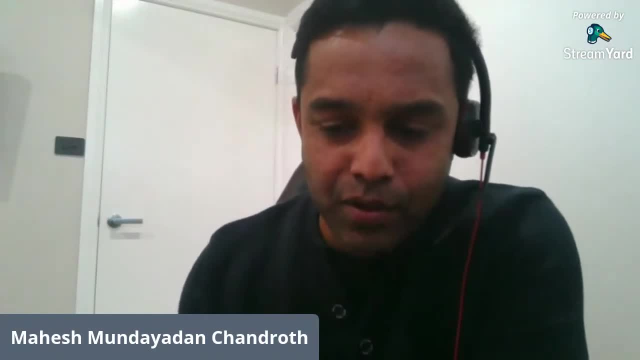 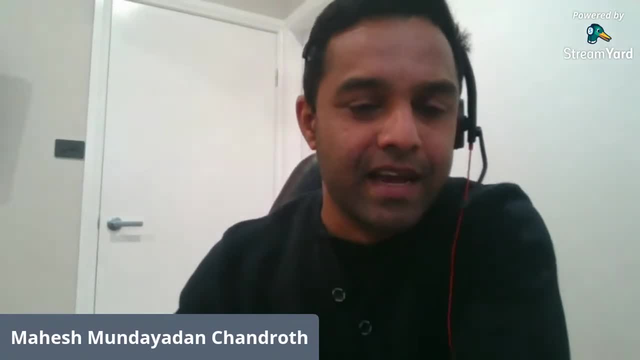 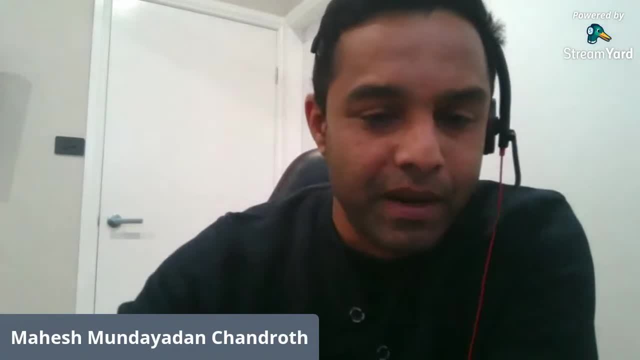 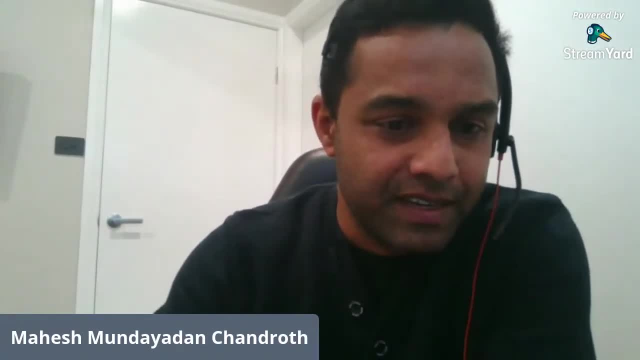 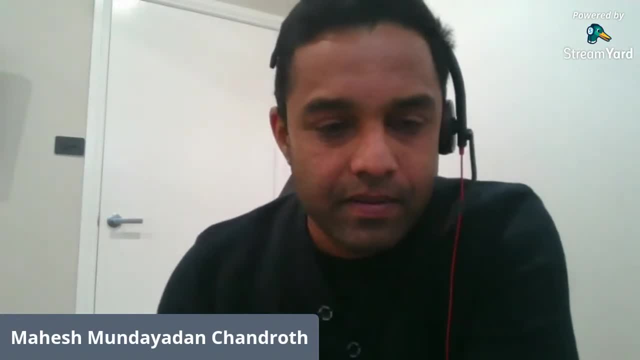 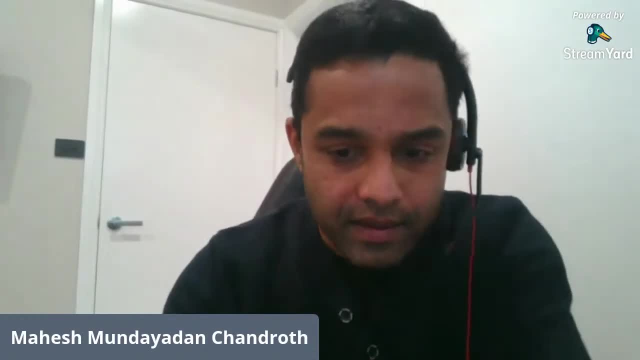 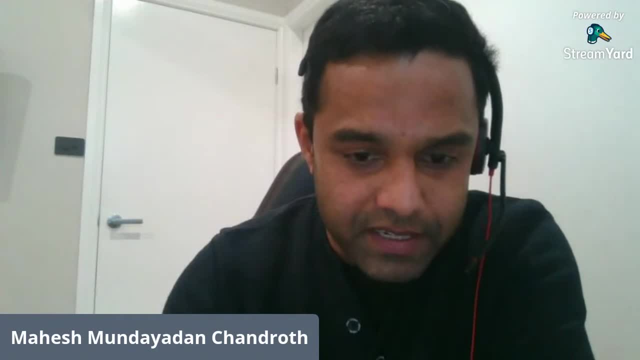 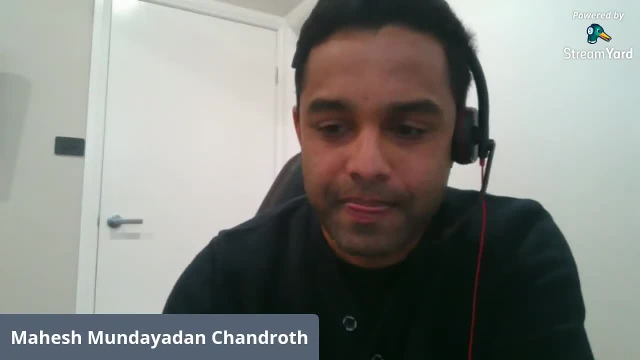 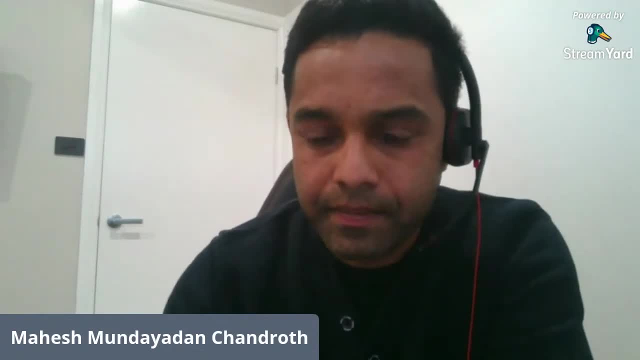 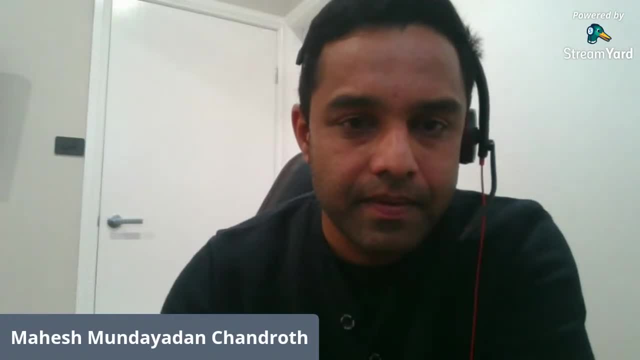 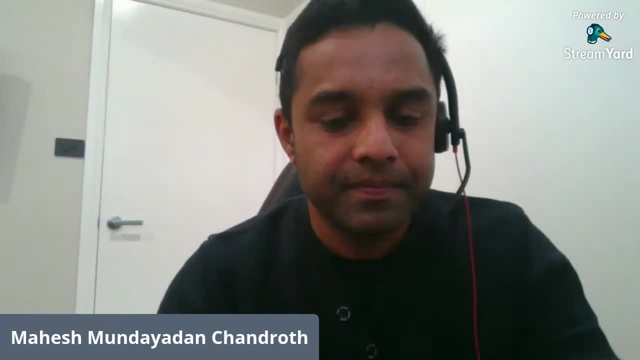 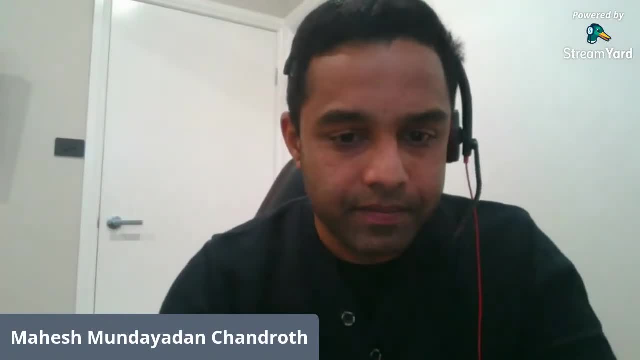 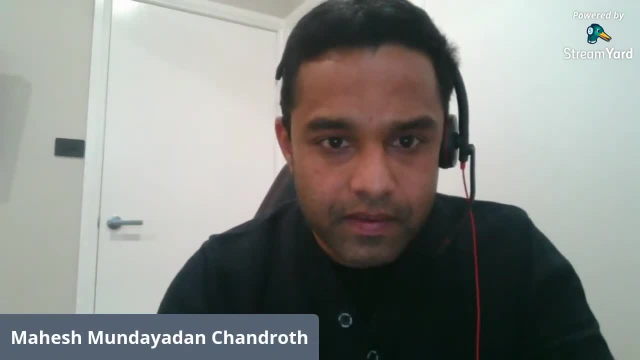 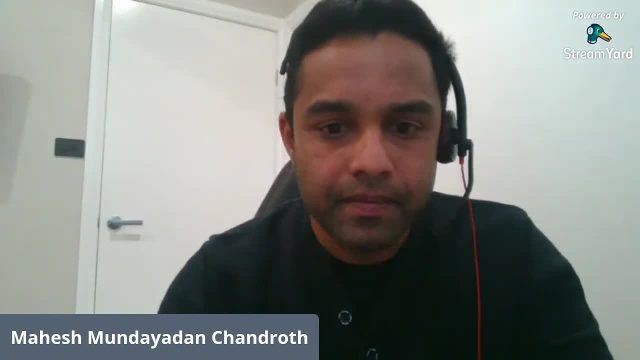 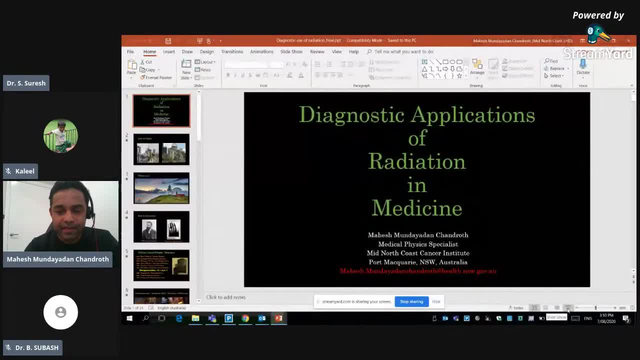 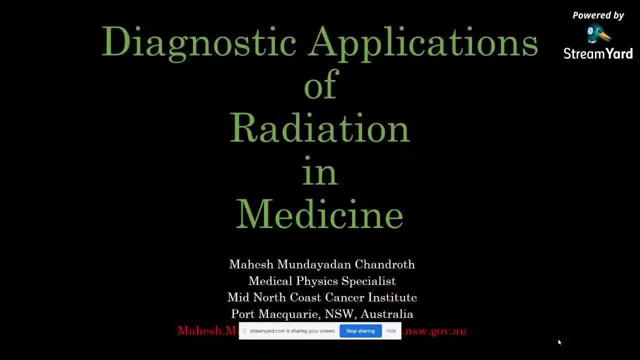 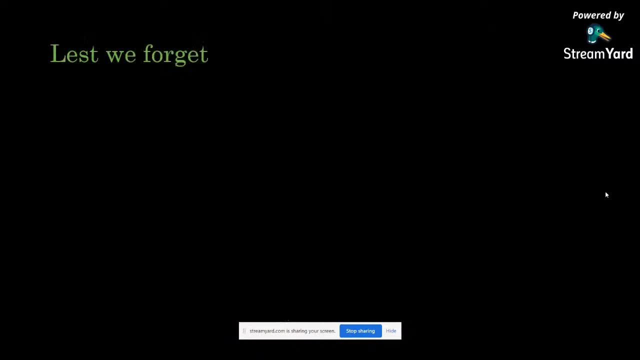 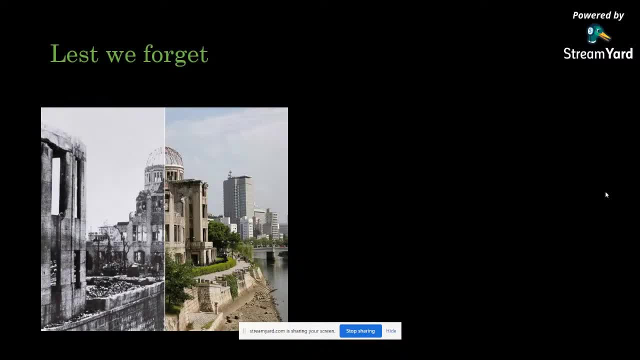 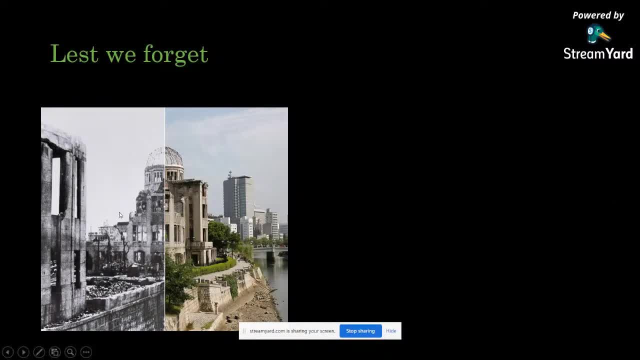 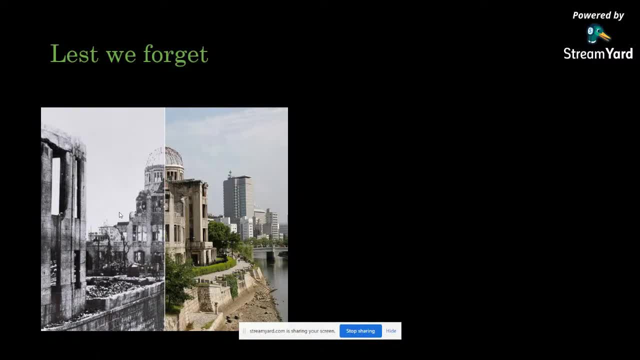 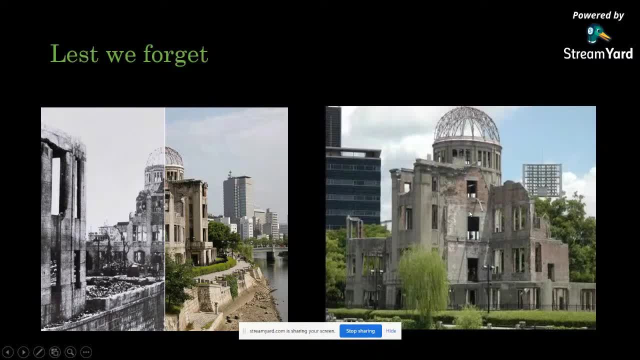 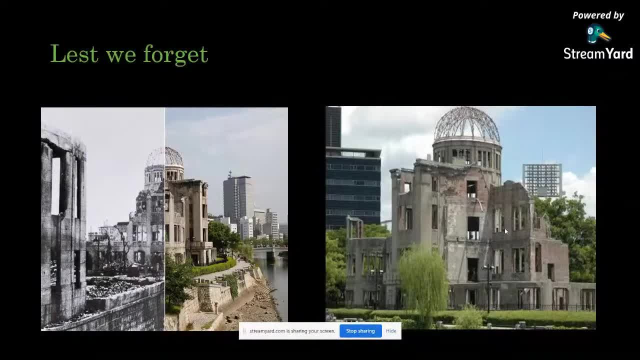 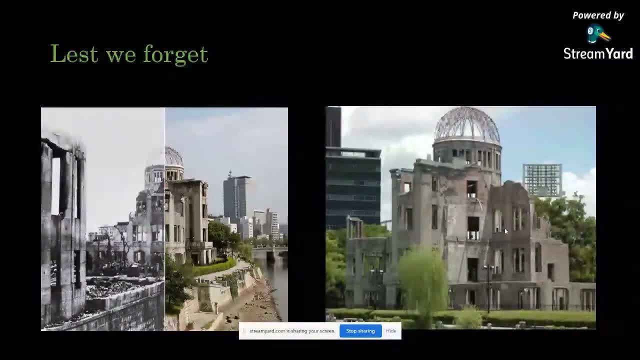 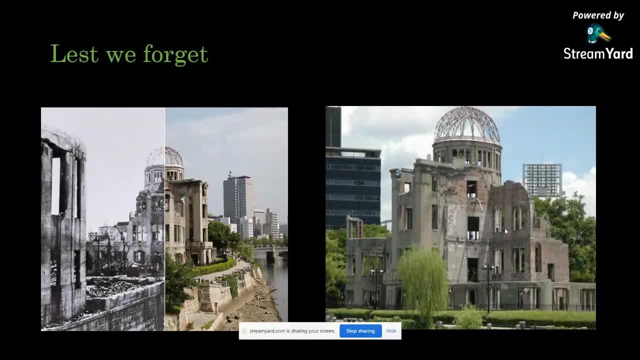 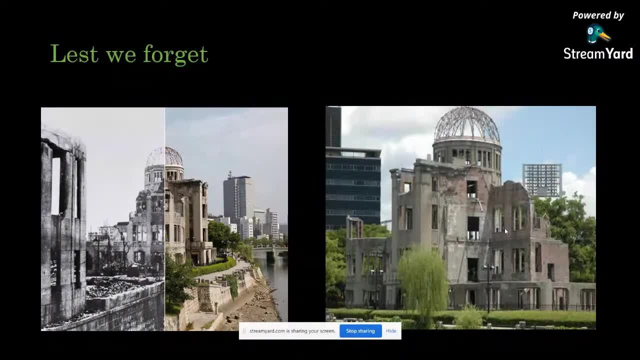 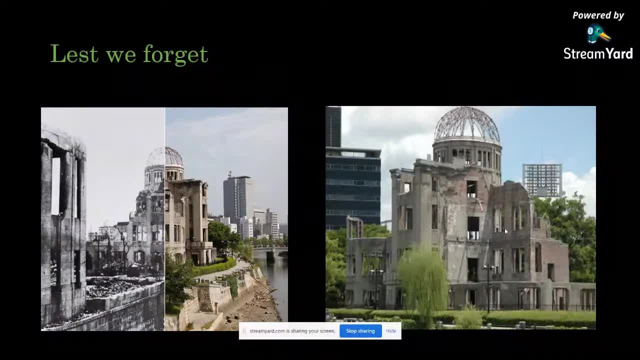 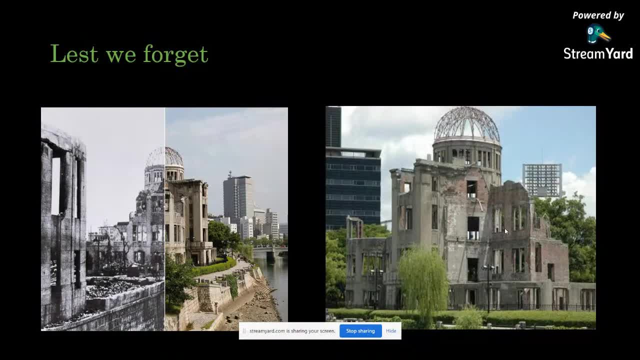 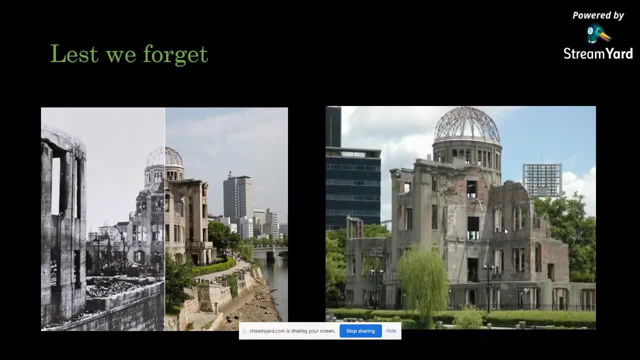 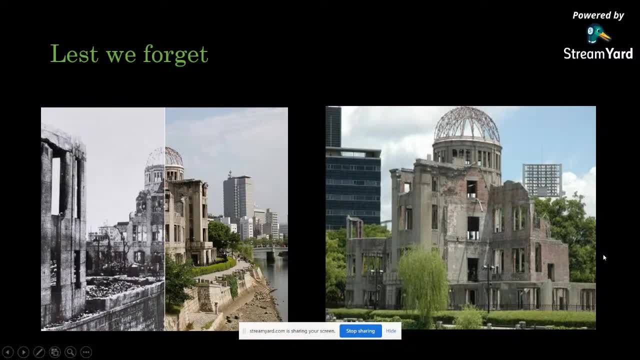 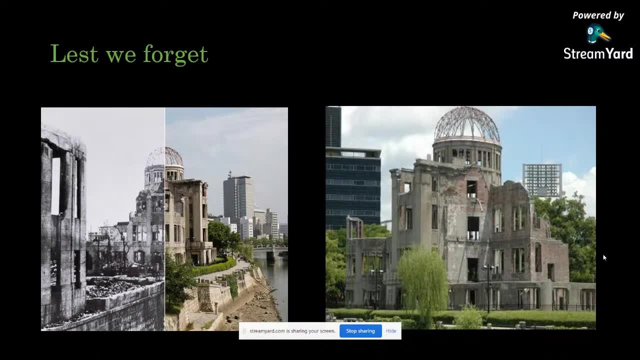 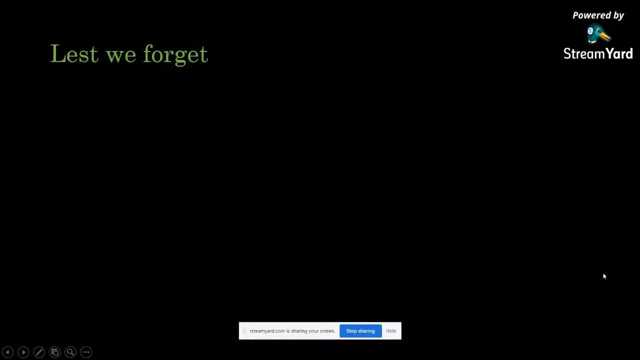 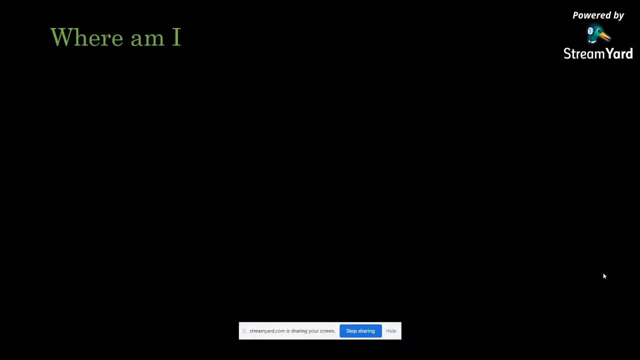 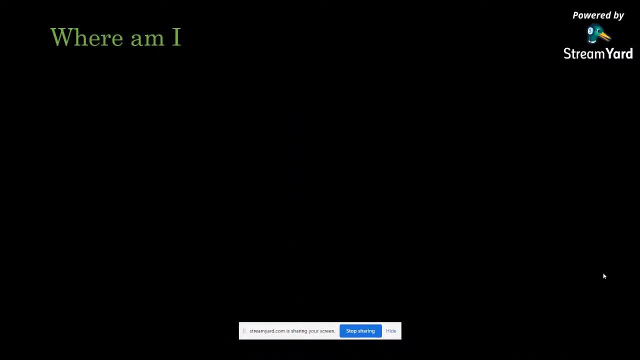 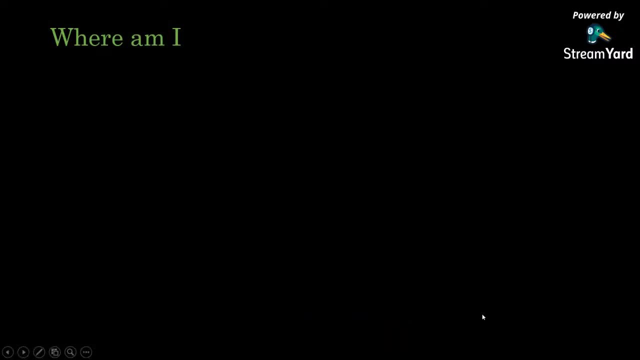 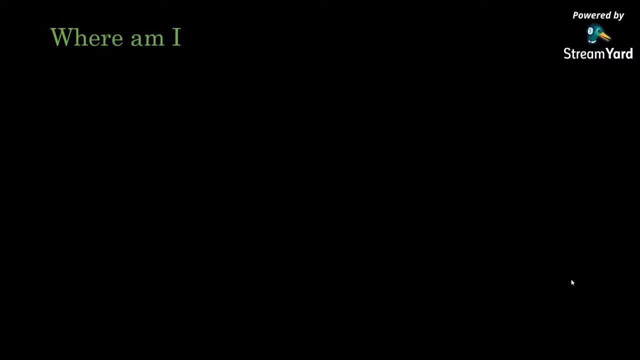 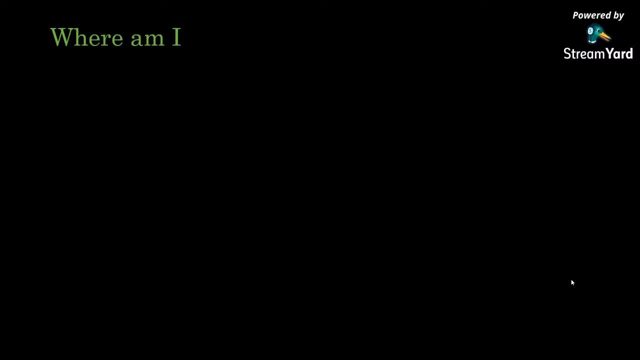 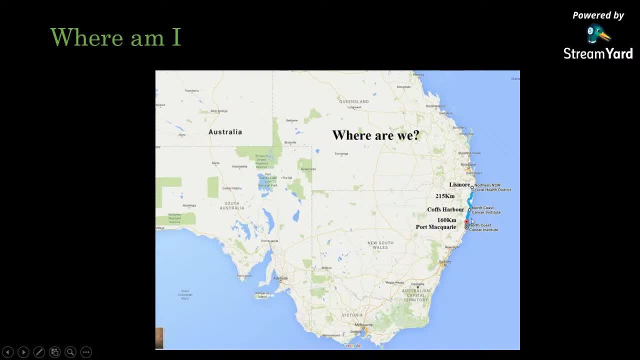 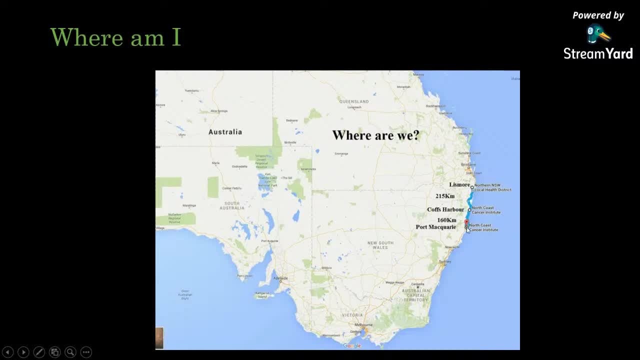 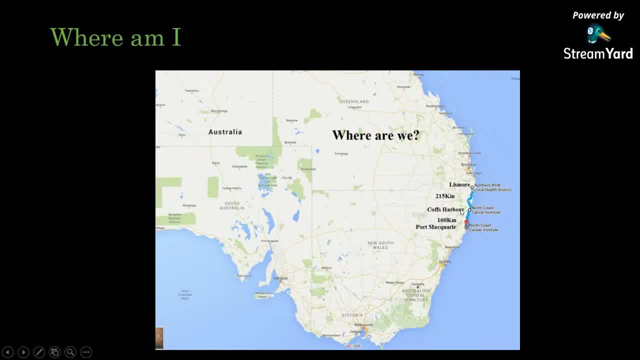 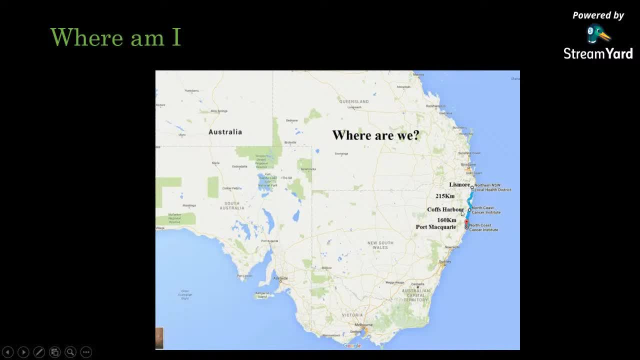 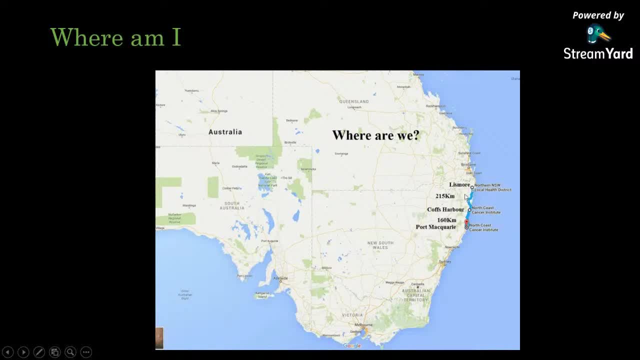 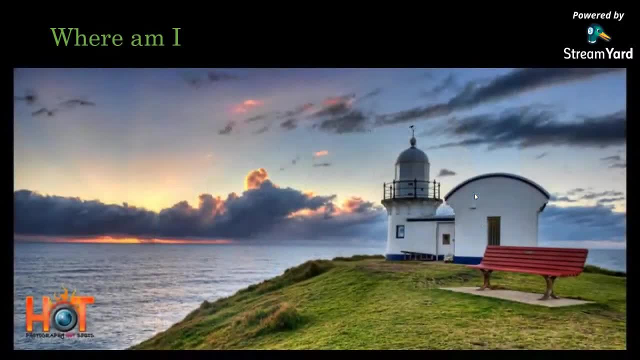 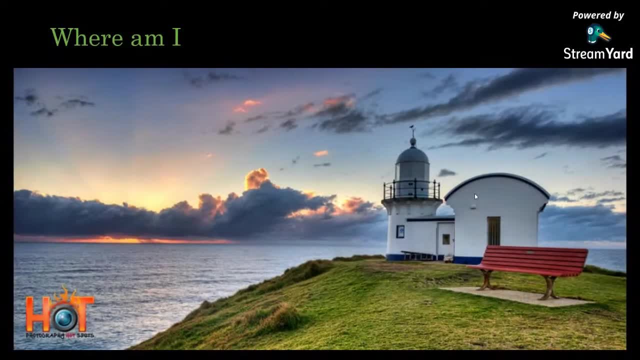 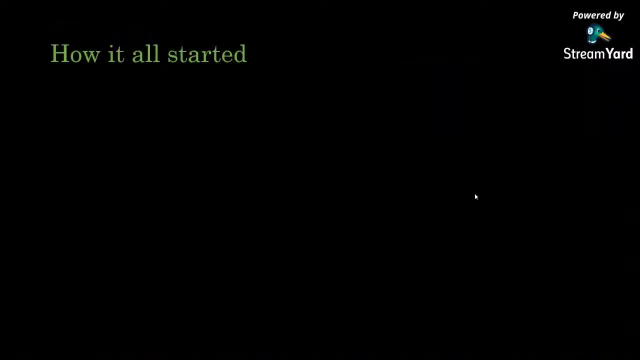 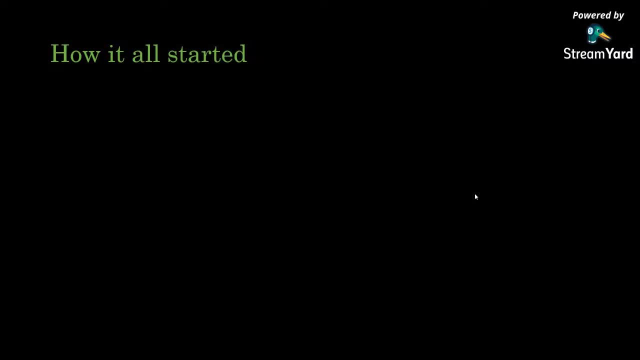 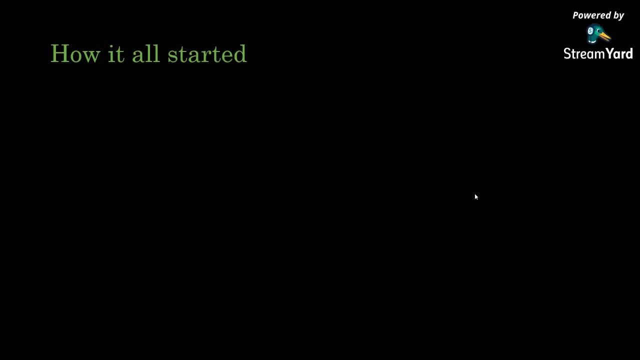 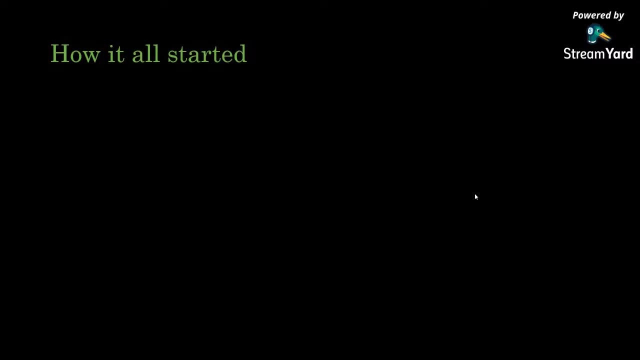 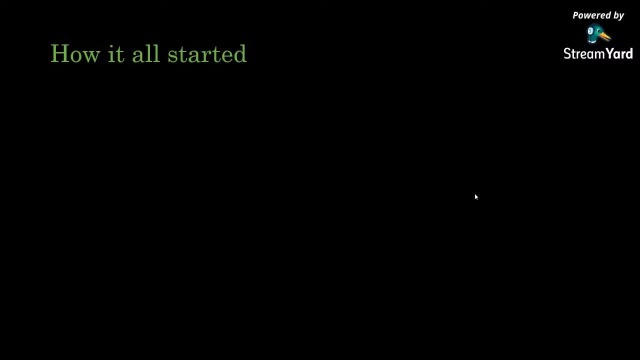 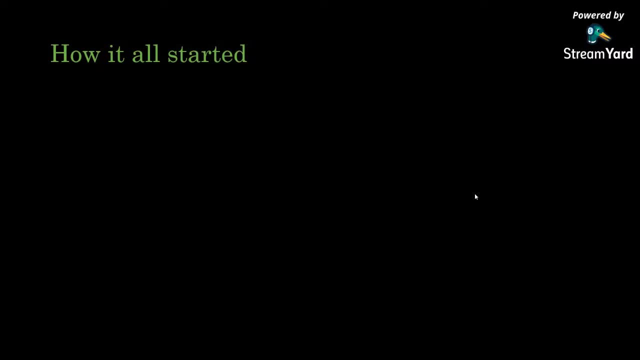 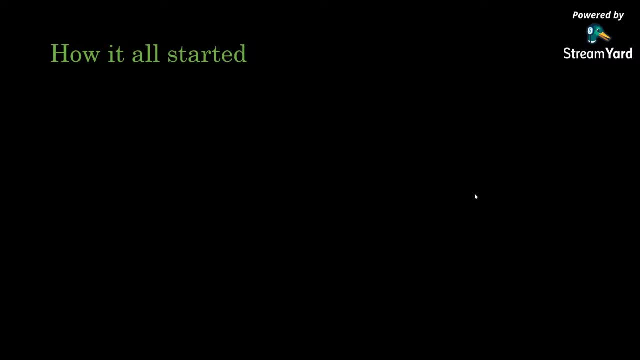 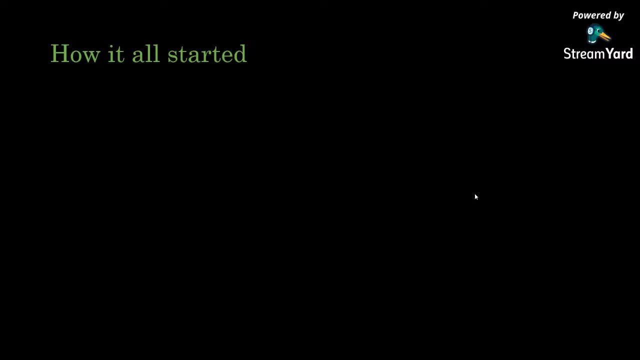 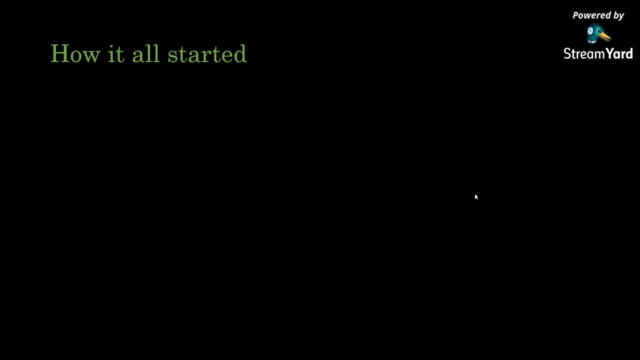 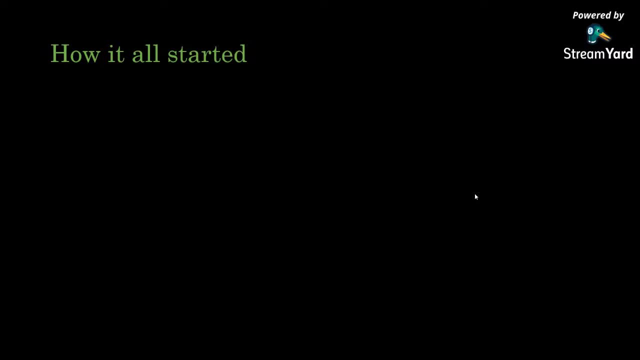 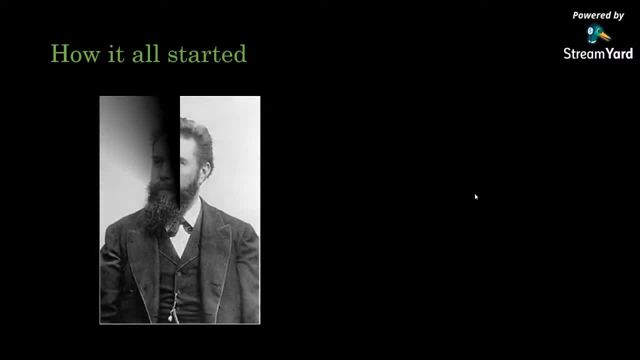 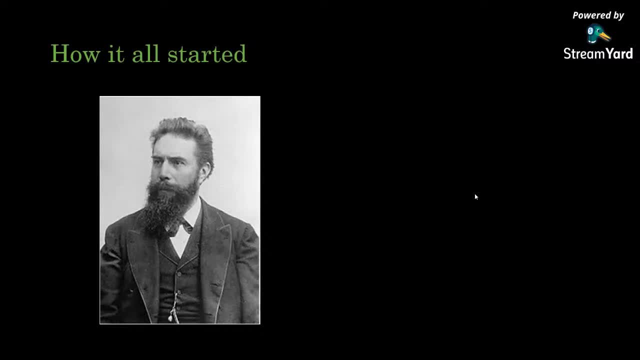 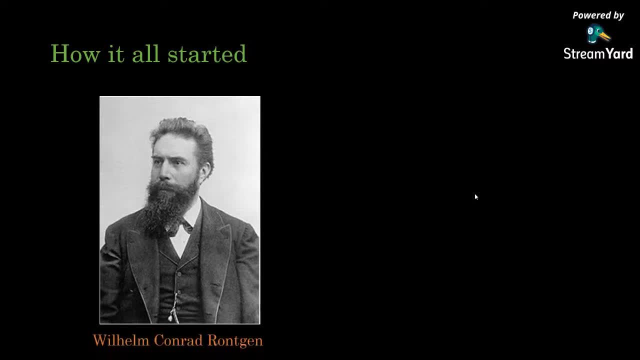 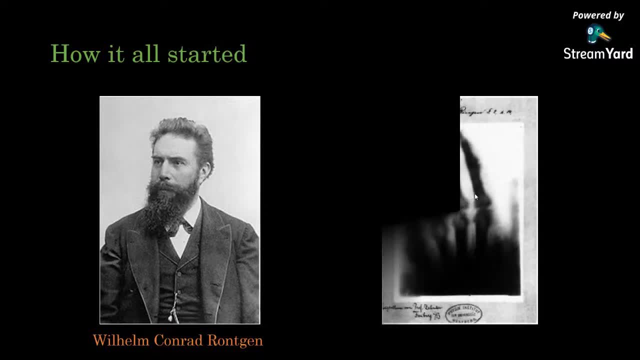 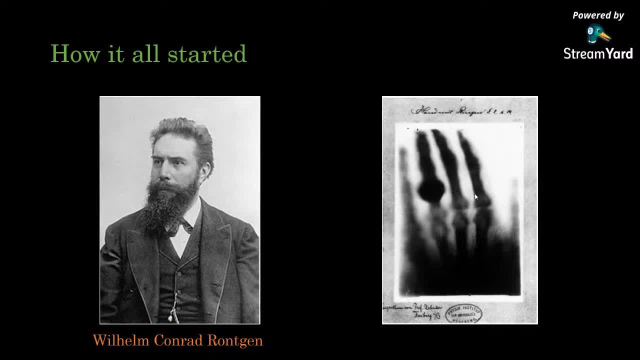 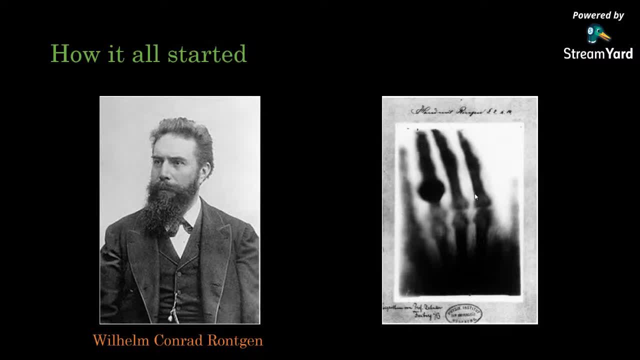 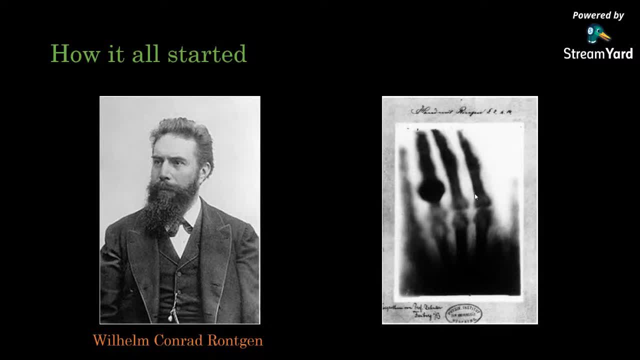 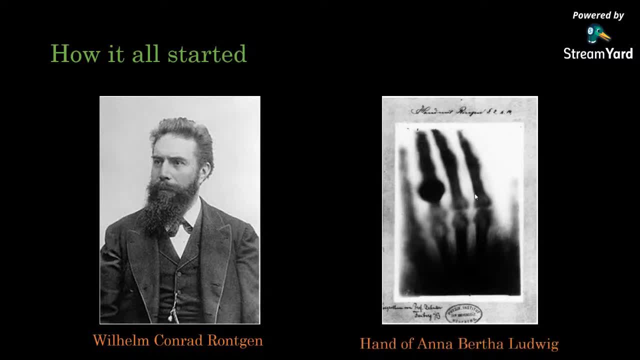 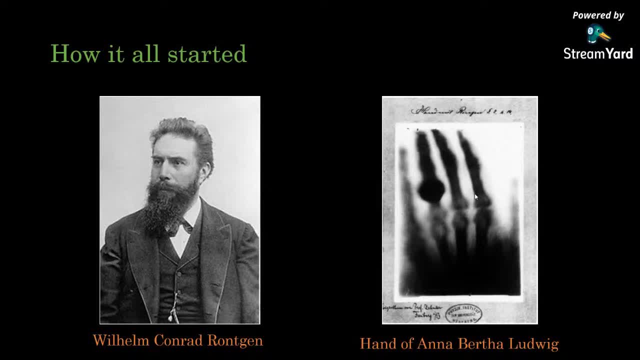 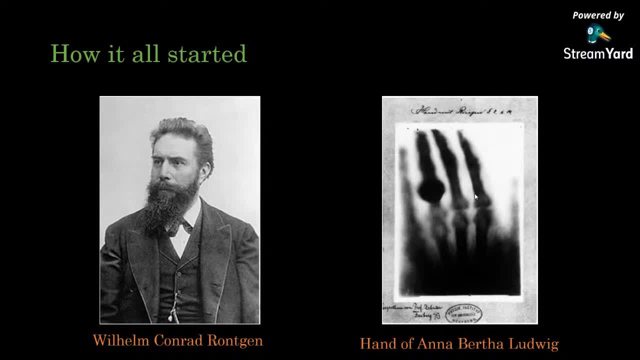 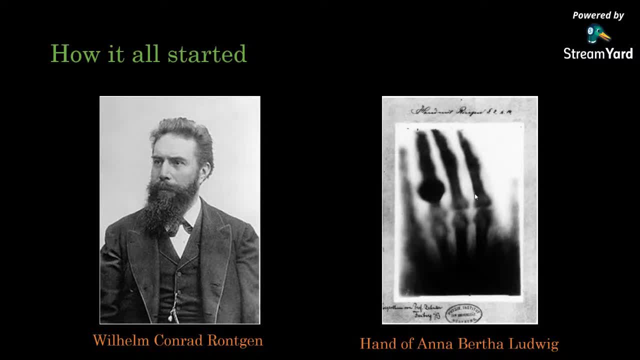 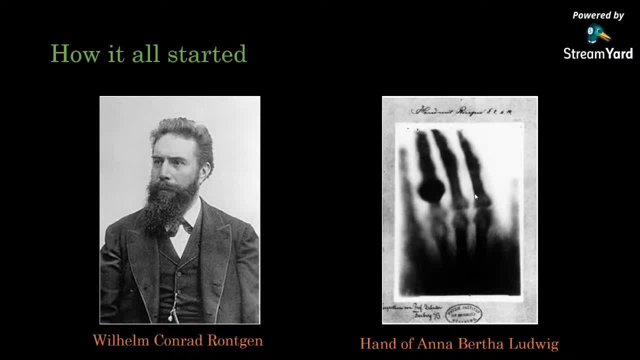 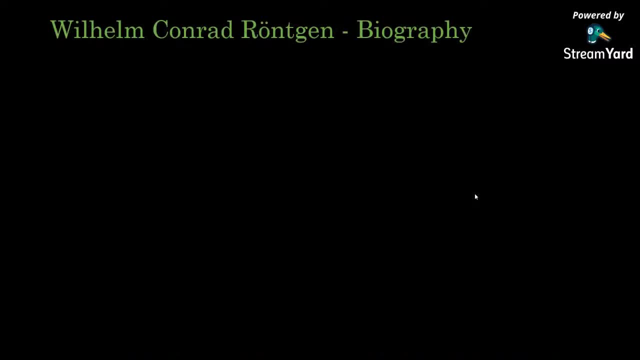 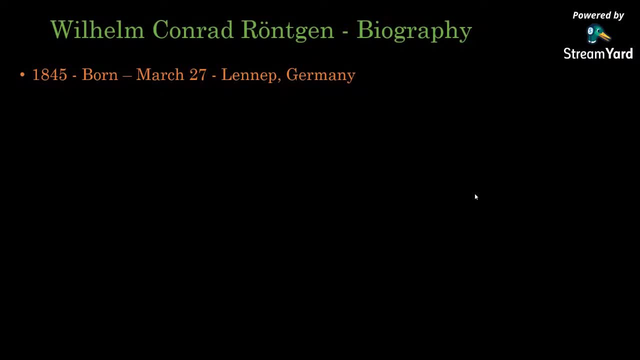 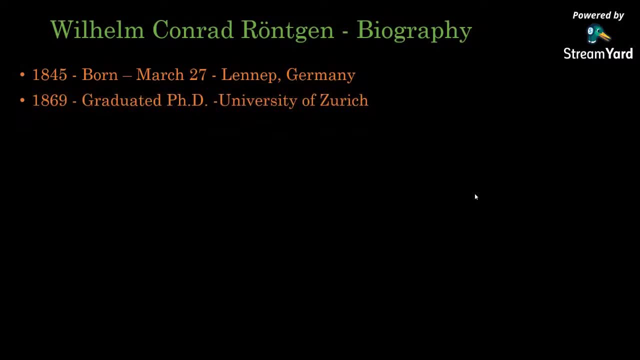 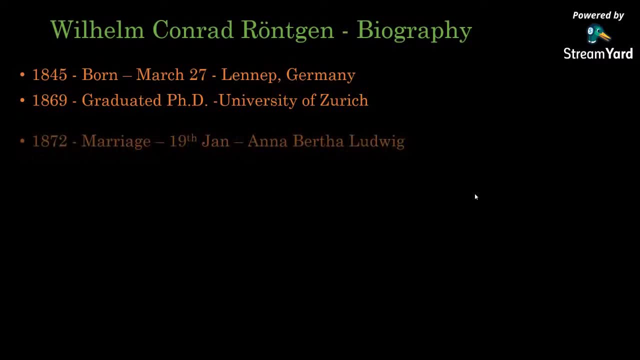 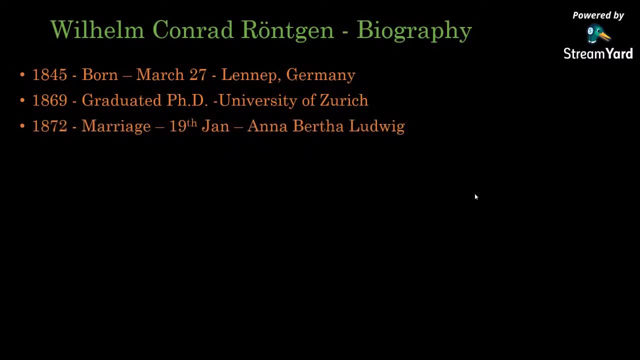 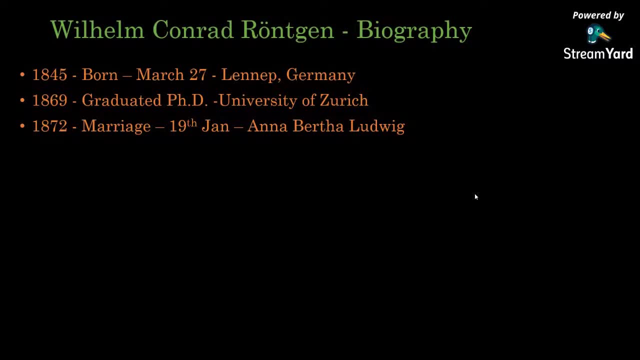 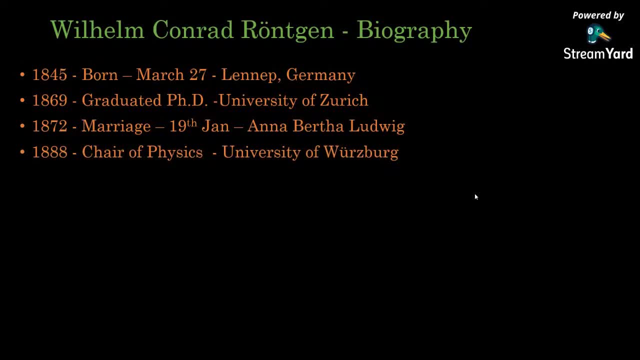 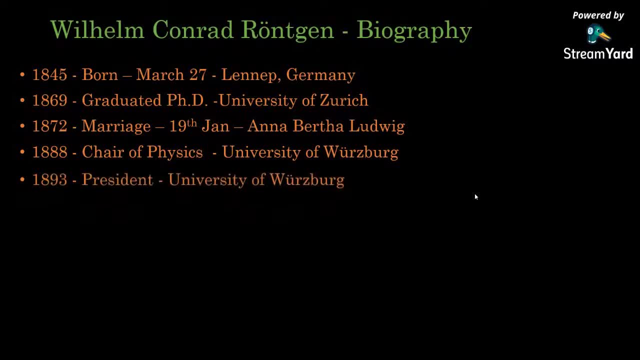 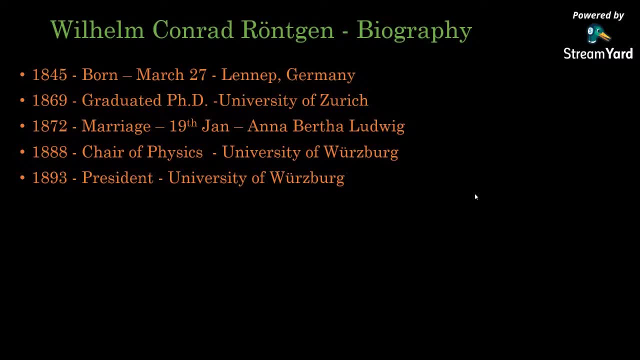 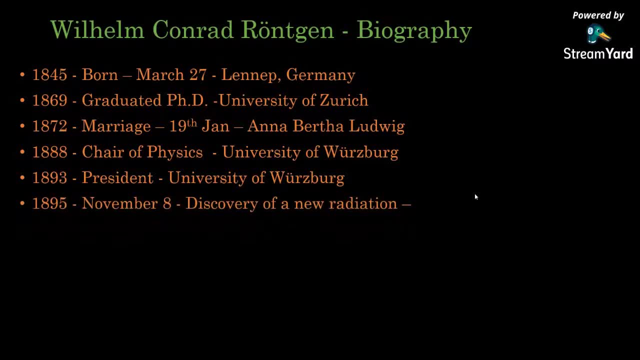 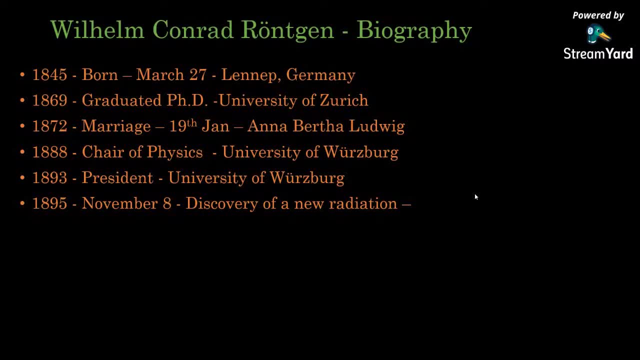 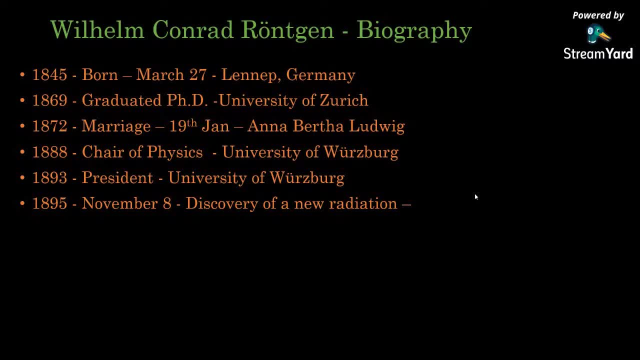 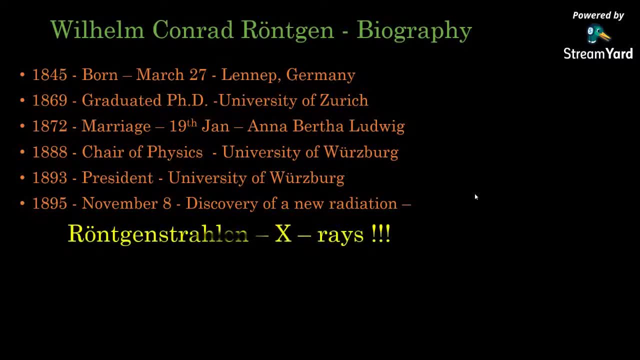 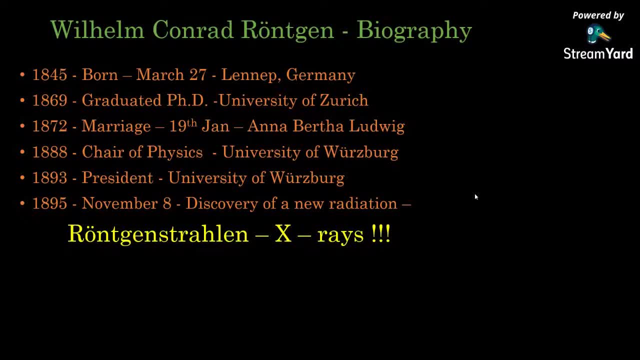 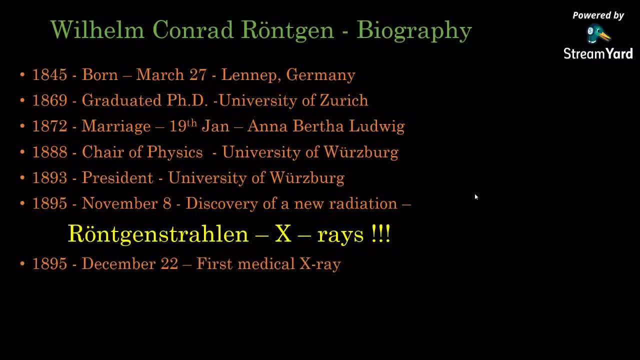 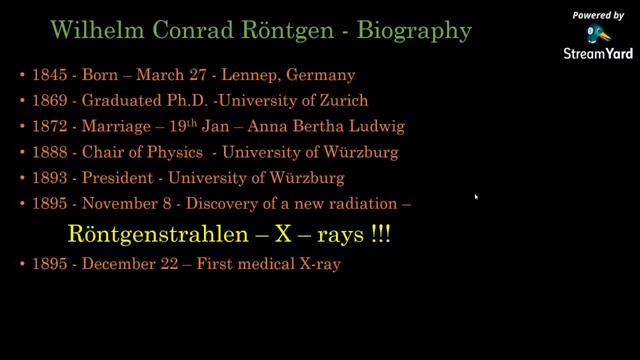 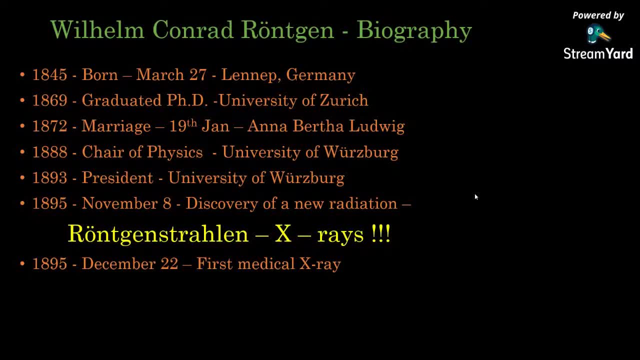 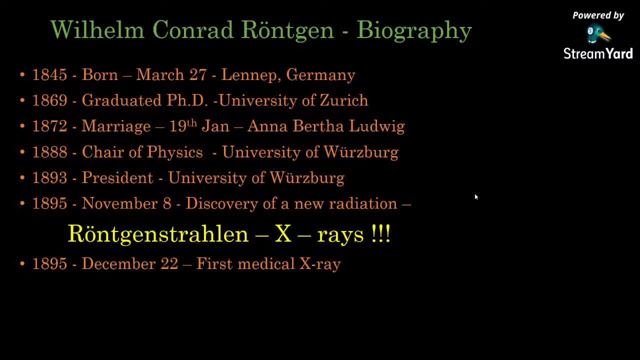 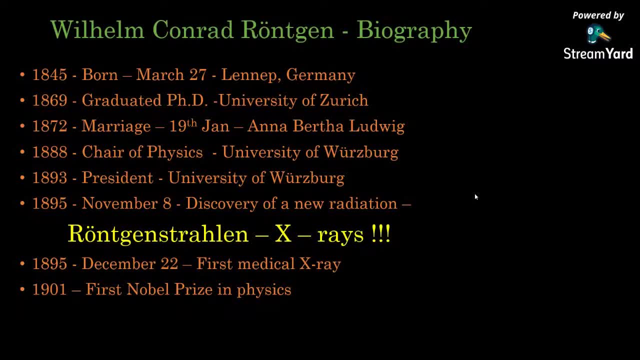 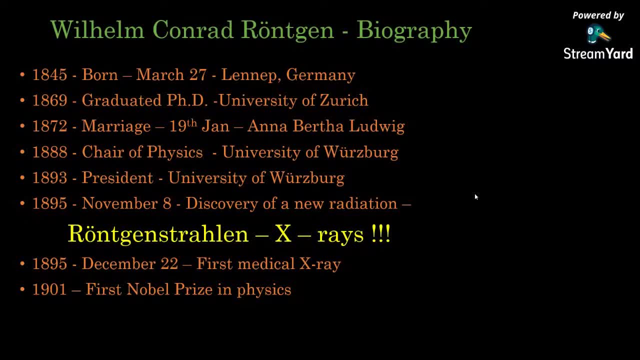 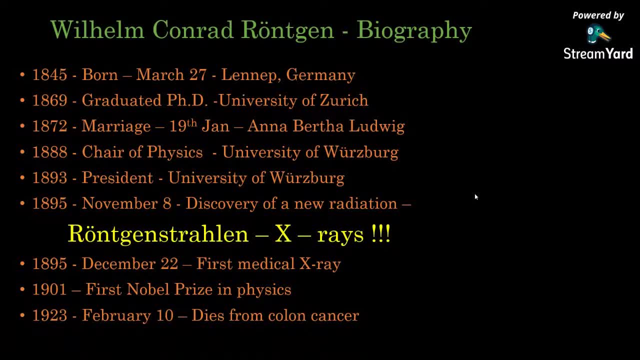 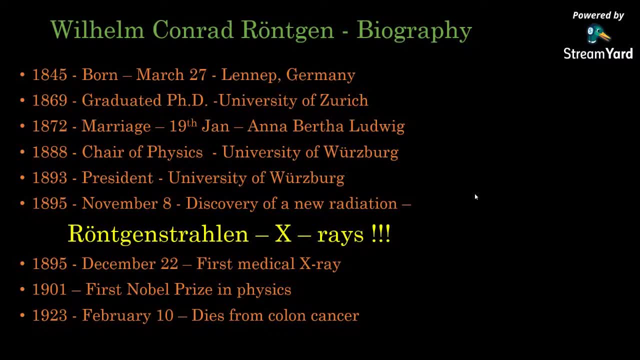 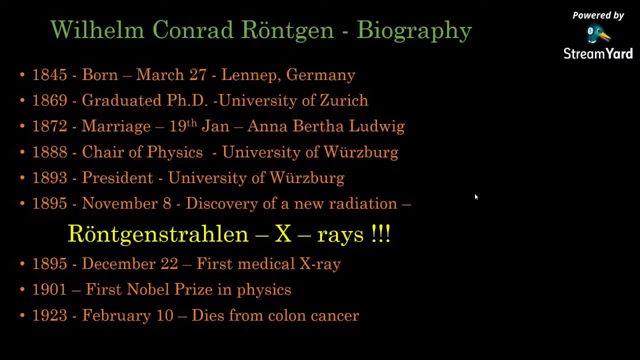 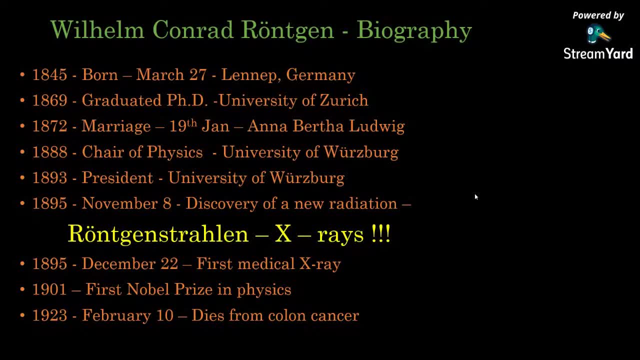 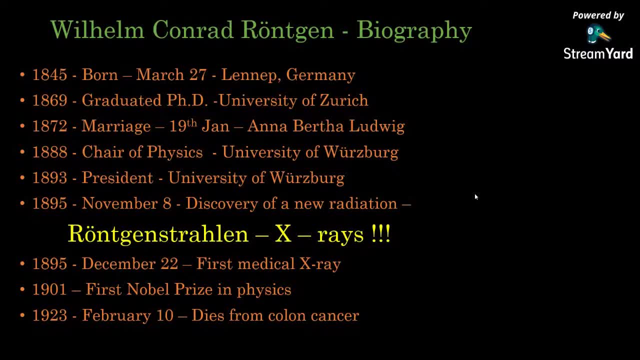 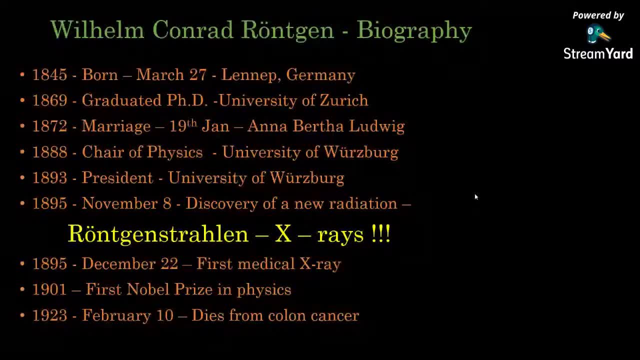 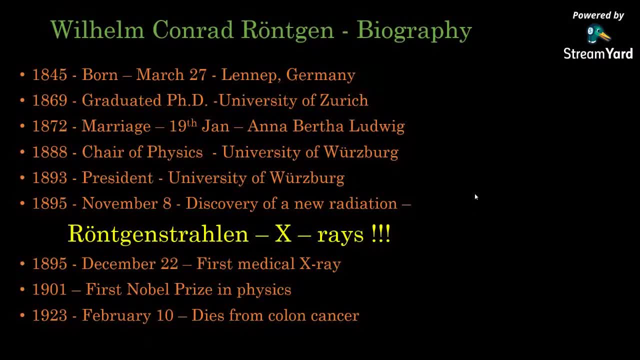 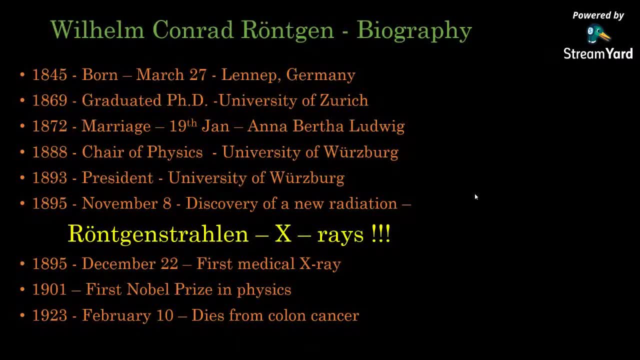 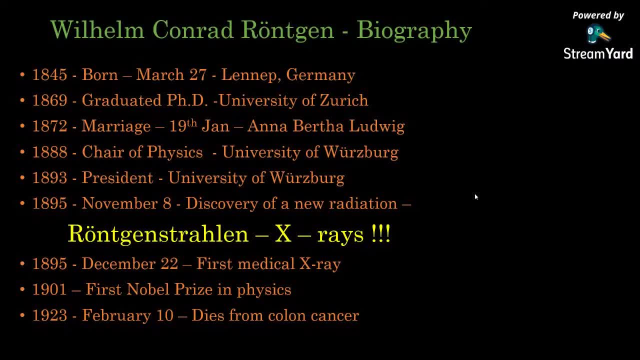 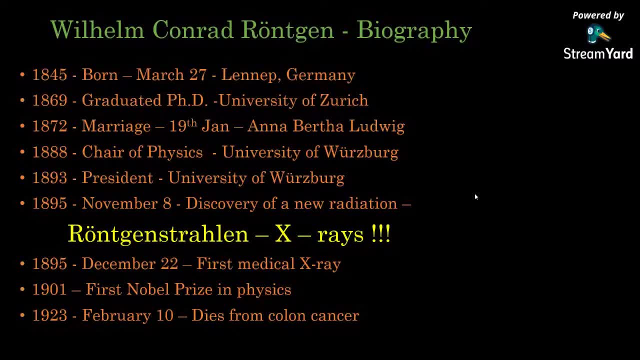 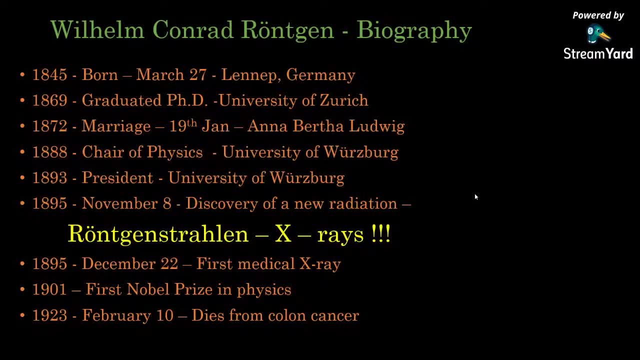 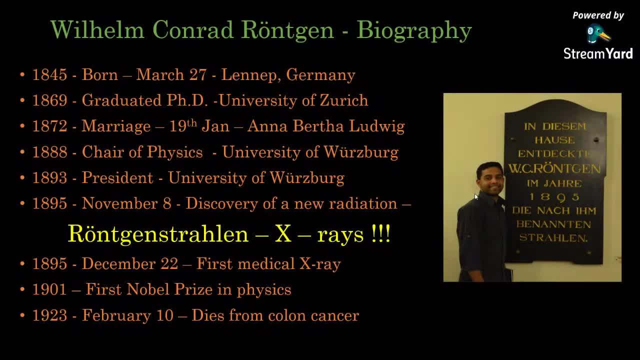 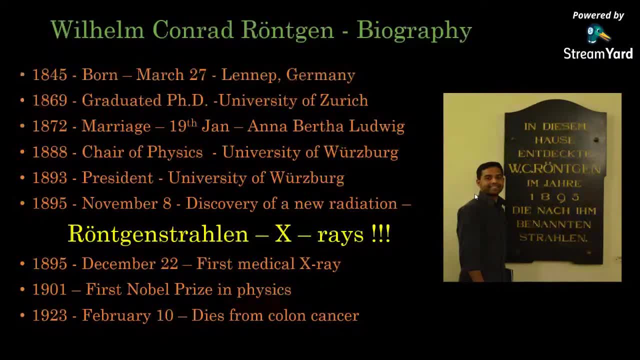 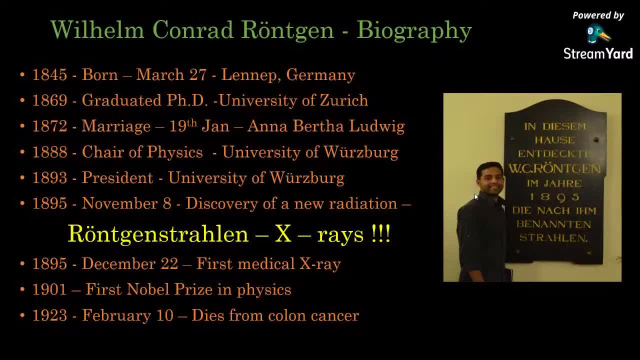 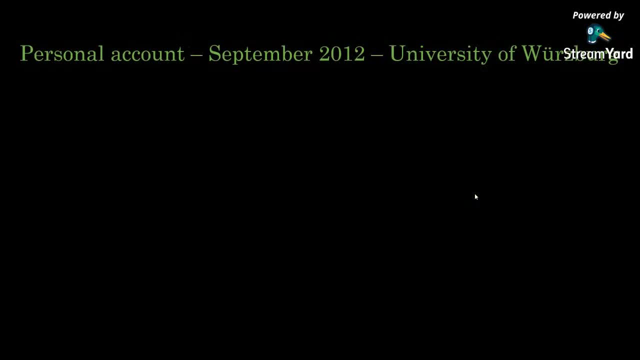 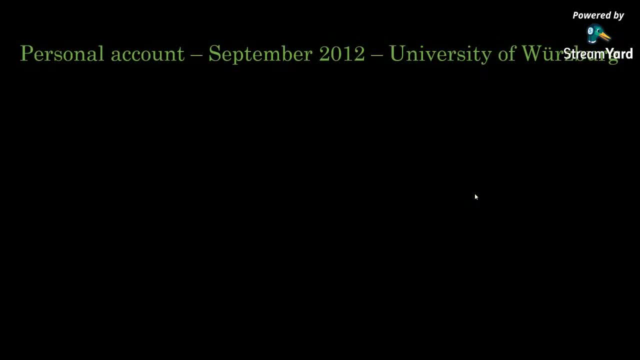 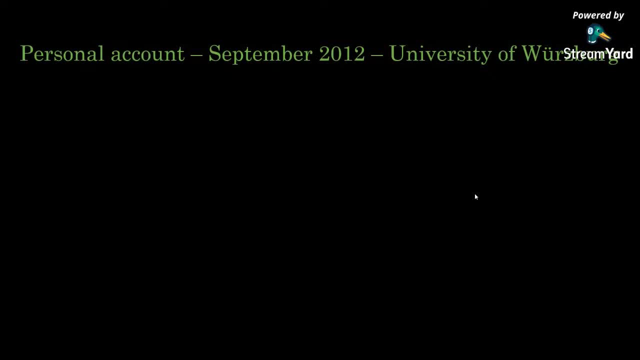 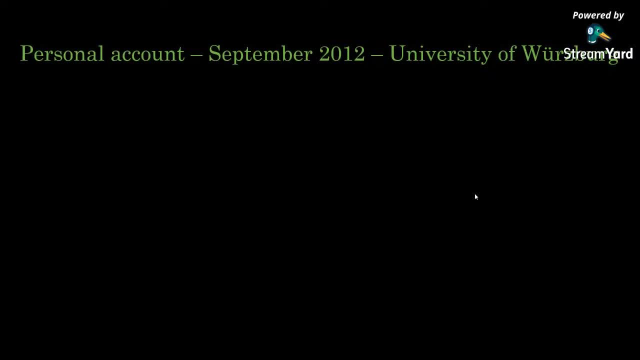 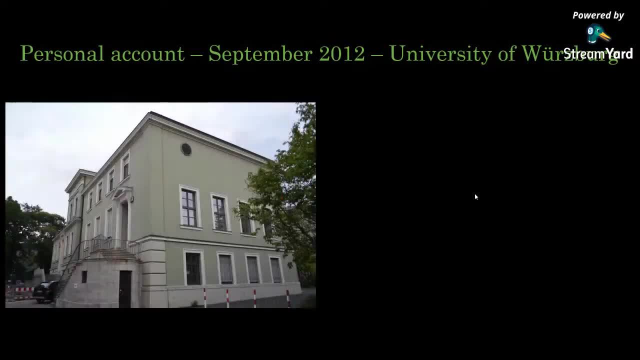 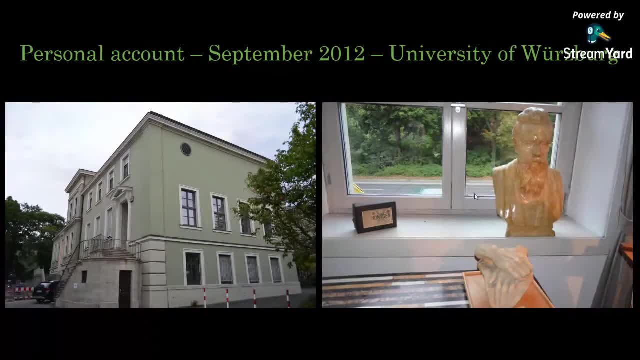 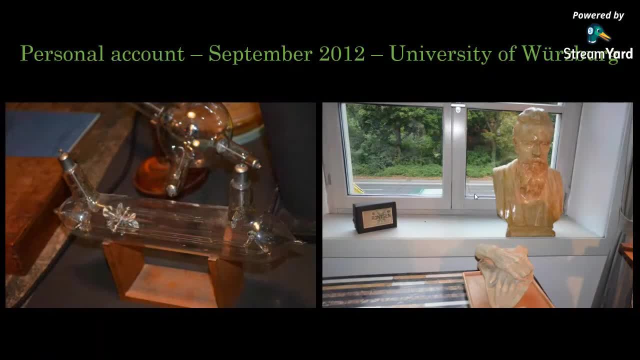 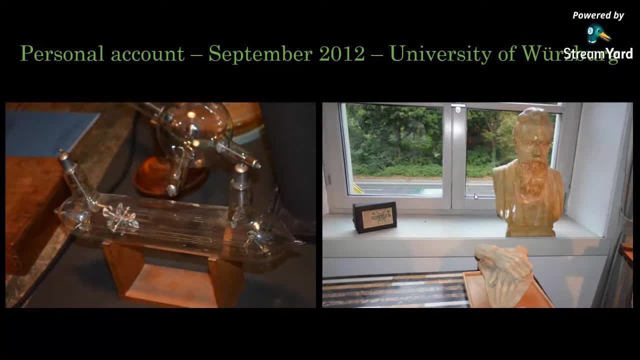 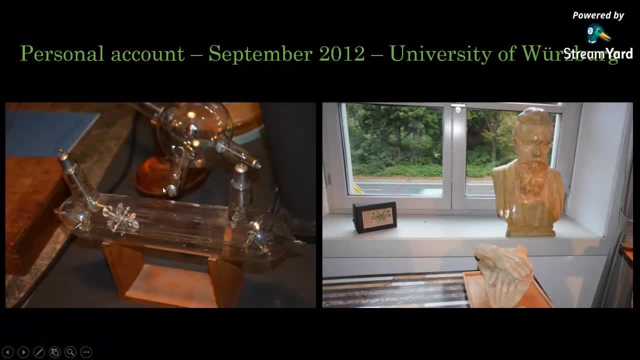 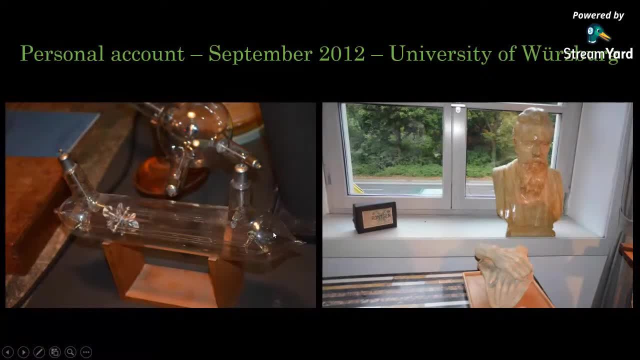 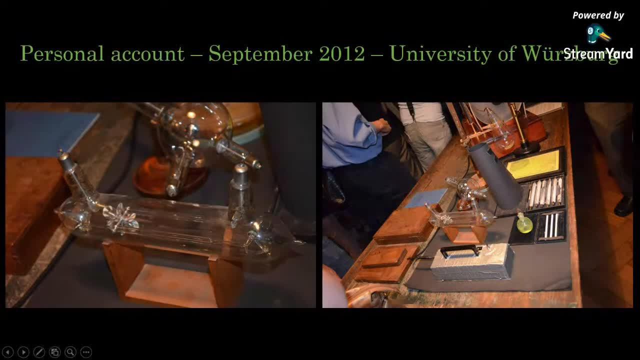 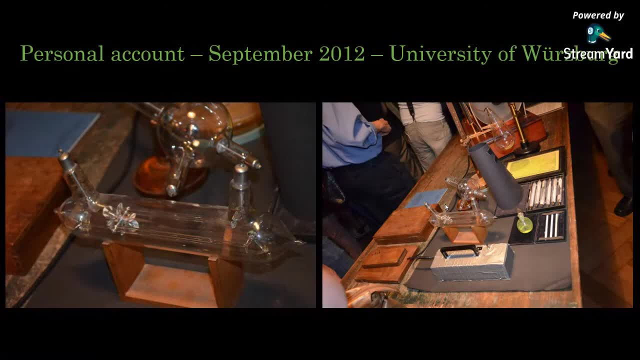 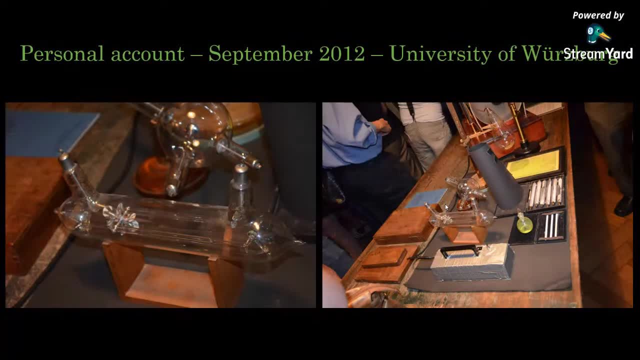 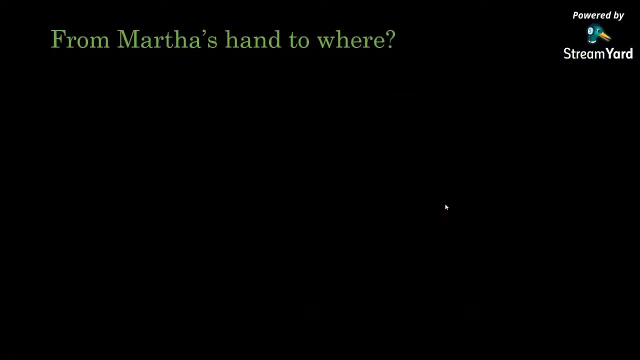 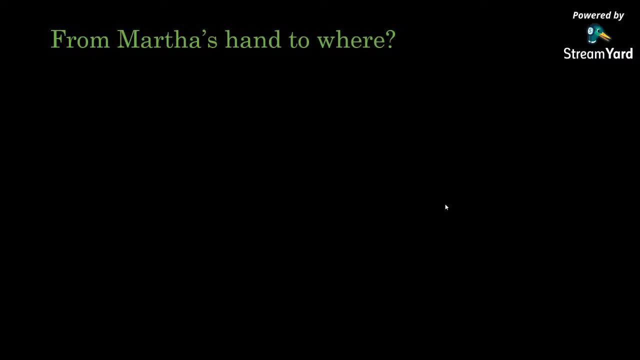 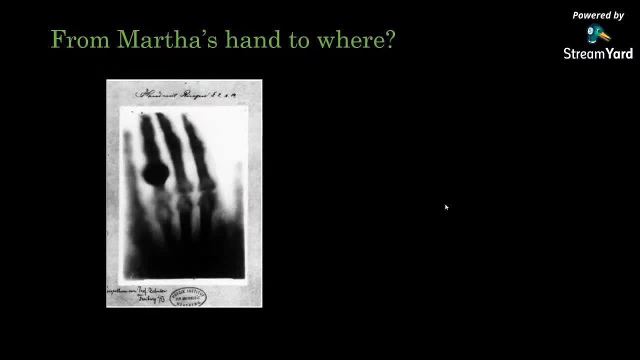 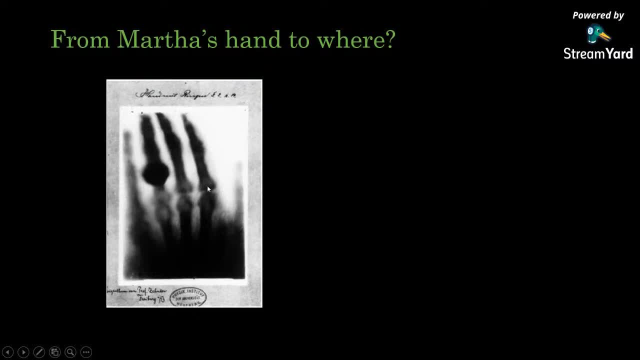 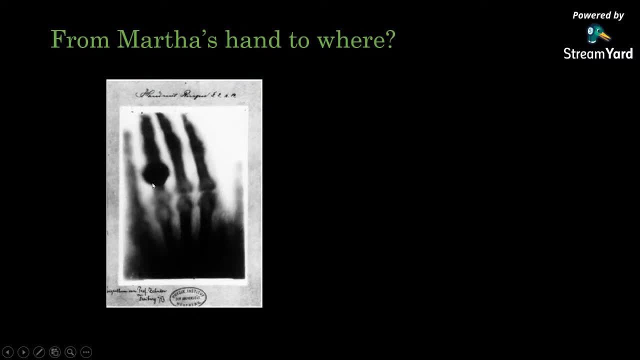 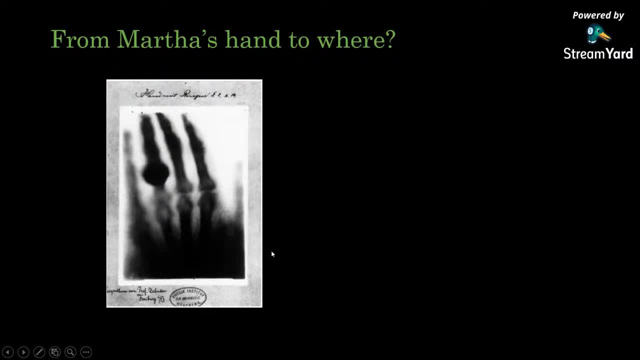 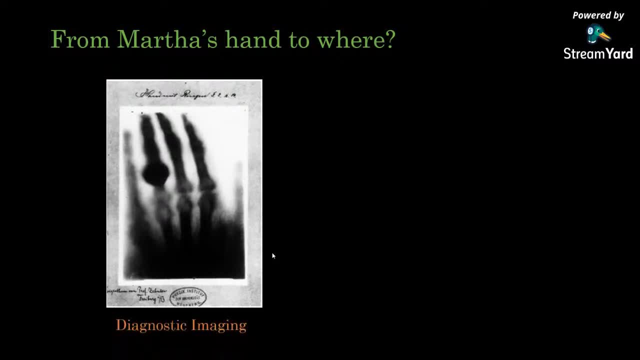 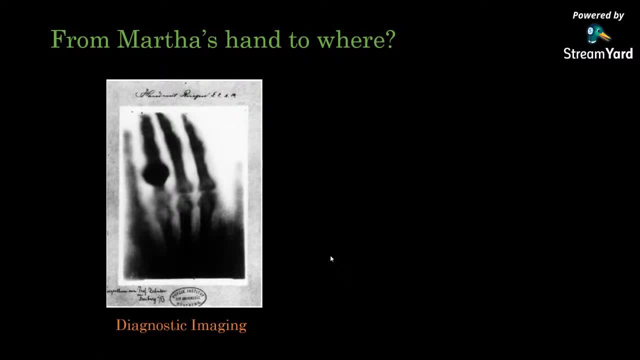 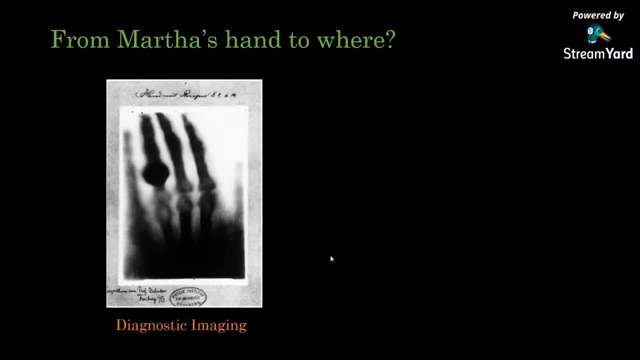 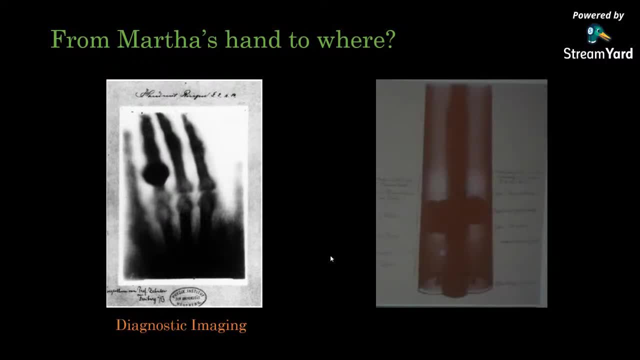 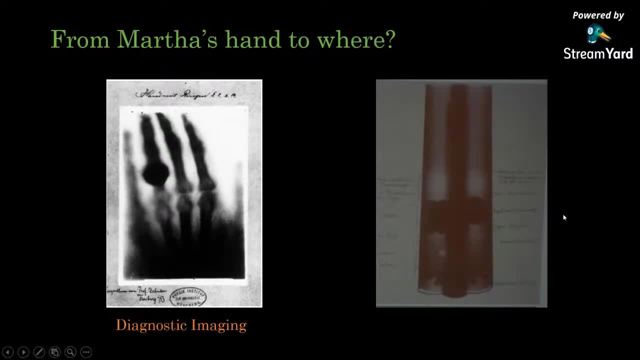 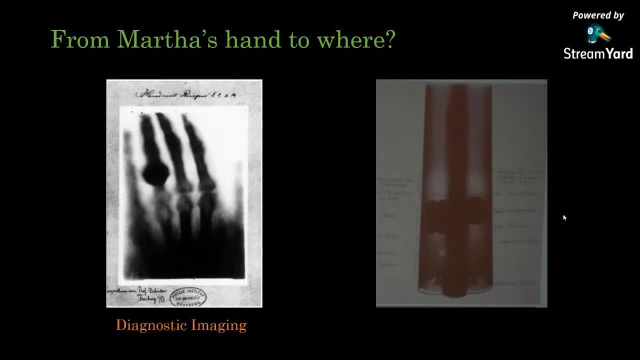 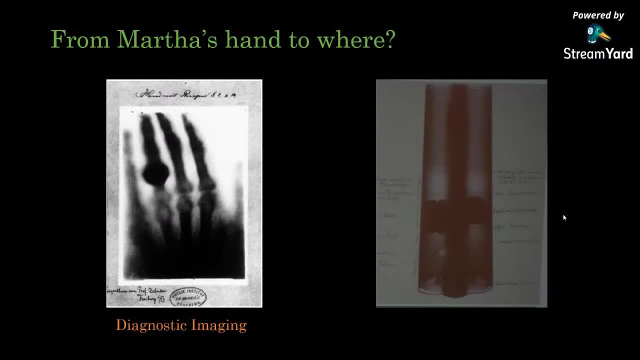 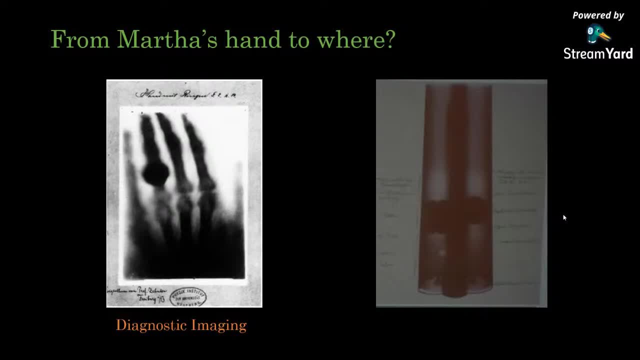 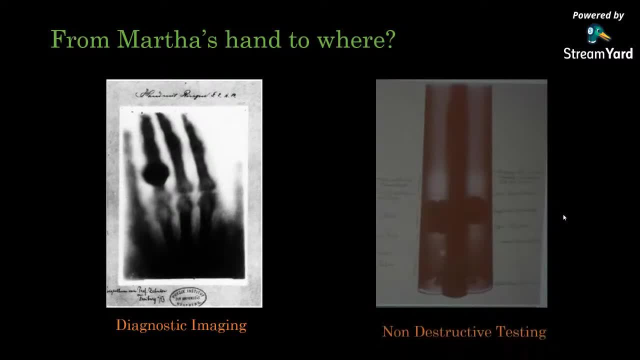 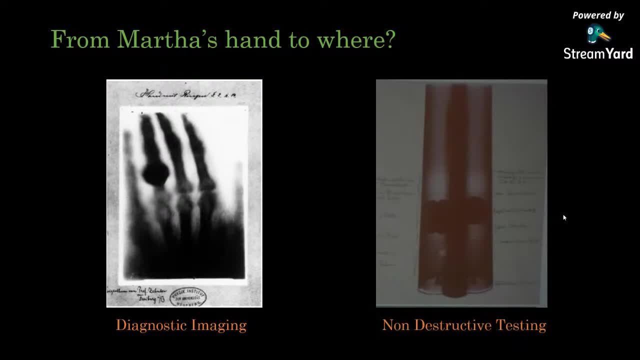 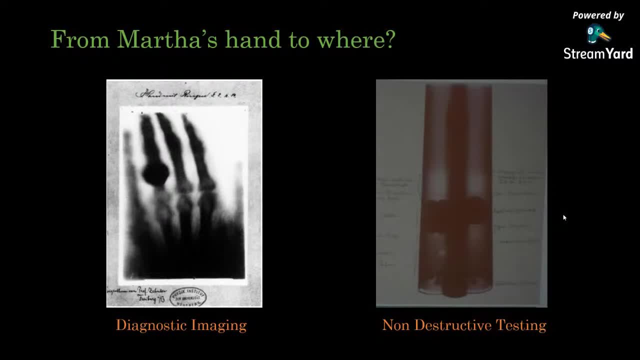 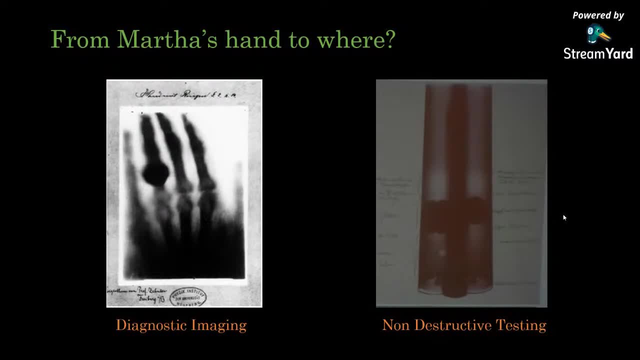 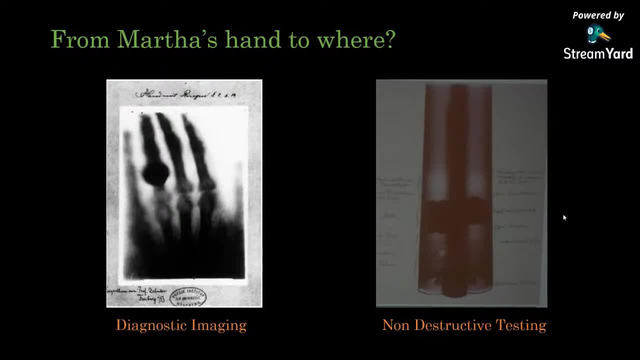 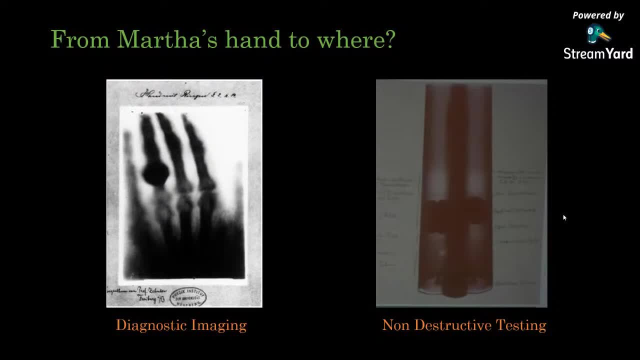 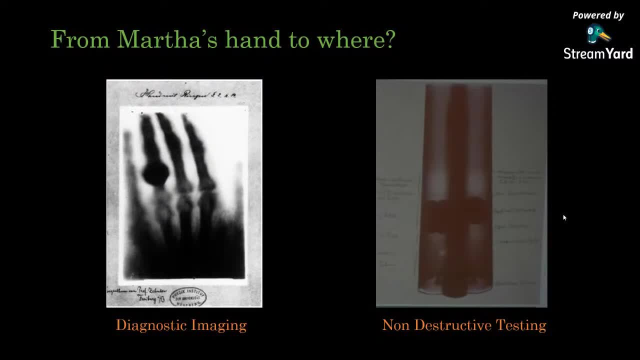 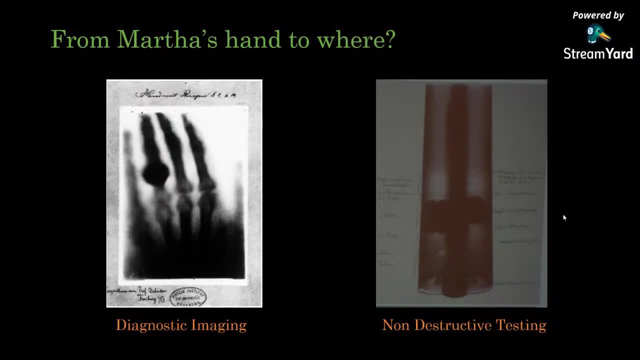 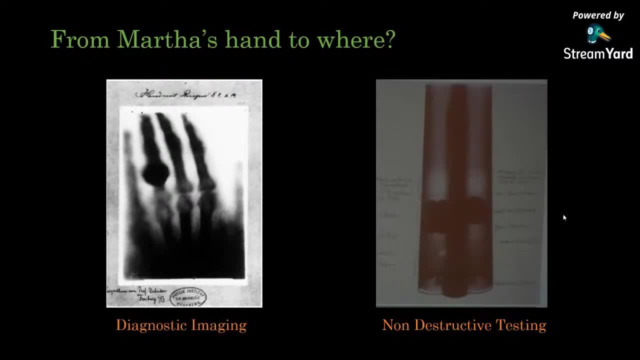 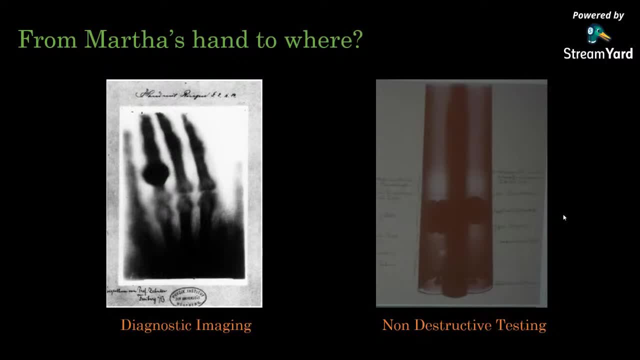 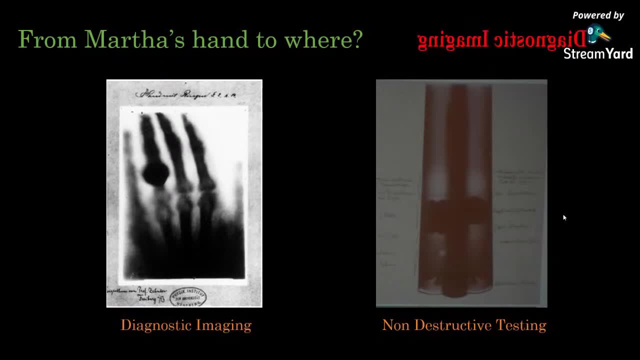 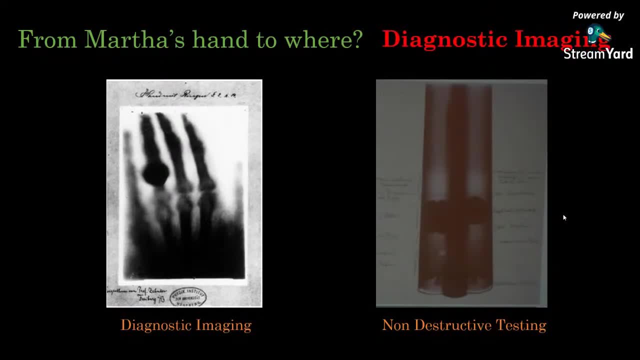 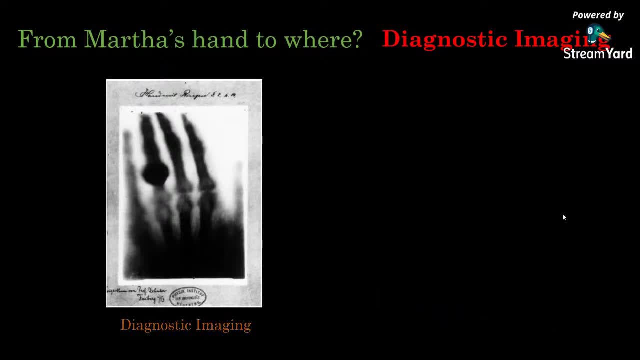 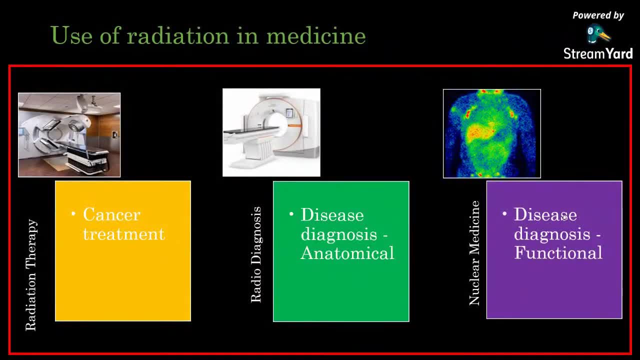 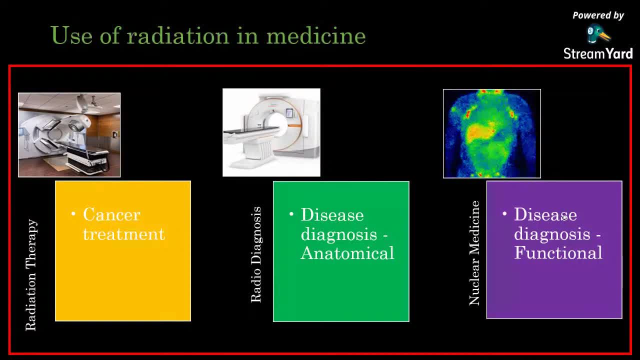 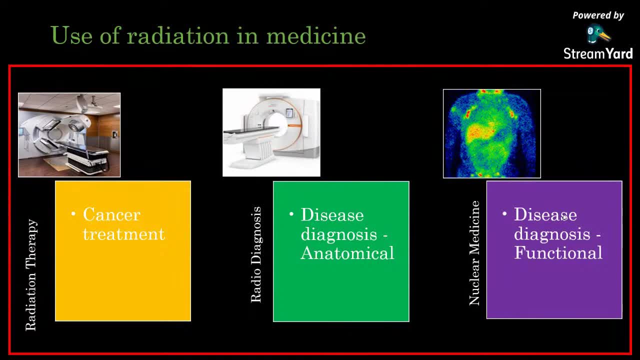 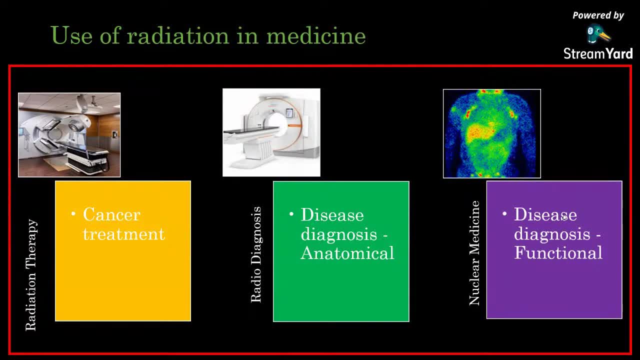 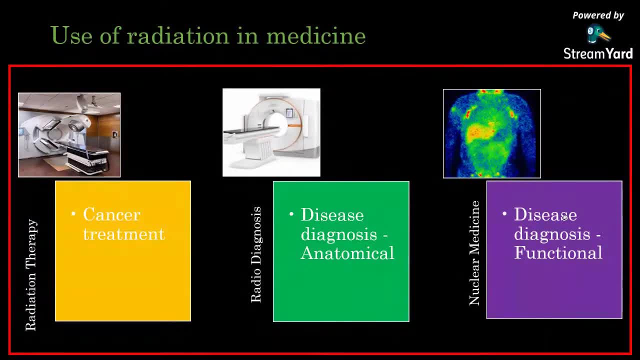 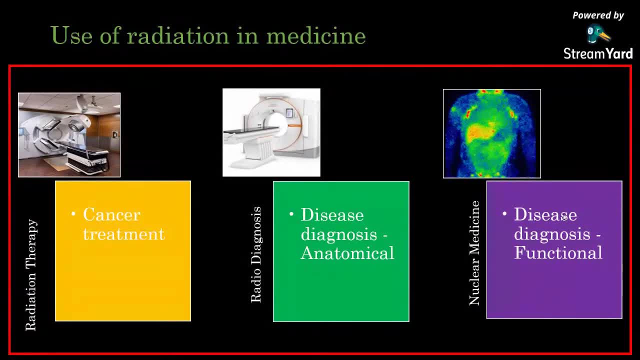 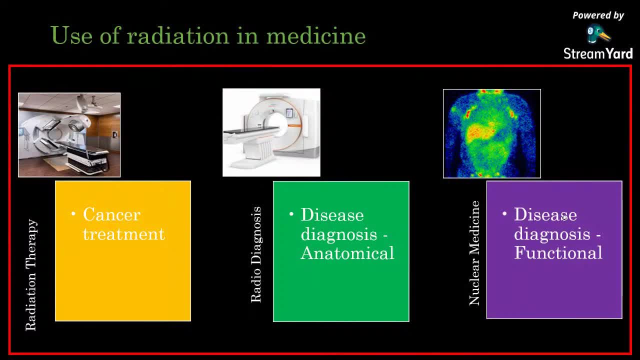 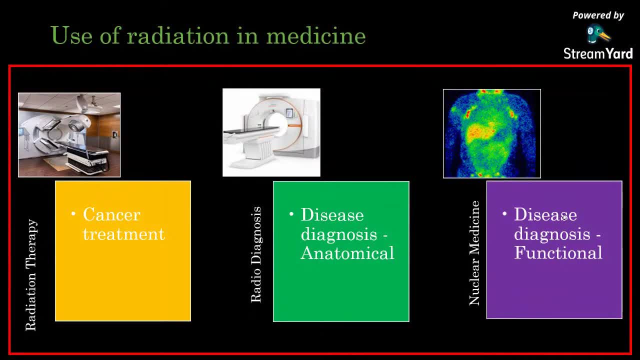 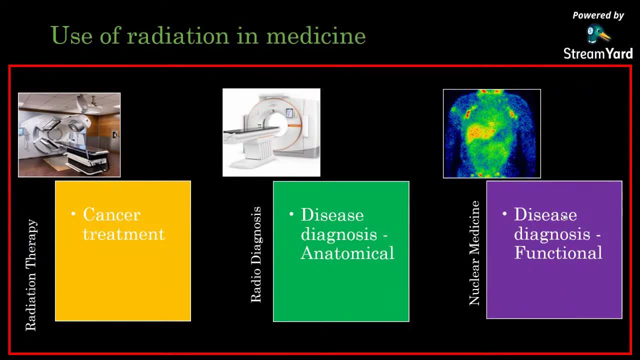 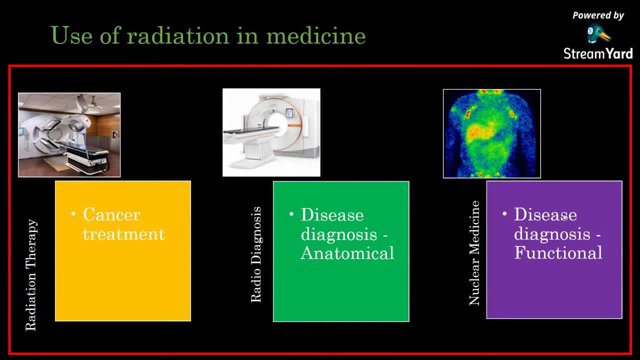 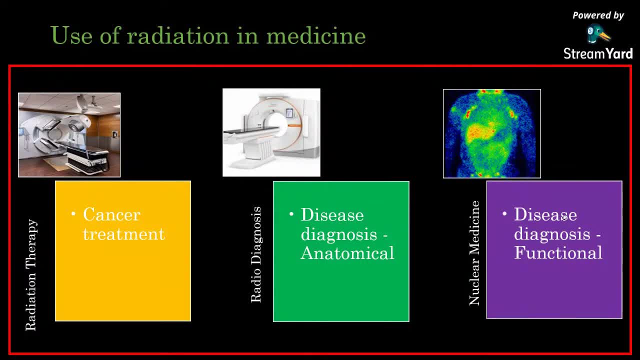 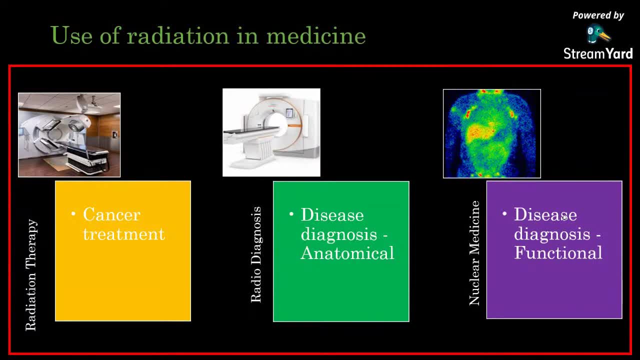 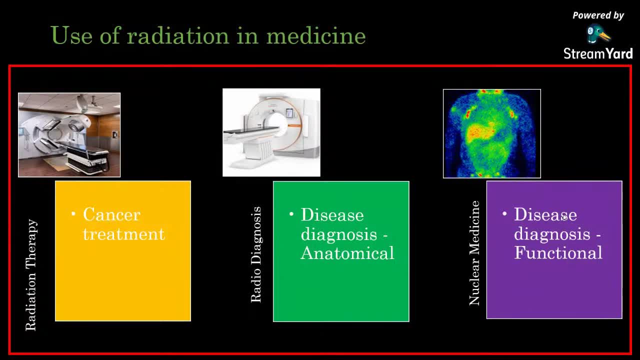 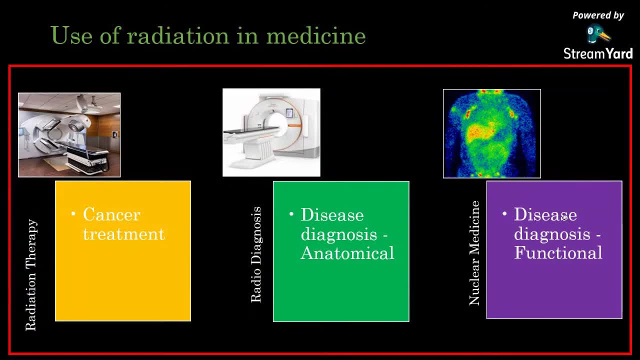 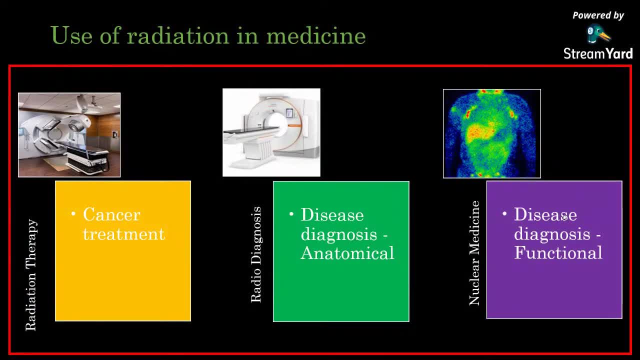 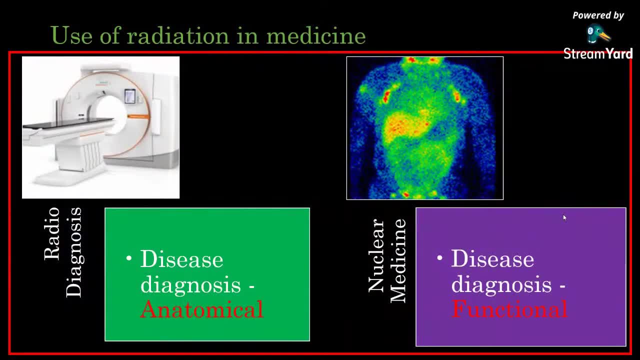 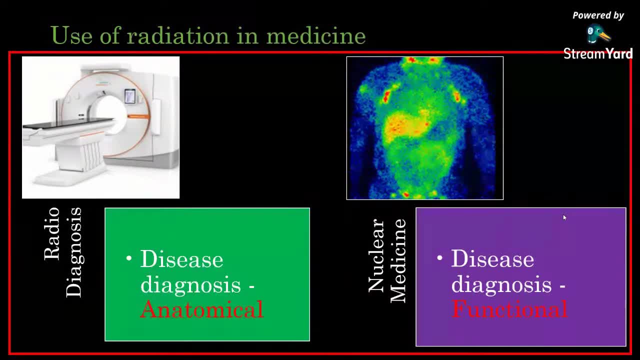 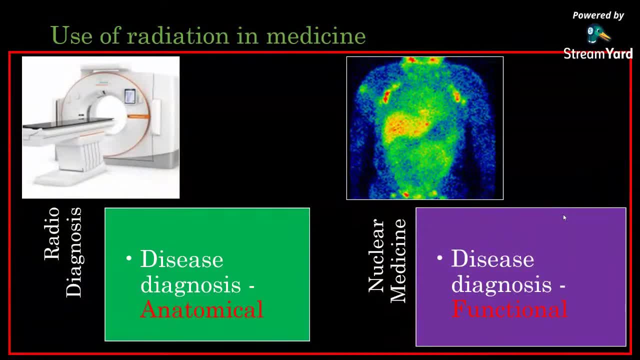 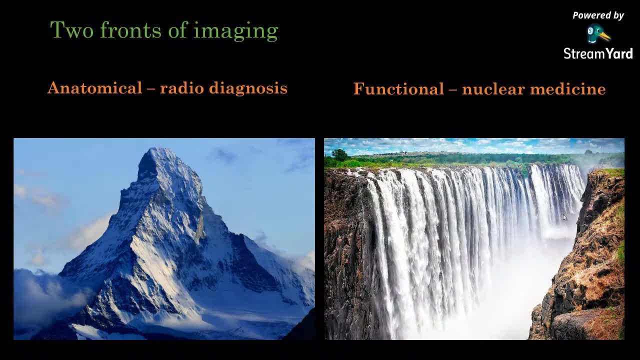 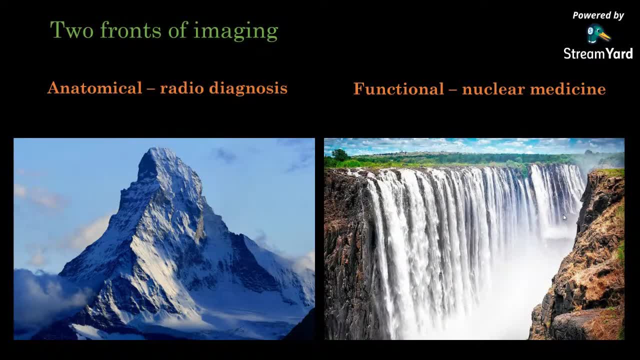 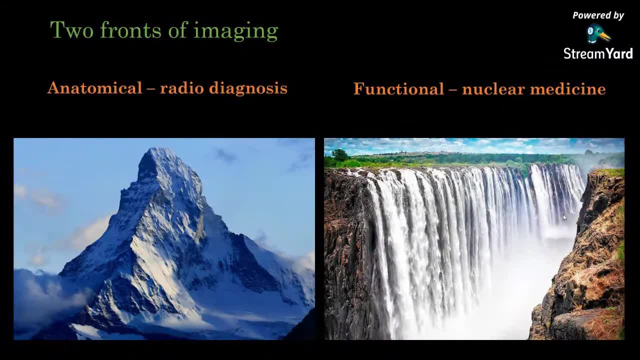 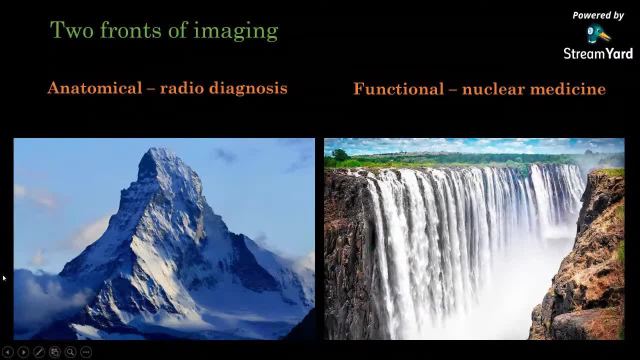 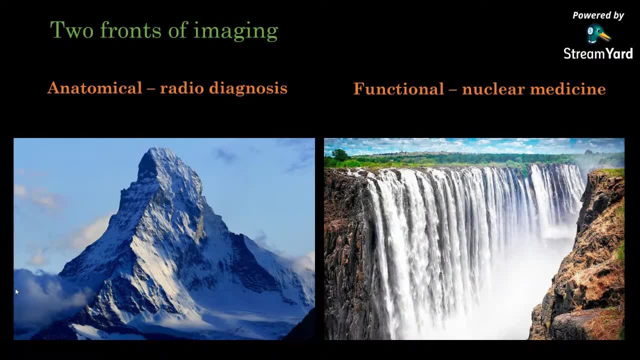 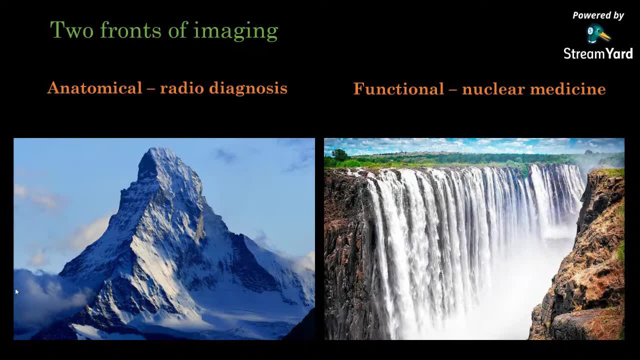 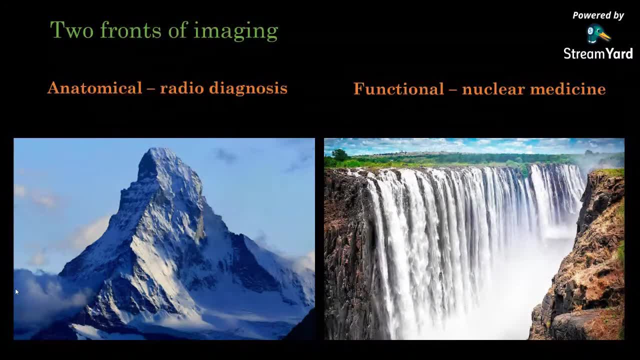 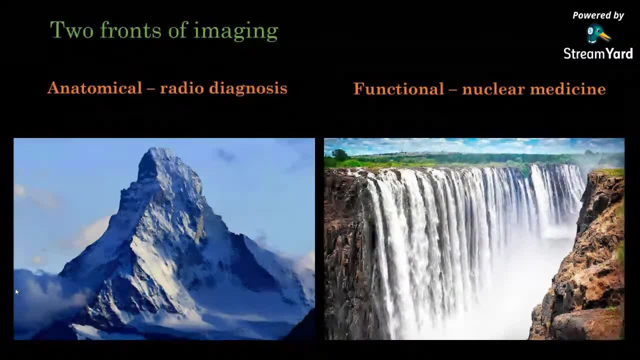 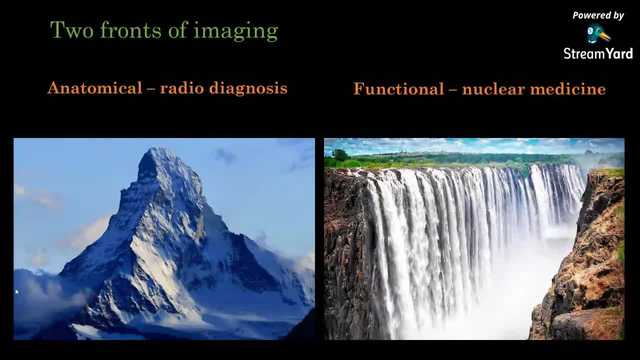 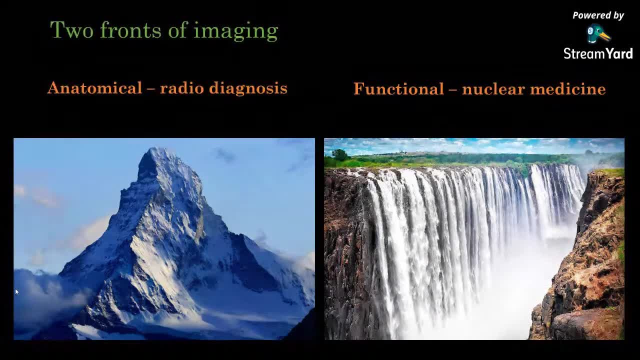 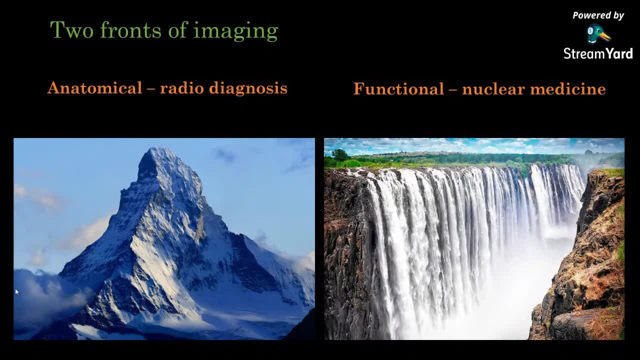 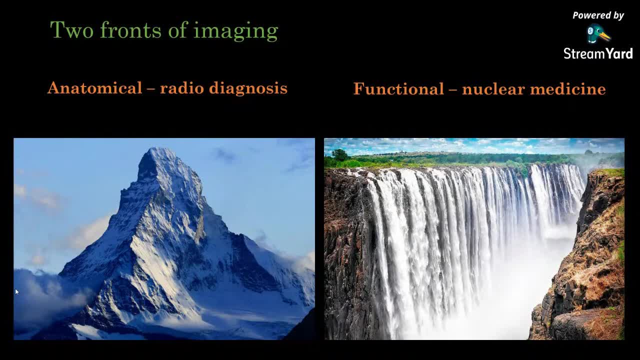 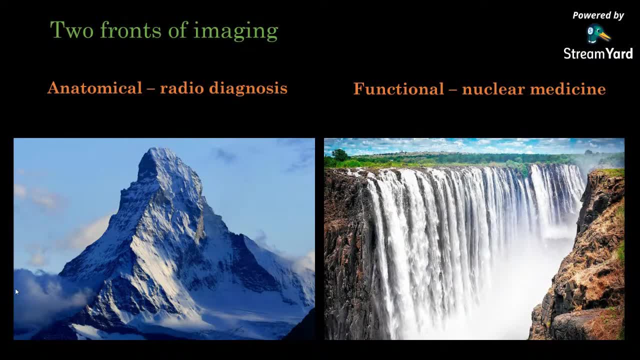 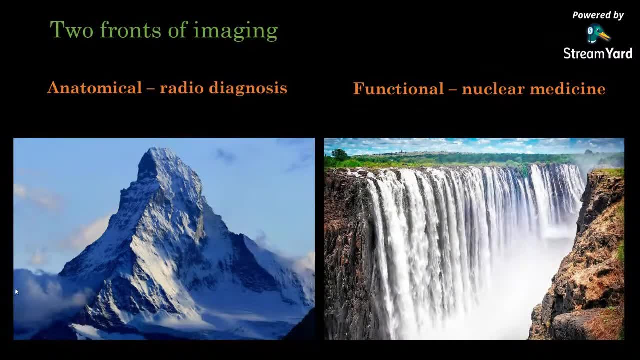 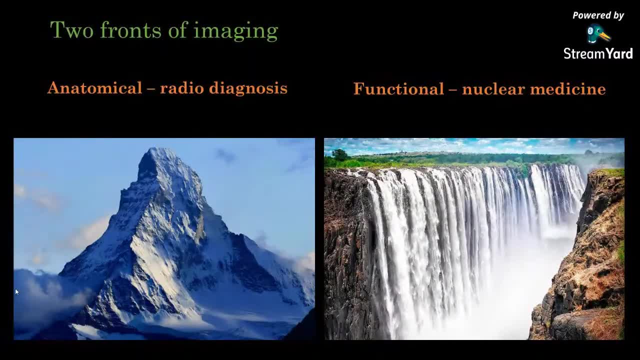 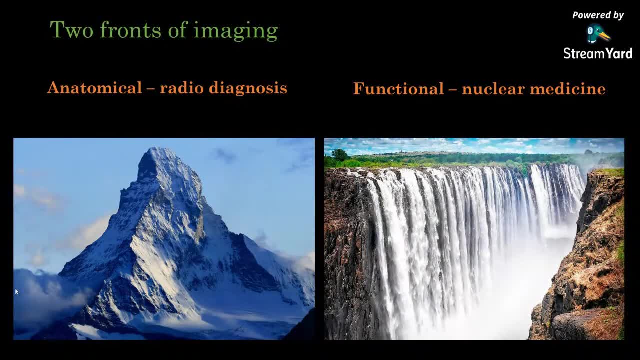 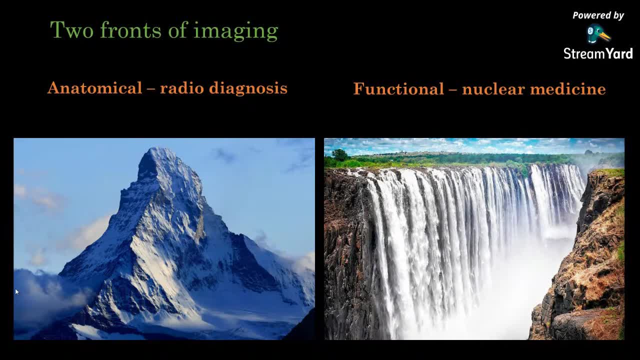 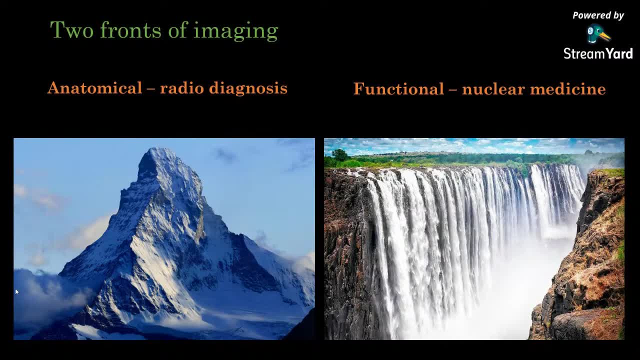 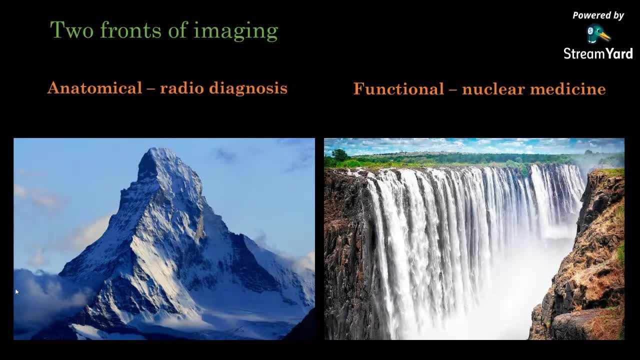 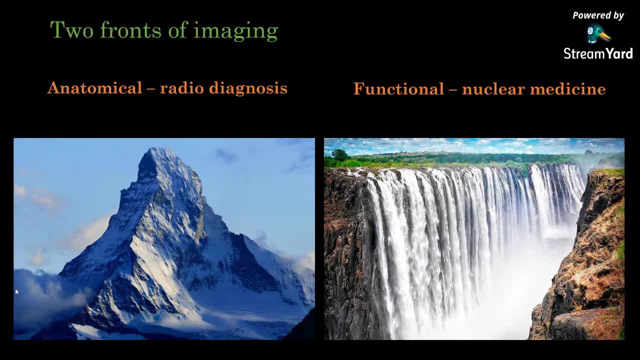 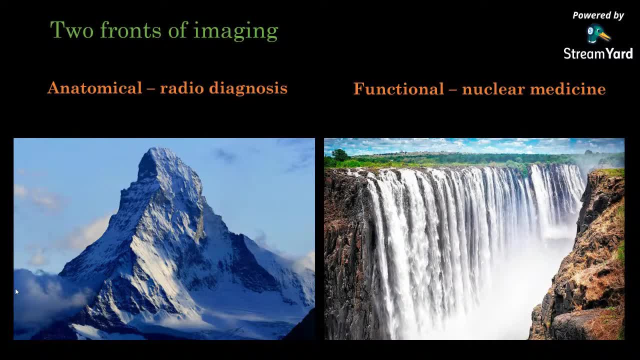 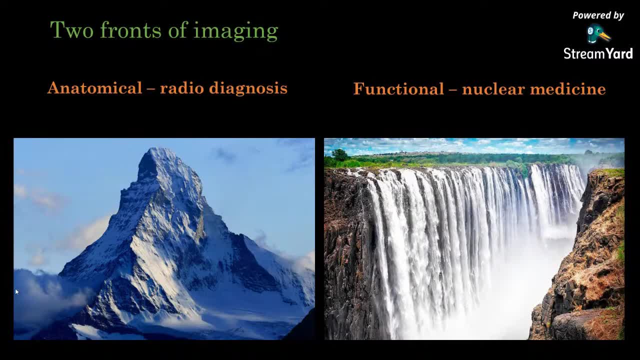 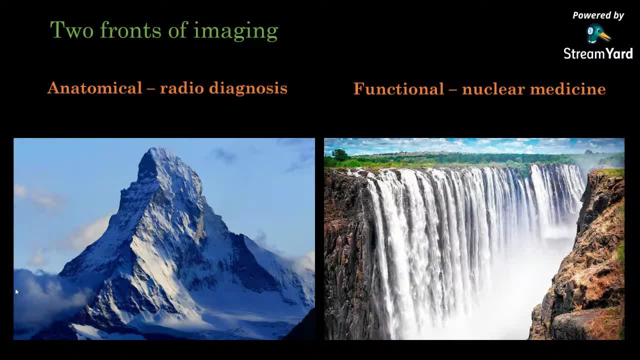 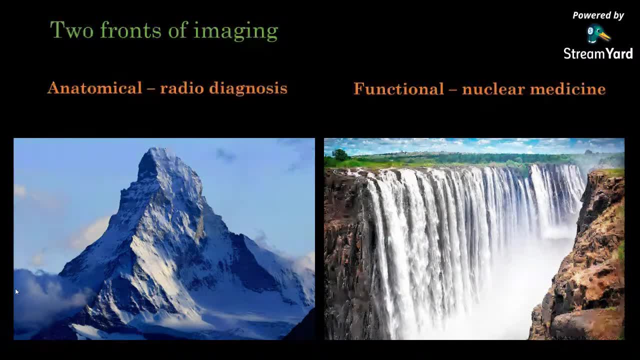 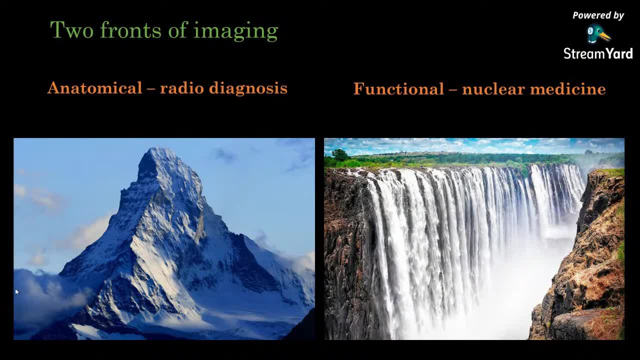 Radiation can be considered as the trigger for the development of radiation. Radiation can be considered as the trigger for the development of radiation. Radiation can be considered as the trigger for the development of radiation studies. you will find that different parts of the liver actually works differently and you will be 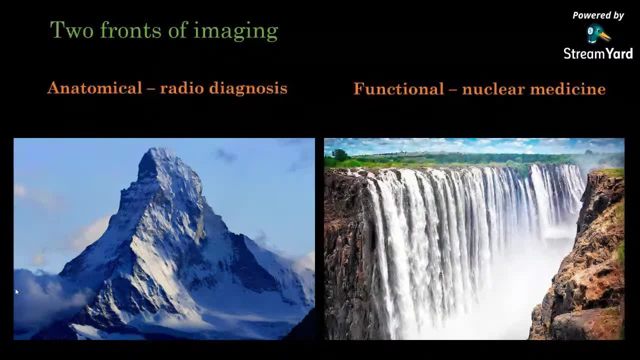 able to get a functional idea about, or a physiological idea about, the organ itself. So they both have their own roles to play in radio diagnosis or in diagnostic imaging, but one is more focusing on the anatomy of the organ, whereas the other one is focusing more on the physiology. 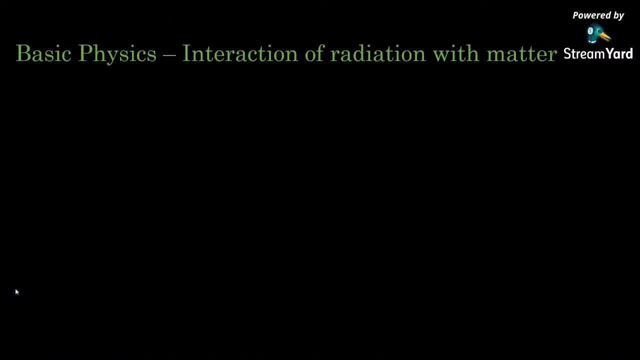 of the organ. So the basic physics of radio diagnosis is the interaction of radiation with matter. As I said, the focus today is purely on photons and when photons interact with matter, physics students and some of the basic science students would know that the three predominant 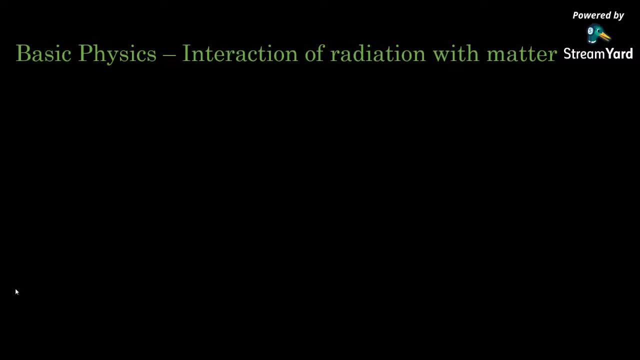 phenomena that happen are photoelectric effect, Compton effect and pair production, And we know that at relatively lower energy ranges, that is, around 30 kiloelectron volt and below, the only phenomenon that exists is photoelectric effect. And above 30 keV we know that Compton effect starts to take over and then 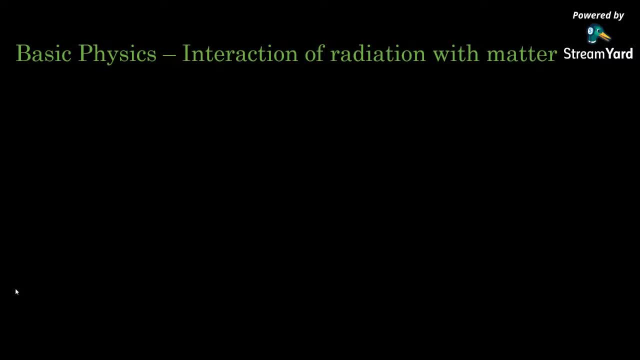 after 1.02 meV. that is a threshold for pair production to happen. when the energy range becomes 1.02 meV and higher, pair production starts to kick in and then there is a share of energy. So that is a phenomenon that exists. And when the energy range becomes 1.02 meV, we know that Compton effect starts to take over, and then, after 1.02 meV, there is a threshold for photoelectric effect And Compton effect starts to kick in. and then, after 1.02 meV, there is a share of. 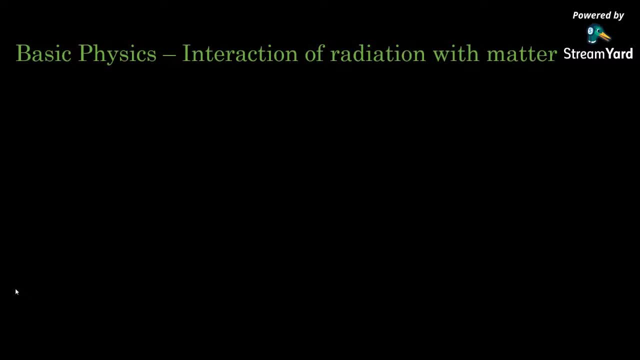 photoelectric effect and Compton effect and pair production. that can happen based on the statistical nature of the interaction, So based on the energy of the incoming spectrum and the property of the material through which the radiation passes. these three phenomenon can happen And it is a statistical phenomenon based on the cross-section of the material. 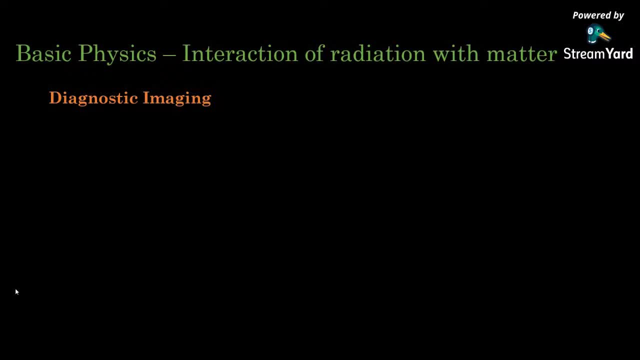 Diagnostic imaging relies more on photoelectric effect and Compton effect, And you can see that there is a starking difference between the two, which is diagnostic imaging and radiation therapy. If you were to draw a comparison, you know that diagnostic imaging is used for diagnosis, whereas radiation therapy is for treatment. 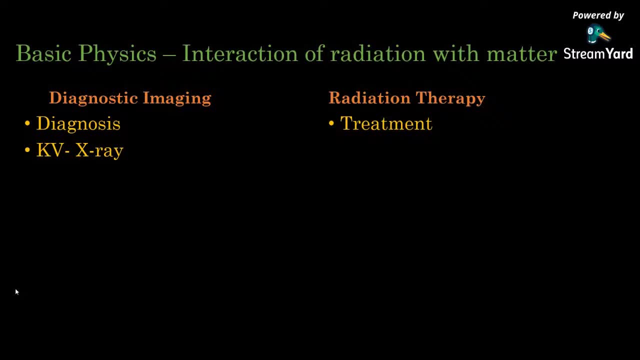 Diagnostic imaging uses kilovoltage X-ray. If it is an X-ray-based imaging, it uses kilovoltage X-ray, whereas radiation therapy uses megavoltage X-ray, which is around the range of 60-20 MeV, whereas diagnostic imaging uses around 60-120 KeV, which is the kilovoltage range. 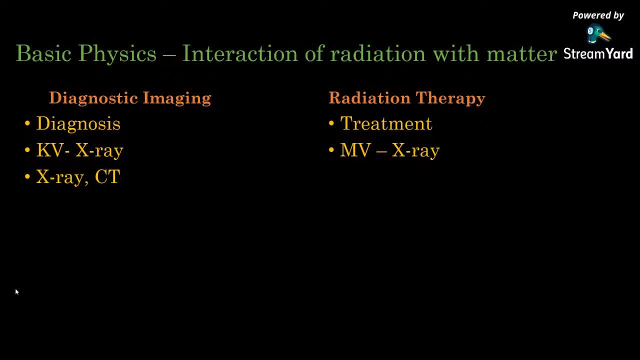 And some of the very common techniques used are X-ray machines, CT scanners- I'm sure you would have heard of all these terminologies In your day-to-day life- whereas in radiation therapy, the state-of-the-art device used and the most common technique used is using a device called a linear accelerator. 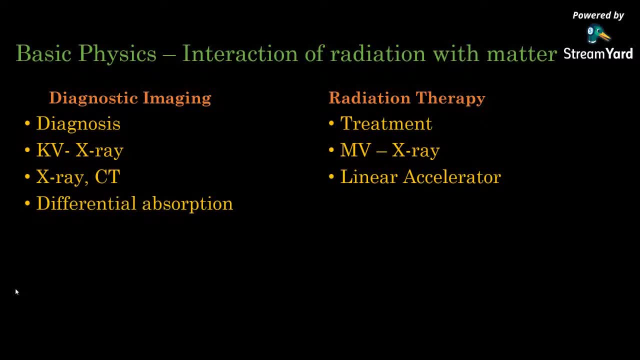 And the basic physics behind diagnostic imaging is called differential absorption, which I'll come to what it is in a minute. Whereas in radiation therapy what is expected is a biological change through a deposition of of energy by the incoming radiation into the biological material, whereby the radiation- the high-energy radiation that pass through the organs, deposit the dose and ultimately results in the biological effect which is the killing of the cancer cells. 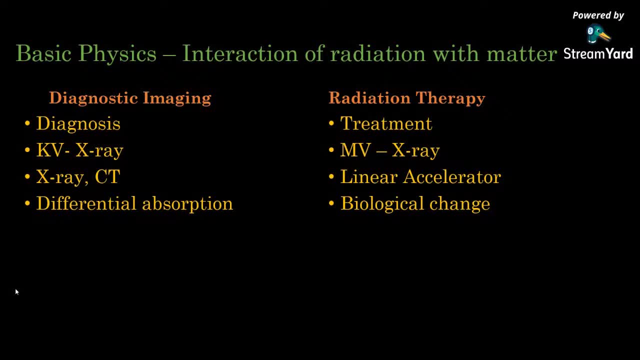 That is the aim of radiation therapy, whereas in diagnostic imaging we try and reduce the effect, biological effect. We do not want an alteration of the cells, but we rather want a differential absorption of the incoming X-ray by the organs of the body so that we get an image. 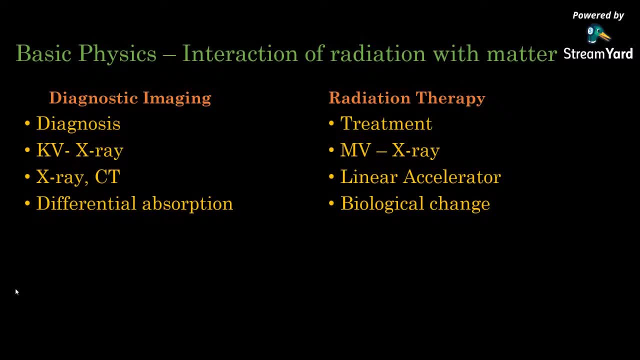 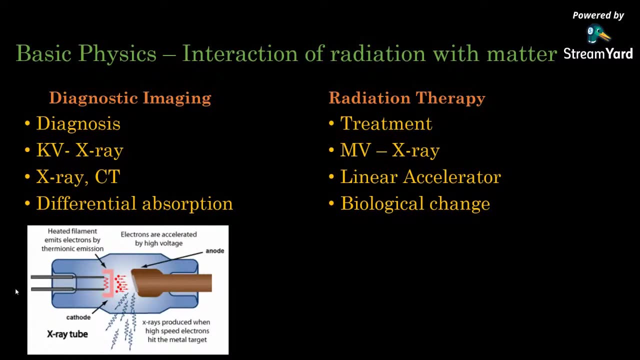 We do not expect to have a biological change within the cell, Even though that happens as a side effect. that is not the aim of the procedure, So focusing more on the diagnostic imaging side, this is an X-ray tube, a cathode ray X-ray tube. you can see. 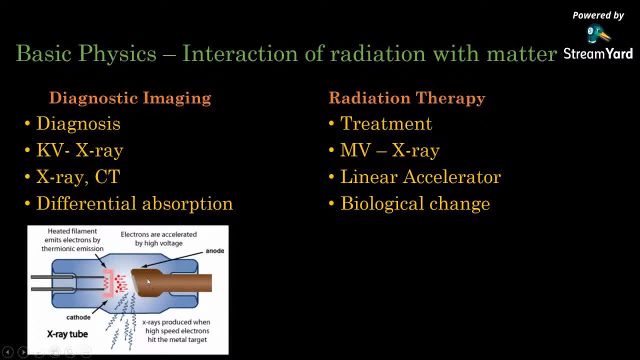 That is a cathode of the tube and that is the anode, And we know that electrons are accelerated using a high voltage from The electrons emerge from a heated filament by thermionic emission. You heat the filament and the electrons come out, and then you apply a voltage across the cathode and anode and the electrons are accelerated towards the anode. 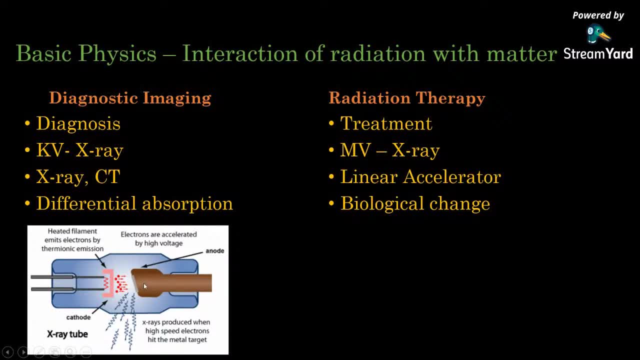 When the electrons come and impinge the anode, they undergo something called a bramstrahlung, or the sudden stoppage of the electrons, whereby the energy that was carried by the electrons are converted into photons and thus X-ray is generated. 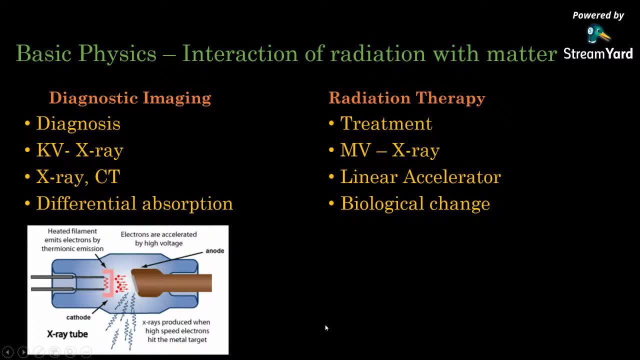 You can see X-rays produced when high-speed electrons hit the metal target, and that is what leads to the bramstrahlung, which in German it actually means by breaking radiation. Breaking not as in break to B-R-E-A-K, it is actually B-R-A-K-I-N-G which is the break, as 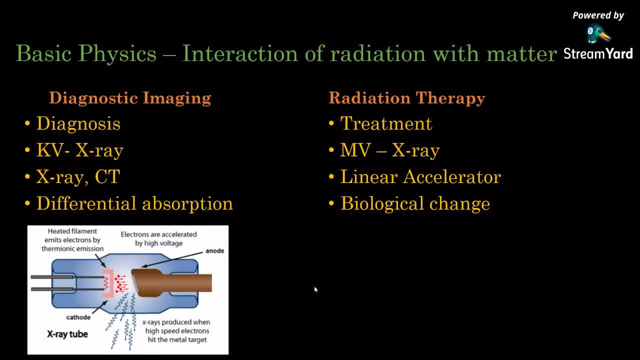 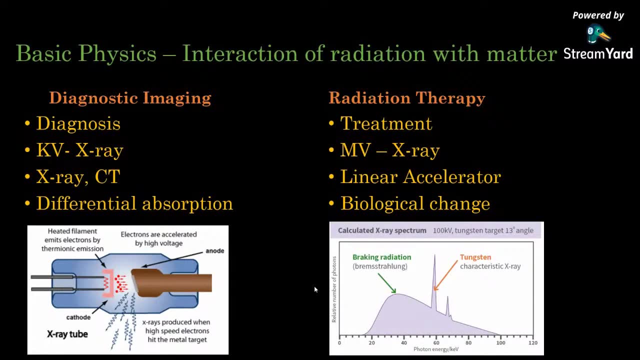 Like stop. So when the X-rays or the electrons stop at the anode, the energy is converted into radiation or into X-ray And eventually it leads to something called a spectrum, and you can see that that is a bramstrahlung spectrum. 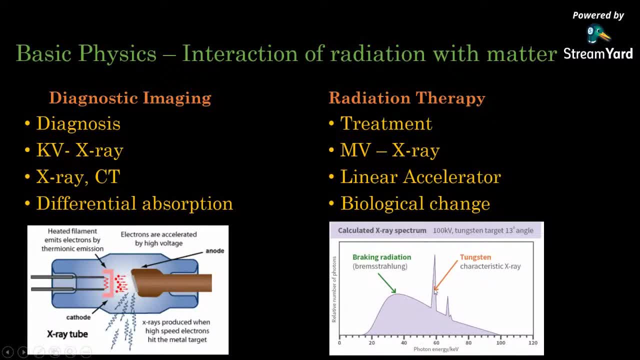 It is not monoenergetic. You can see, for tungsten, which is one of the very common targets used, that is the characteristic X-ray, which the physics students would definitely be having a bit more understanding Of what characteristic X-rays are. so bramstrahlung as well as characteristic X-rays are produced in this, in this phenomenon, and it leads to the production of a spectrum. 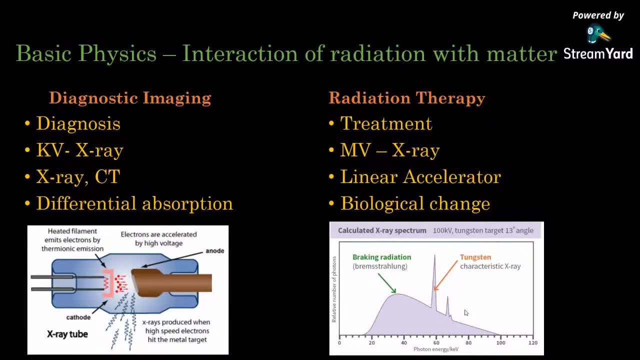 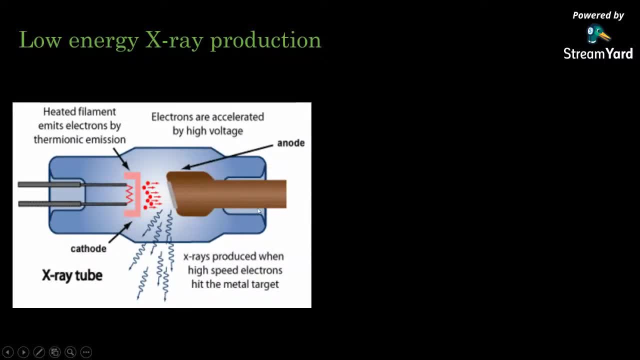 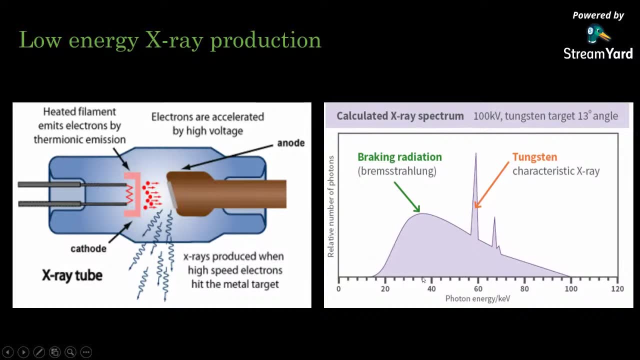 So it is this spectrum that is used in in diagnostic imaging. so low energy X-ray production. This is- this is exactly what I have said- the same picture, and you can see, focusing on this spectrum here, the relative number of photons versus the photons. 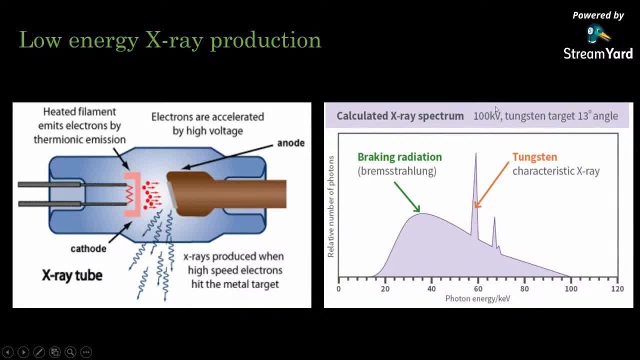 You can see that when 100 keV, 100 kilovolt, is the voltage or the potential difference between the cathode and the anode, the maximum energy of the photons generated is 100 keV. Which means if there were electrons in this process, if there are electrons that has got 100 kilovolt or 100 keV energy, and if, when, in the process of them bombarding with the target. 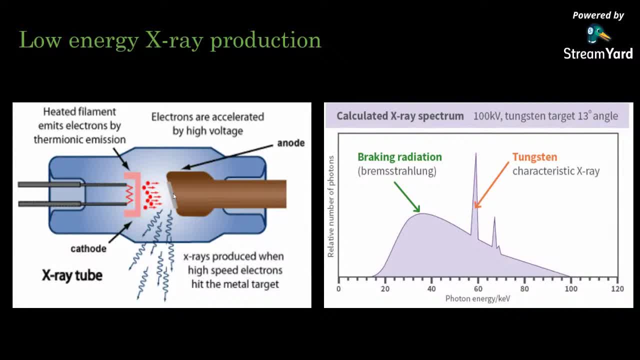 if they manage to transfer all their energy into X-ray, then those photons which are generated will have 100 keV energy, Whereas not all electrons actually convert their energy into photons and hence, depending on the amount of energy that is transferred by the electrons, there is a spectrum that is generated. 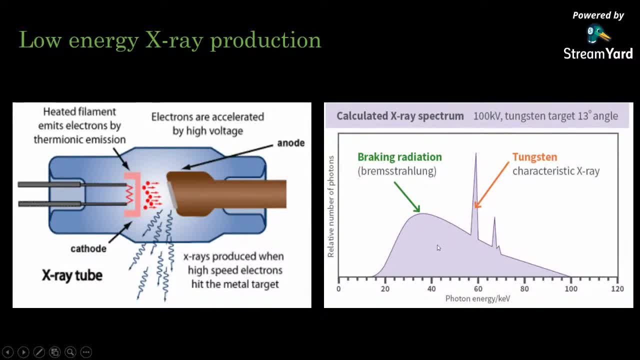 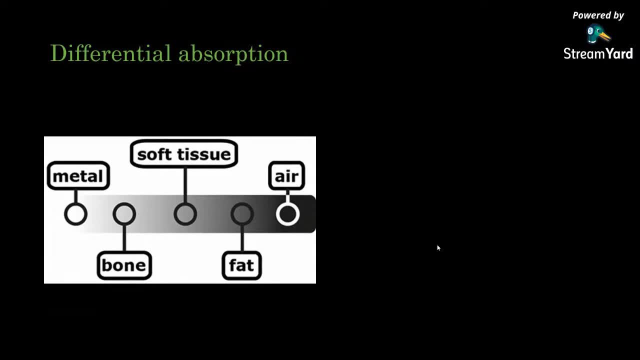 So it is this spectrum or this photons that is used for imaging purpose? Then what is Differential absorption? So you can see now, if you put a material in the beam line or in the path of this X-ray, depending on the density of the material, they transmit the X-rays differently. 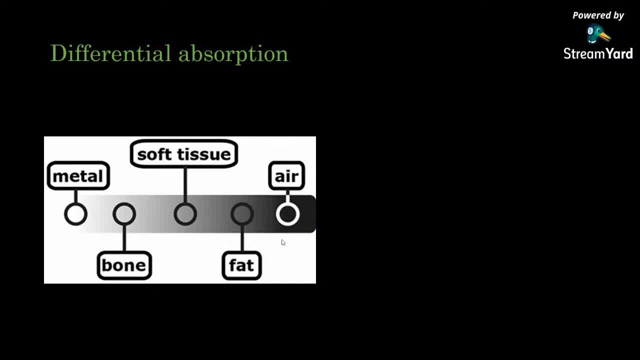 It is more like if you were to have light coming from one end and if you were to put different material in the path of the light. the amount of light that is transmitted through different material differs based on the thickness and the density of the material. 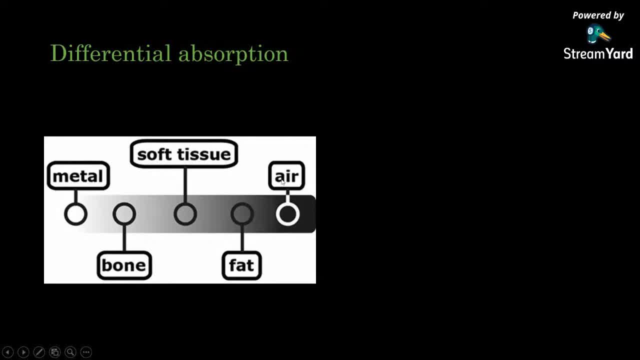 So it is a similar concept whereby you can see, air passes most of the X-ray without any stoppage or without any absorption of the X-ray. There is only very, very, very little amount of X-ray that is absorbed by air. That is because in air, being gas, the atoms are sparsely populated and the cross-section or the chance of interaction of atoms to the X-ray or to the photons is very low. 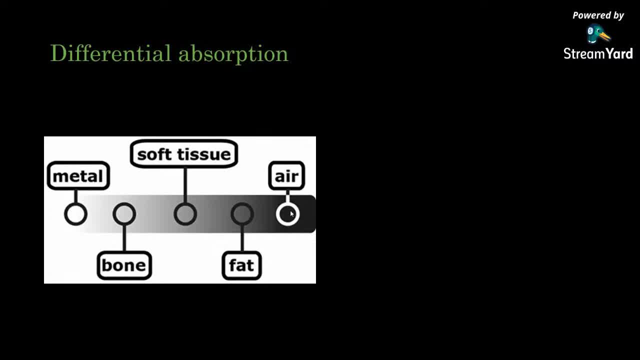 The chance of interaction of photons is very, very limited. Hence there is very little chance for the atoms to absorb the energy and hence reduce the intensity of the radiation. So air absorbs the X-rays very little, whereas fat absorbs it a little bit more. 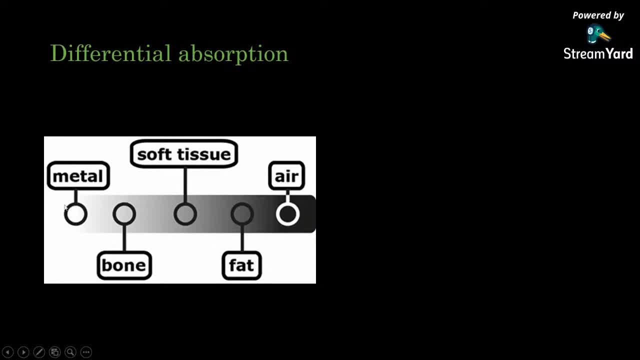 Soft tissue absorbs it even more, Bone absorbs it even more And metals absorb most of the X-ray. But again, there are X-rays that can easily penetrate through metal. But if you were to look at the X-rays in the room in the range of diagnostic imaging, which, as I said somewhere around from 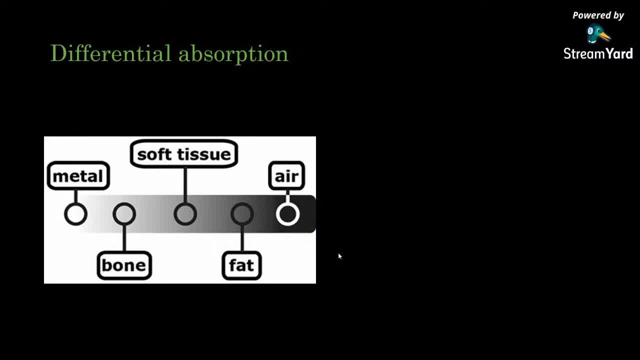 say, even up to 20 kV, to around 120, 150 kV. in that range of X-rays, metal pretty much absorbs all the X-ray And this leads to: or this is what I call, or in scientific community we call: 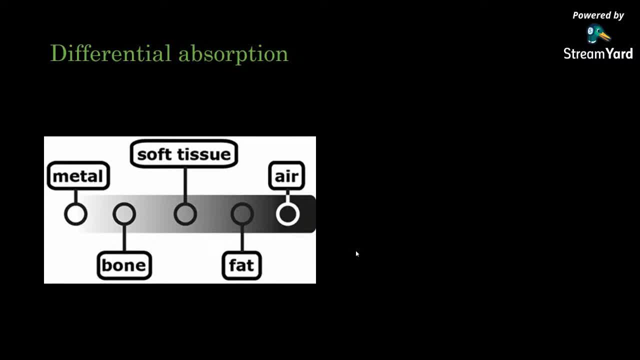 the differential absorption, whereby different material, based on their density and other physical properties, absorbs X-rays differently, which then, if a uniform fluence of X-rays were to enter into a subject, Then, depending on the material density of the subject, the exit X-ray or X-rays that comes out of the body, is not the same as that went in. 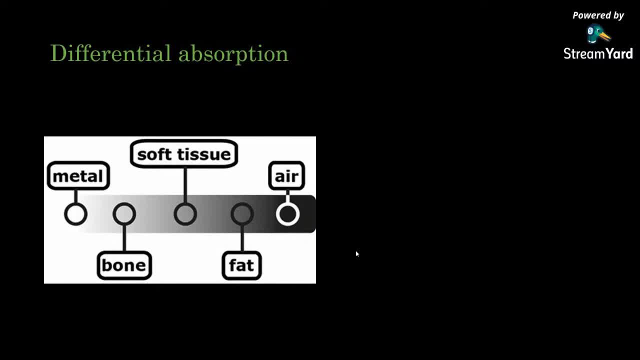 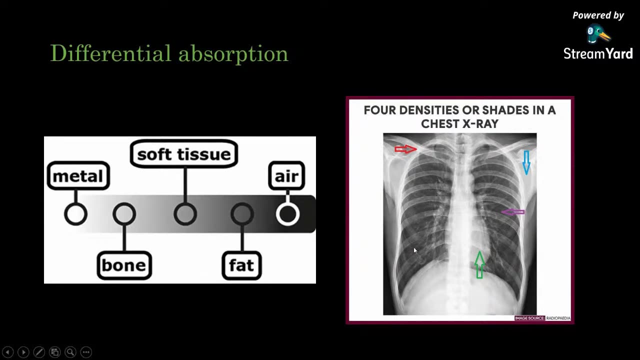 The one that comes out is having a differential fluence as a result of the absorption, or differential absorption by the different materials, And this is a classic example of a chest X-ray. So now, looking into these two pictures side by side, I'm sure you will be able to tell me which one is which. 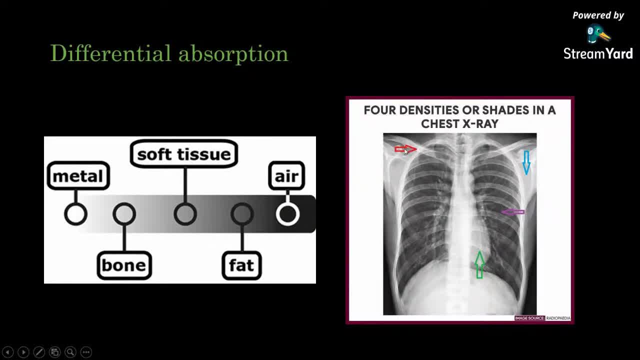 So you can see the one in the red arrow is has definitely absorbed a lot of radiation and that is something closer to bone density. So you can see bone here and that density looks very much like bone, Whereas something that is a little bit less is more like a soft tissue here. 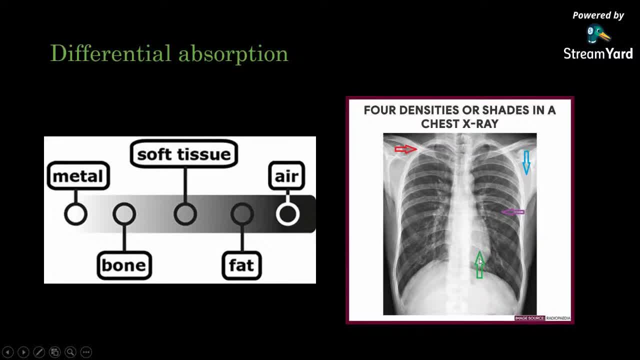 Then this is: that is the green arrow points to something: soft tissue, which is more hot, And then you can see that is the fat deposition, which is the blue arrow, And what is lungs is the air cavity which is in the purple arrow. 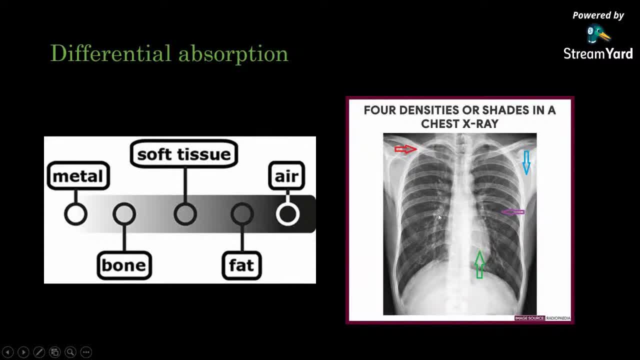 That is what the air cavity is. So this is a classic example of four different densities or different shades that comes out in a chest X-ray when X-rays pass through. So it is a differential absorption of X-ray by different material What leads to the production of an image. 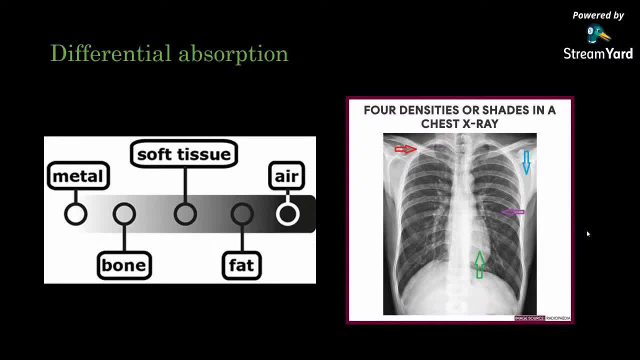 then it is all about converting that fluence that comes out at the other end of the subject. converting that into a visible image is what is all left. So that is done by. in earlier days that used to be done by using a photographic film. 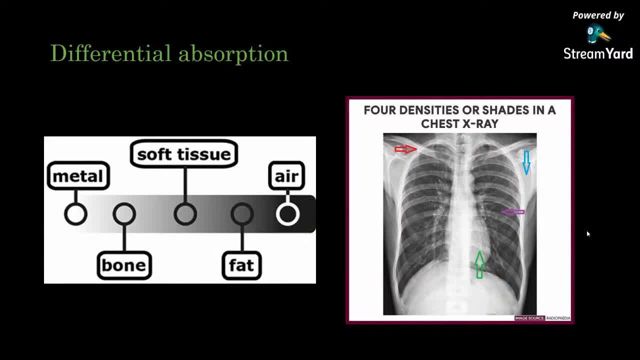 But modern day X-ray machines actually use a digital imaging technology. So that is, that is, the conversion of a digital and analog image to a digital image, and then we do not need to wait a few hours or days before we actually get the image and a result of the of the examination. 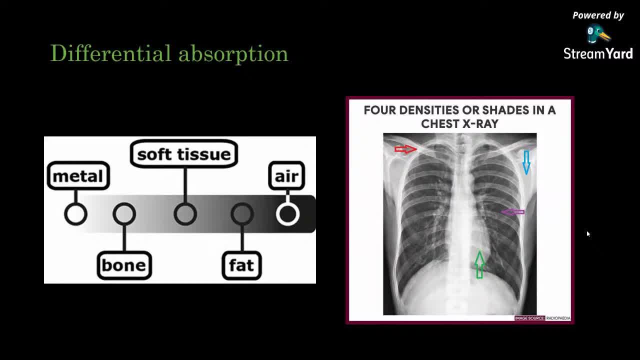 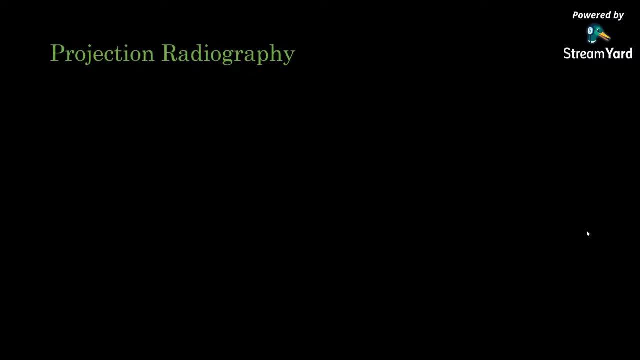 These days, the digital images appear instantly and we might get a report within 30 minutes of the Procedure being taken. So that is. that is how advanced these imaging technology these days are. I'm keeping an eye on my time. I think I've got another half an hour left. 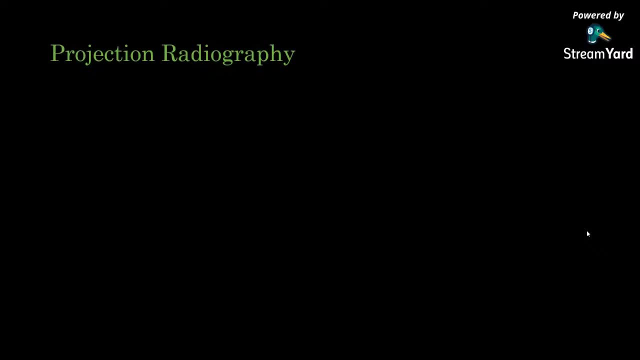 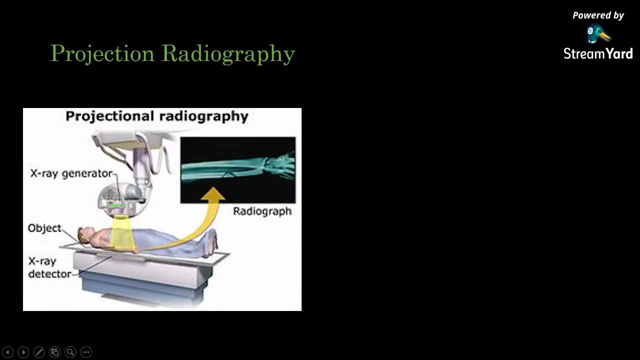 So what we have seen just now is what we call projection radiography, Whereby, as I said, in projection radiography there is an X-ray generator, which is a mobile which, which is mounted on a mobile arm, with all the electromechanical circuit that is connected to the arm and the object. 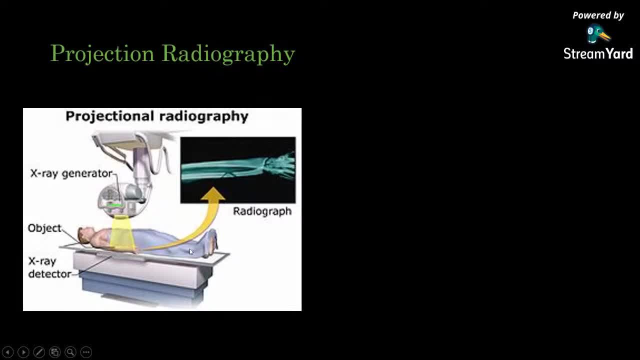 or the the subject that is being examined lie down or stand up on a on a couch, And then there is the X-ray detector that is right underneath the object And then, once the X-ray beam is turned on, it is usually turned on for a for a millisecond or a few milliseconds. 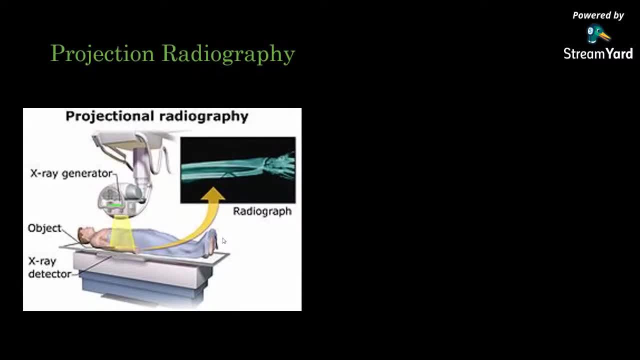 So it's not like a long exposure, because as the exposure is long, it can lead to artifact in the image which is more like a blurring of the image which people deals with. Photography knows that very well, even with a mobile phone. 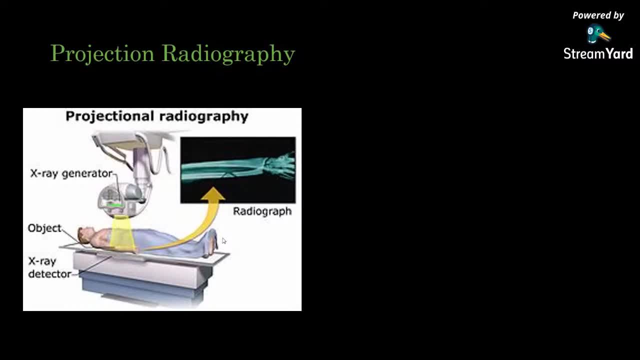 When we try and take a picture, if we keep the, keep it for too long or if the object moves, then we know that there is a blurring of the image, And the same thing can happen here in in projection radiography as well. 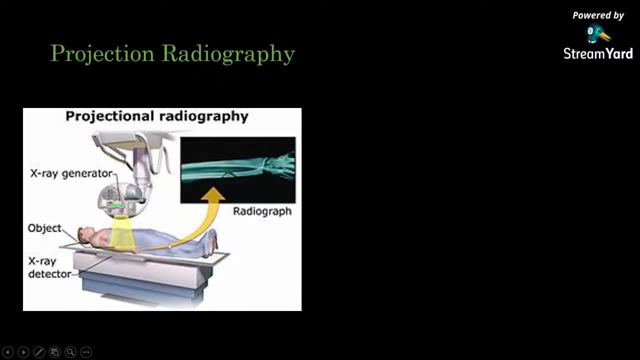 But the one thing that you need to be aware of is that this is this is called a projection image, whereby we know that the object being examined is a 3D volume or is a three dimensional object, But the image that we get is all squashed into a two dimensional plane. 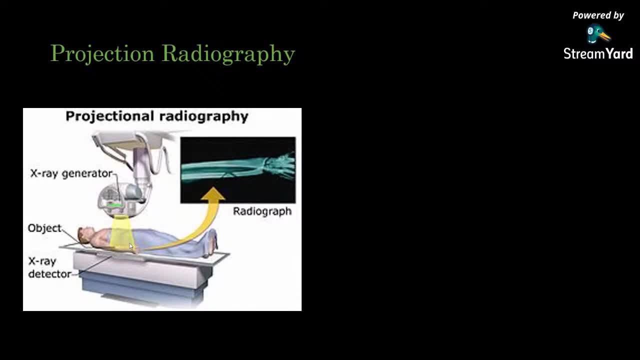 So if we think of a chest X-ray, we know that there is heart and lungs and other organ in the in the beam path. Same with abdomen. You know if you, if you image around or take an X-ray around your abdomen or a tummy. 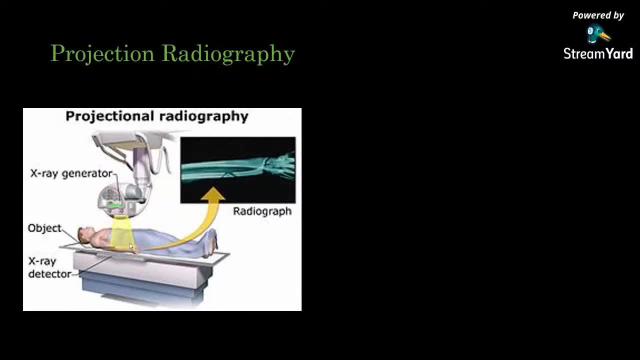 We have got quite a number of vital organs in there Which will be all in the image. They will all be squashed onto the one plane And it is difficult to find out which organ is which, unless you are an expert. So what I mean here is, when you do projection radiography, the amount 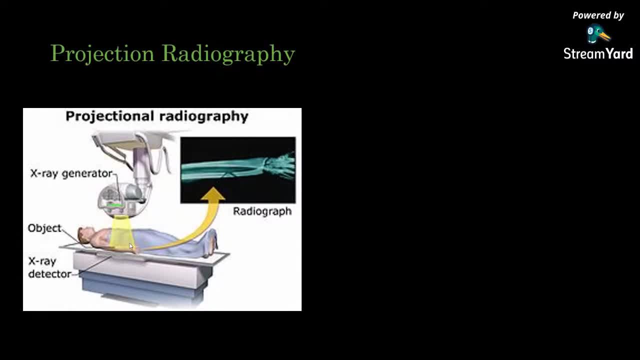 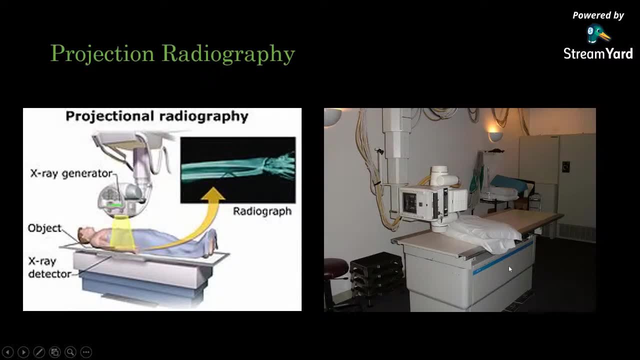 of information. the radiographical information that we get is limited, that you have to be mindful of. So this is a typical X-ray machine, as as most of us have been to an X-ray lab or an X-ray facility Once in the lifetime and have seen this machine. 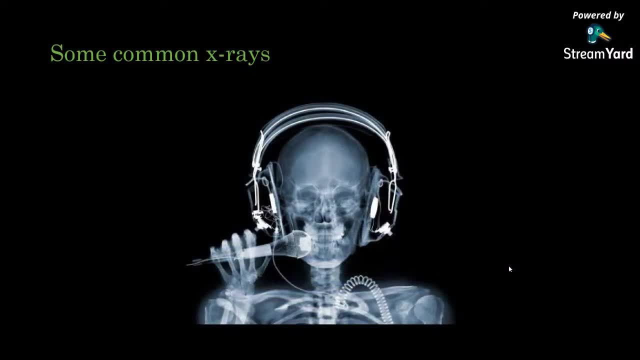 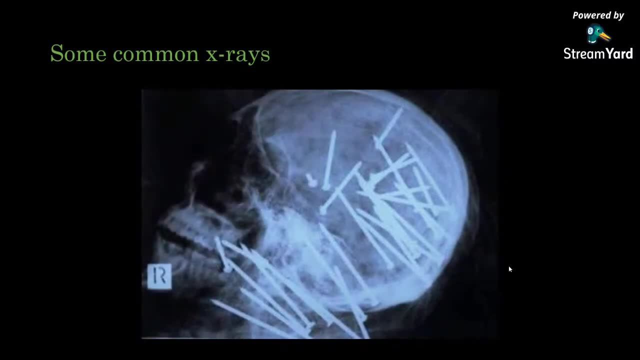 Some common X-rays. even though I say it's common, it's very uncommon. This is a digitally generated X-ray. This is a very common X-ray If you Google on or if you go on Internet and look for funny X-rays. 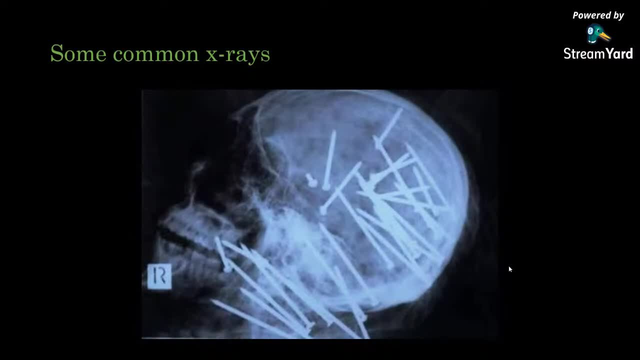 you can see some of them. This is not as funny as it looks. This is an accident happened from a nail gun and a number of nails actually penetrated through the skull of a of a human being And you can see all the X-ray or the nail that is sitting inside the head. 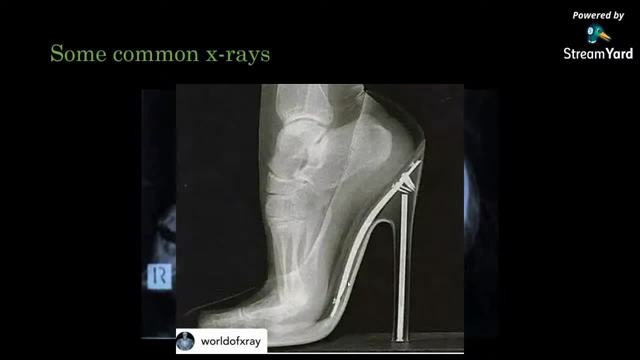 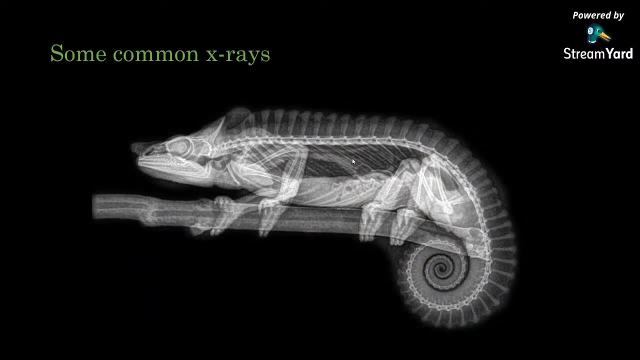 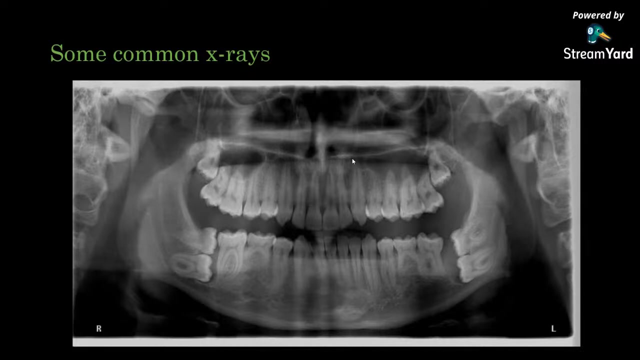 This is something what looks like when women wear high heel shoes. This is what happens to the to their leg. So this is, this is a foot, And look how, how it stands up. This is a, an X-ray of a common organism, And this is a special X-ray technique whereby the X-ray unit 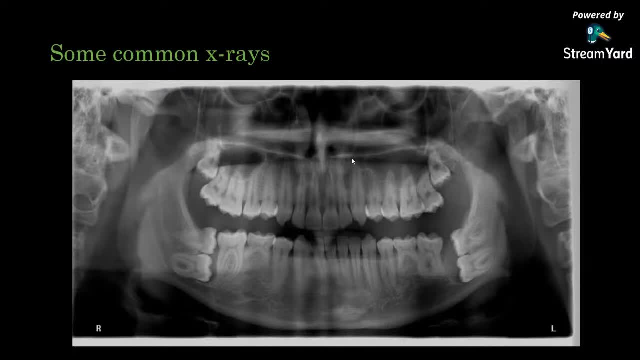 actually goes around your face and take a more like a three dimensional picture. It is not a full 3D, It actually puts images together and creates a 3D effect. So this is- this is the image of which dentists use quite often to see the full. 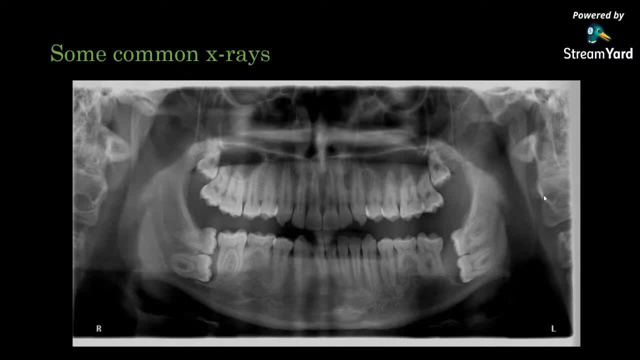 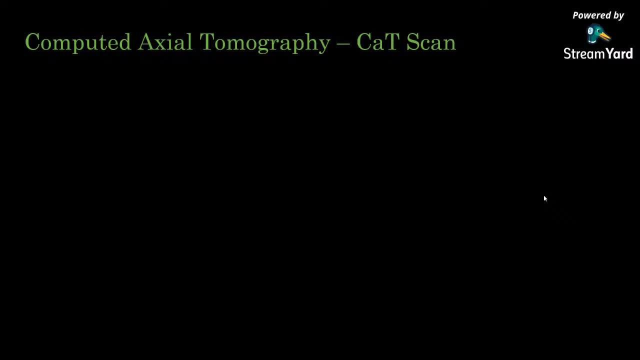 picture of your teeth before any dental procedure is done. Now, as I said, a projectional radiography has got limited information, whereas how we get a little bit more three dimensional information is using something called a computed axial tomography. It it's called a CAT scan, but we we shorten it to say say CT scan. 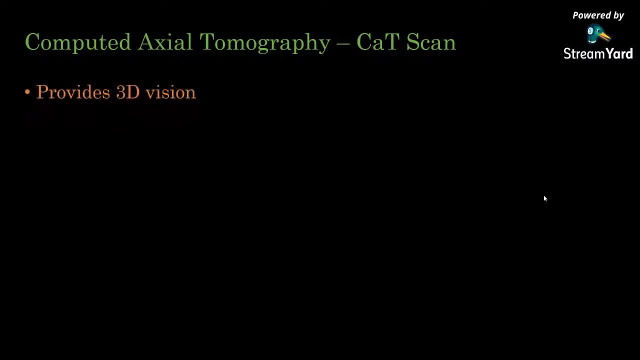 So it is a CT scan technology. What is the basis or what is the use It? a CT scan provides a 3D vision, as opposed to a 2D vision by a conventional X-ray machine. And when I say 3D vision, 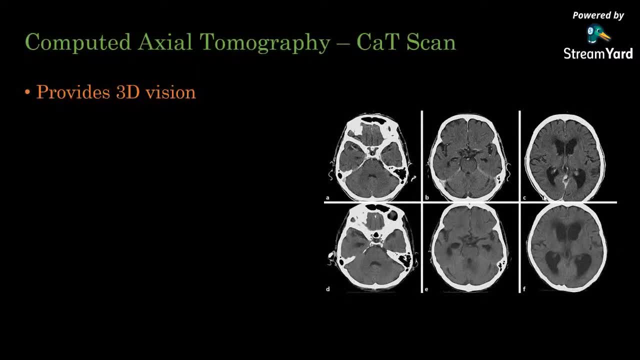 it actually acquires axial slices And this is the CT scan slice of a brain And you can see it takes multiple slices. It is more like the common analogy that I use is more like a slicing a loaf of bread. So you brought a bread from the market and then you suspect that it's been sitting. 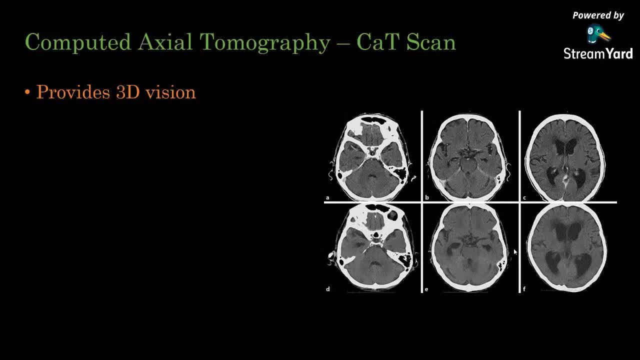 there for a few days and you want to know if there is any fungus. that attack happened inside the bread And is it still usable. So what you do normally is you take a knife and you slice the bread through and find out the slices you make. then the better is the possibility. 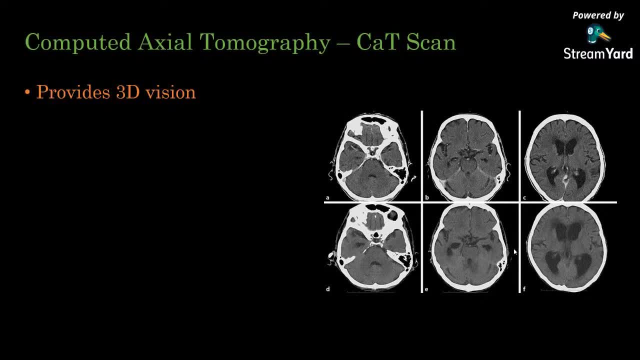 of finding if there is anything wrong with the bread. So you slice it and look through individual slices, And those slices are what we call the axial slices in a CT scanner. Then when you put those slices back together, you actually get the full 3D picture of the bread. 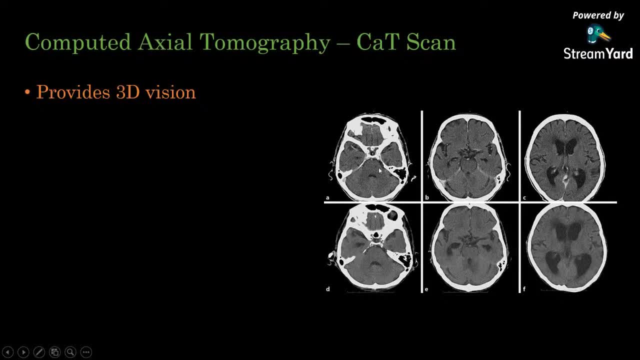 So it is the same concept. It is a very similar concept whereby the subject being examined goes through the CT machine and the machine acquires CT slices and you can see multiple slices acquired of the brain And it gives a much better imaging facility or a capability to identify anything wrong with the organ being examined. 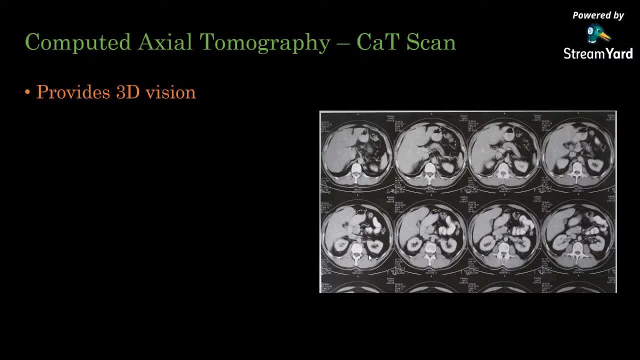 So this is the CT scan slice of abdomen And you can see some of the organs very clearly. That is the liver sitting there, kidneys- I'm sure you will be able to recognize some of them. This is the vertebra. That's a spinal cord that's going through. 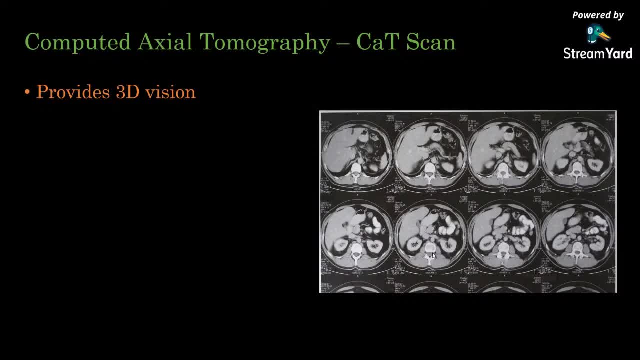 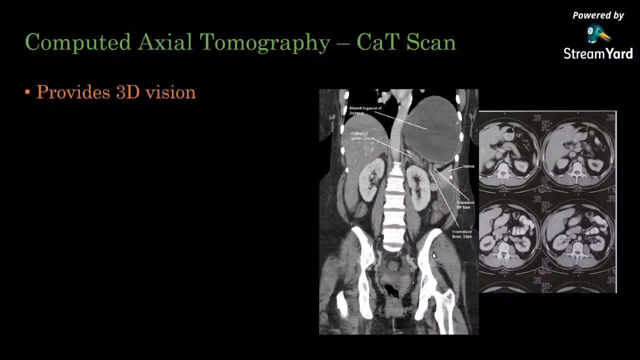 So it's so easy, even for a common man, to go through CT slices and identify some of these. But the good thing is, these axial slices can be then put together to generate other views, like a sagittal view and a coronal view. So this view that you see is what? in medical terminology, you call it a coronal. 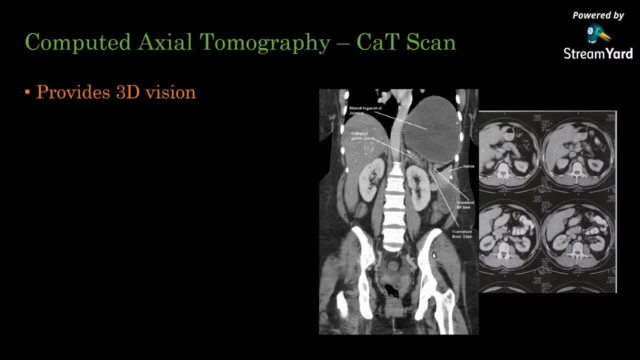 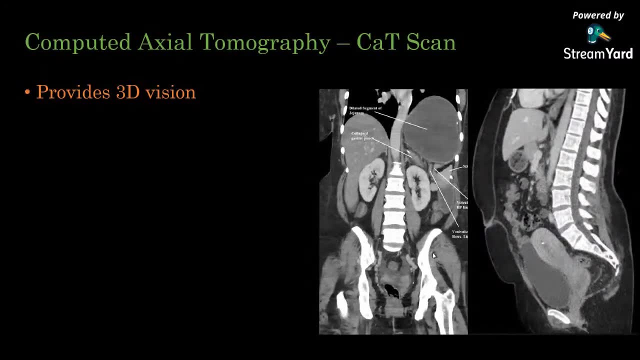 view, or a coronal view, whereby it is more like slicing you from back to front or from front to back, And this is called a sagittal view. This is more like slicing the object from left to right or from right to left. So these views can be generated digitally. 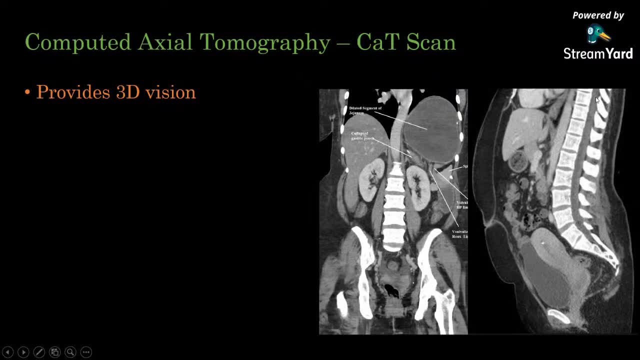 And that gives a very good picture of the subject being scanned. You can see that the spinal cord running through there clearly That is the vertebra. So if there is any collapse of the vertebra, especially due to cancer, that is so easy to find out. 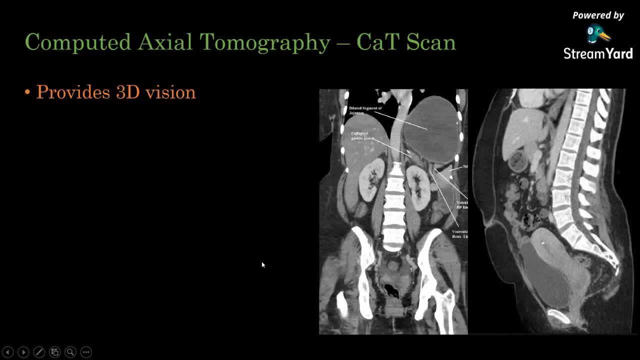 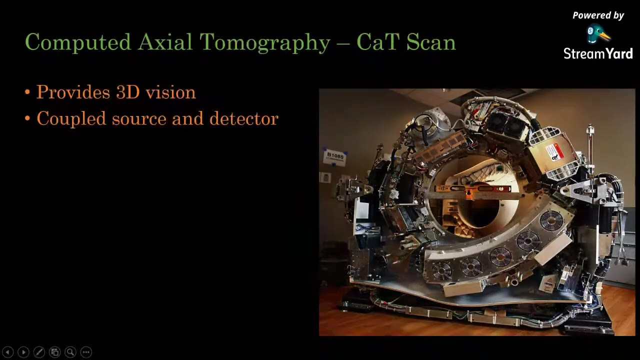 So that is. that is a good thing about having CT scans over conventional X-rays. So how it is done, it uses coupled source and detector technology. So what does that mean? This is a skin off or cover off of a CT scanner And you can see that is again an X-ray unit and an X-ray tube. that is. 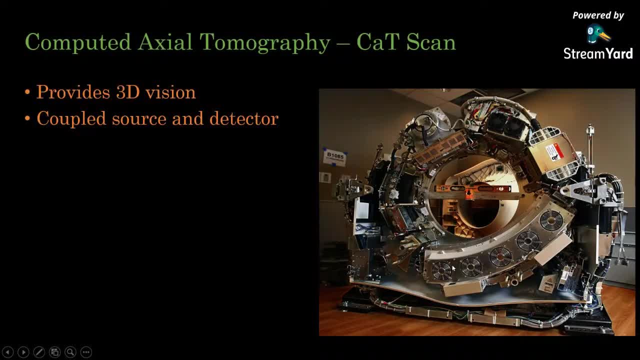 mounted there and that is an array of detectors that is there. So the rest is all the electronics and cooling system and everything that is associated with it. You can see that is the, that is the heart, That is the X-ray tube with its collimation system and all that. 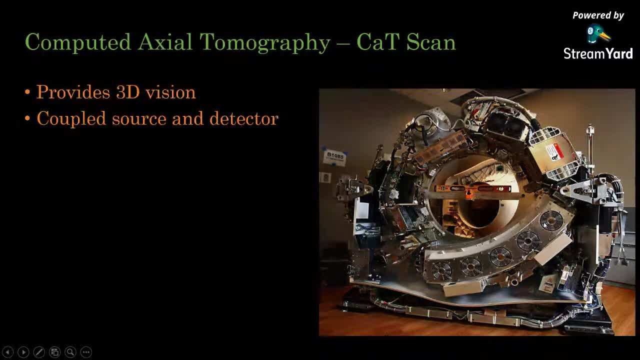 And that is the imaging assembly or the detector assembly. with you can see all the fans that is used to cool the system down and all the electromechanical parts that are used behind to generate, acquire and generate the image. So the good thing is that the source, which is X-ray tube, and the detector can spin around or rotate. 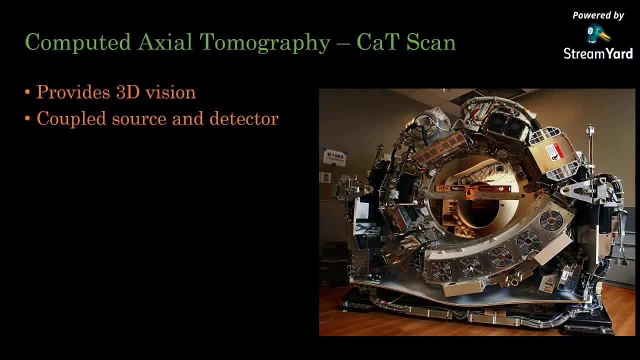 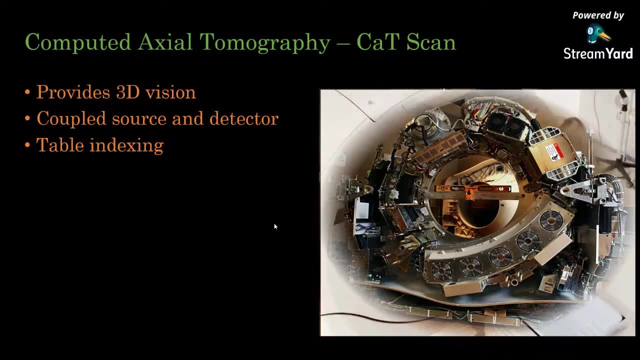 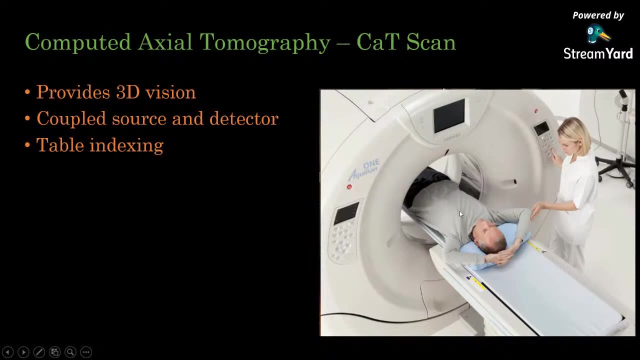 around the patient or the subject together. So that's why I call it a coupled source and detector. And then, once it does it, What? what can happen is you can see when the patient or the person being examined lie down on the table and the 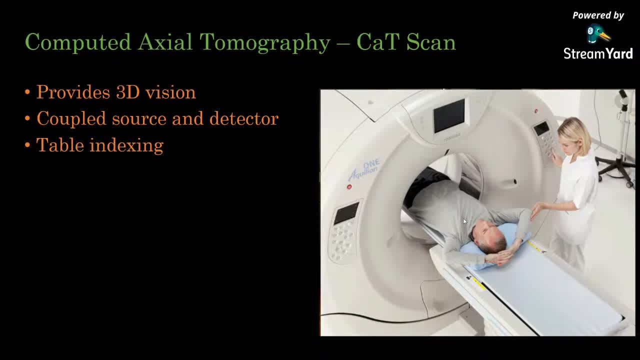 table actually is indexed, which means the table moves into the machine or out of the machine in a in a stipulated manner, in a particular manner, step by step, and then, after every indexing, the coupled source and detector spin around the patient once, and then the table moves again and spin again, and then table moves, spins. 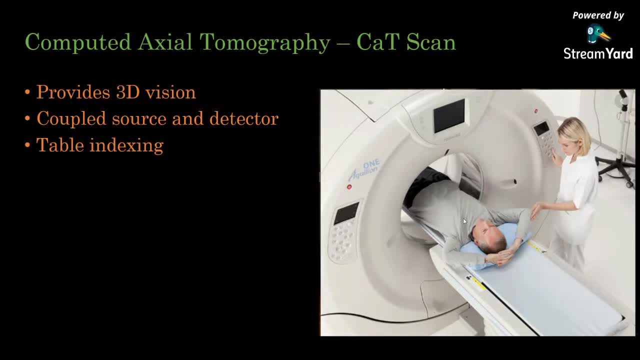 So it is like spinning of the source and detector and movement of the table. So it is done sequentially. So this is one of the early technologies. But these days you don't need to spin and then index and spin an index. You can sort of do it together to acquire the image. 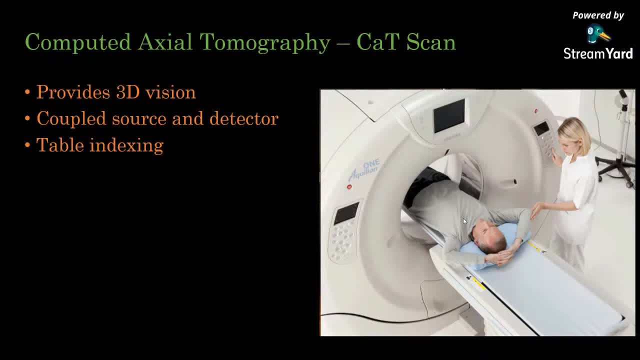 So, but anyway, in a, in a, in a simple way or in a simple sense. it is once you spin the source and detector and then you get one slice, and then you move the table, then the system spin again and then you get the next slice. 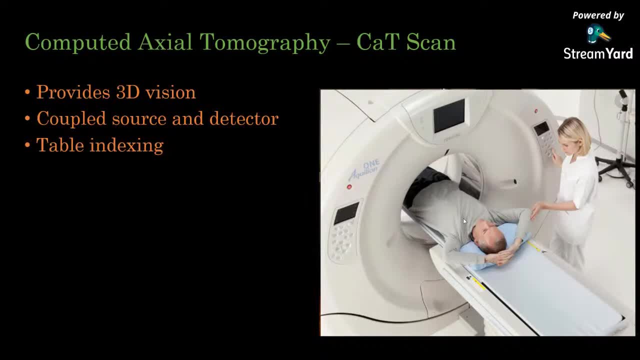 So the CT scanner acquire the image slice by slice. So in every revolution it acquire one slice. That is, as I said, that is the early technology. And depending on the slice or the collimator or the opening of the X-ray source, the slice thickness can be adjusted. 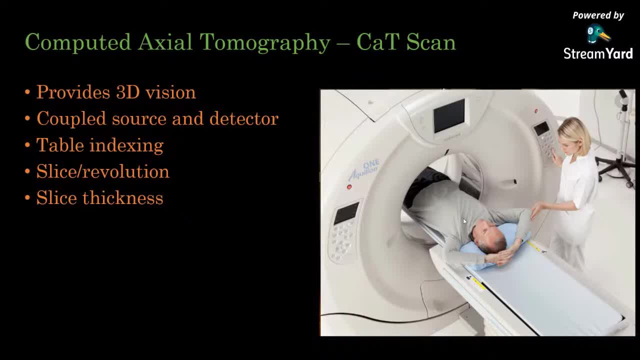 You can do like a one millimeter slice or a 10 millimeter slice or a five millimeter slice. So that's all. those are all things can be set before the scan is done And even after the scan is done, the post processing of the image can be done in order to change the slice thickness. 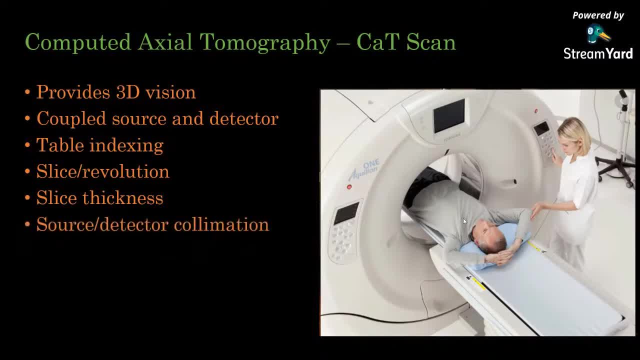 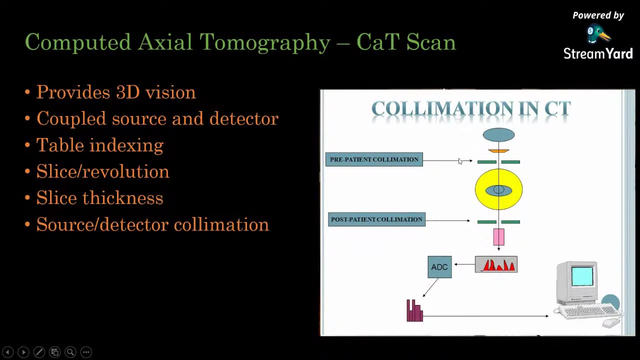 So that's all available technology. As I said, it's To some extent is based on the source or detector. collimation is what decides the slice thickness. So just look at, looking at the collimation. So this is the prepatient collimation, that is a source and that is the prepatient collimation. 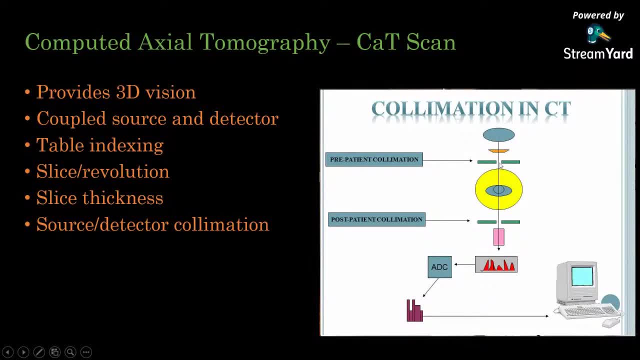 You can actually Move these Collimators. that is shown in the green blocks. you can move it in and out And, based on where it is: as it comes in, the slice thickness decreases. as it goes out, the slice thickness increases. 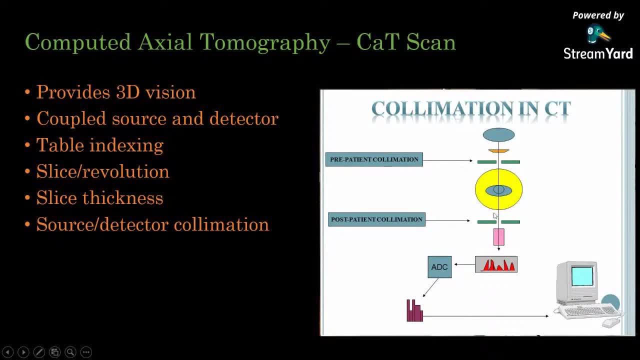 And that's the patient there that's being examined. And you can even do a post patient collimation. That is a detector there that is just before the X-ray gets to the detector. You can increase or decrease. that can adjust the slice thickness. 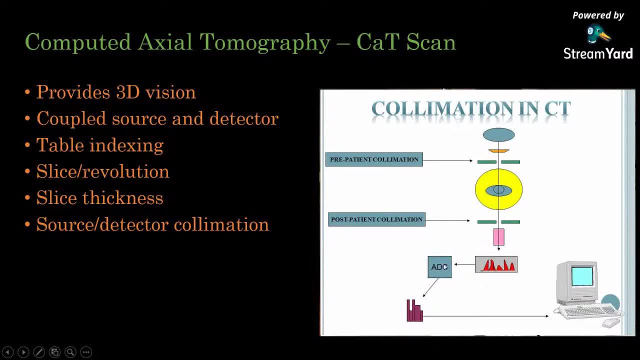 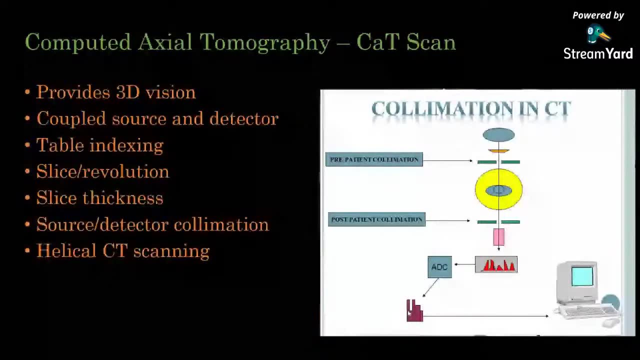 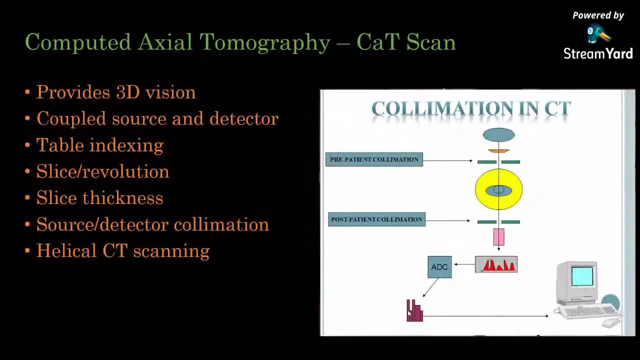 And then you get an image, an analog image, using an analog to digital converter that can be converted into a visible image. Helical CT scanning doesn't use one full revolution to acquire one slice. It actually uses partial revolution to acquire one slice. The advantage is you can actually acquire images faster. 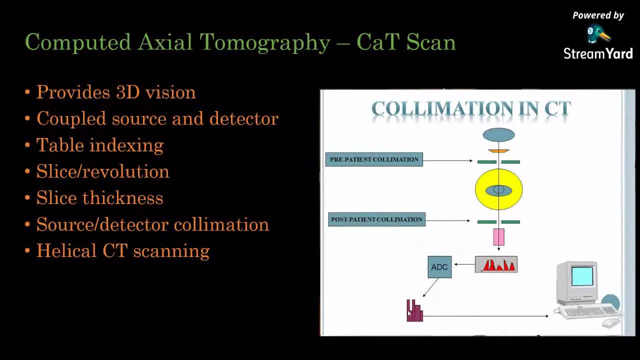 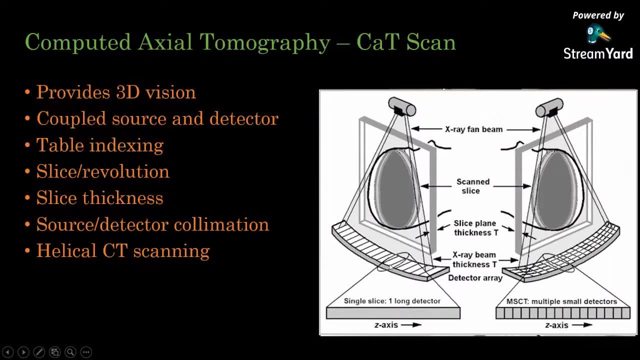 And helical CT scanning technology is a state of the art in all modern day CT scanners. So instead of using a single detector, you can see that is a single detector that is used. It uses multiple small detectors And then that allows that along with the helical technology. 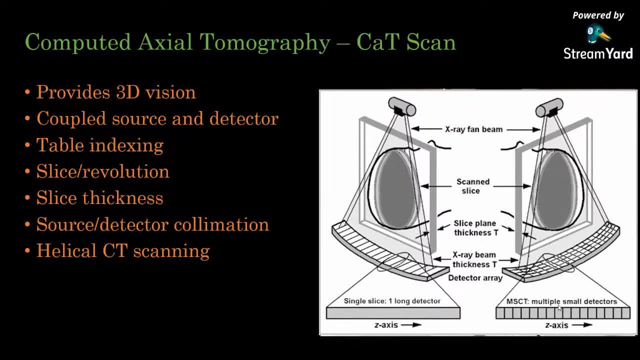 allows you to acquire images really fast, which has got an extremely high advantage in, especially in CT scanning organs that have got involuntary movement within the body, like the lungs and the heart, and all that. even there are organs that moves involuntarily within the abdomen. 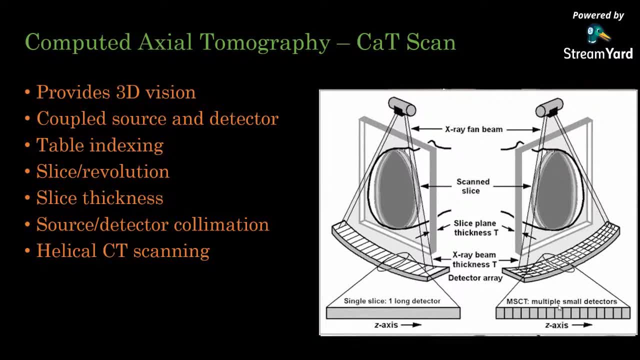 So in order to image those, those organs, fast imaging is helpful because faster the imaging, less is the artifact or blurring of the images. You get a high amount of information or a great signal to noise ratio when imaging becomes faster. So helical scanning technology is actually. 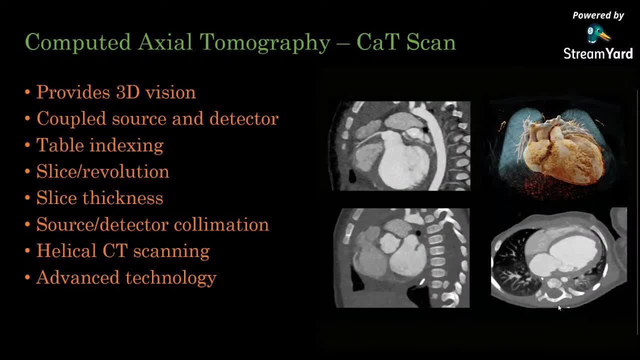 one of the advanced technology that is used in CT scanning. So you can see- so this is, this is a gift of the- how the image would look like once a scan is done, and you can see how a post-processed image looks like. That's the image of the heart. 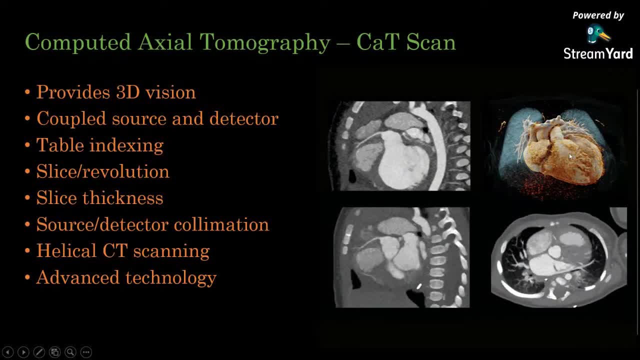 And these are. these were things that we couldn't think of maybe 30,, 40 years ago, when, around 1970s, when CT scanners were first invented And the two scientists who invented the CT scanner actually got Nobel Prize in medicine. So not not in physics, but they actually got the Nobel Prize in medicine. 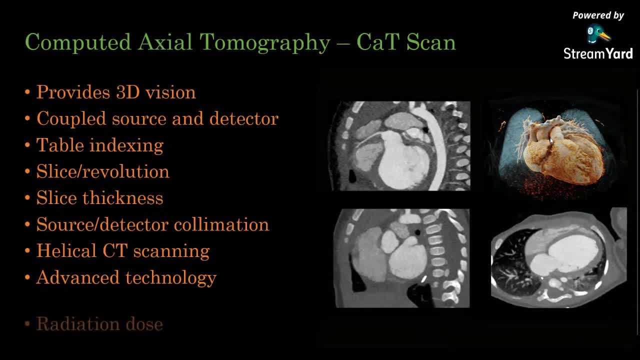 That tells you how important this technology is in modern day medicine. But the one thing that you have to be mindful of is the amount of radiation dose that the person gets, because these are people who may or may not have disease by using radiation. It can actually lead to some. 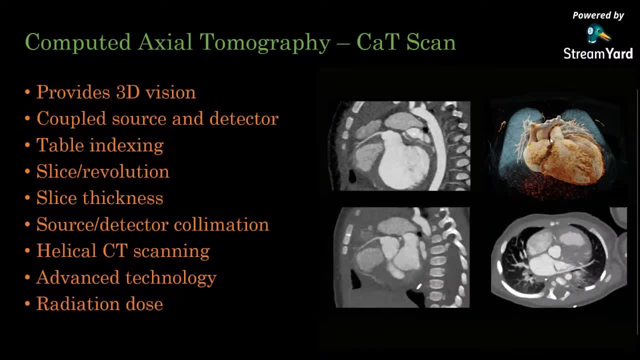 Is a really, really low possibility of radiation induced cancers in subjects that are undergoing these sort of procedures. That is why there is a philosophy, general philosophy, of using radiation devices in imaging. It is the justification of the practice If you can achieve the same image quality. 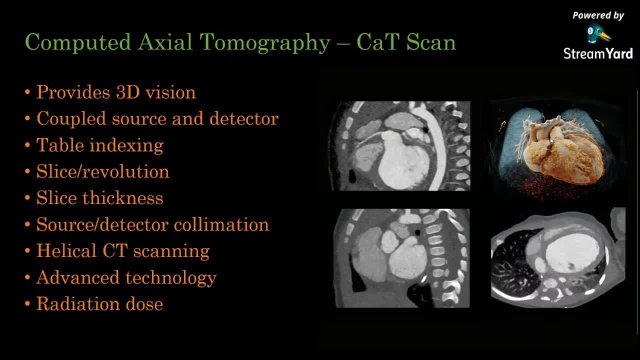 and clinical information can be derived without using radiation, then those technologies should be used. for example, if you can use MRI, MRI or ultrasound scanning to get the same clinical information, then you should- should not use X-ray or CT scanners. that is justification of the practice. 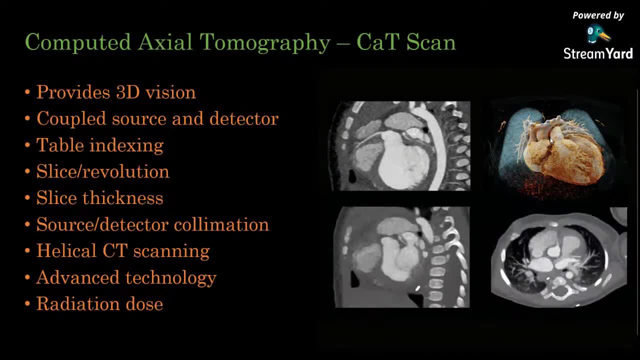 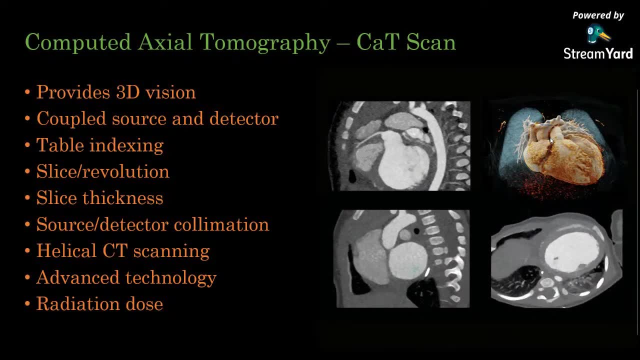 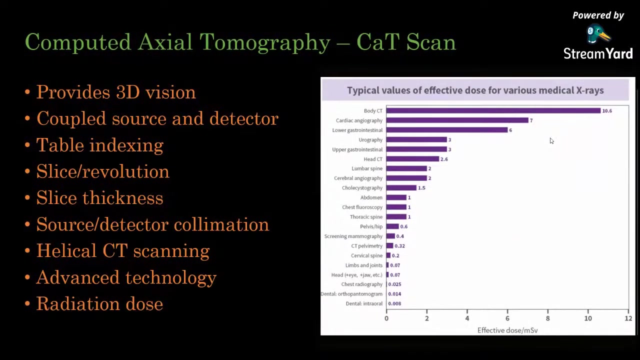 And then if a particular subject needs CT scanning, then the practice must be optimized, whereby the best technology and best practices should be used in clinic, And that is what we call the optimization of the use of radiation. So these are some of the typical values. 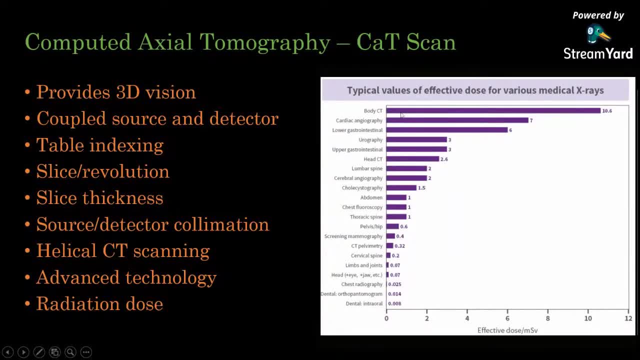 of effective dose for various medical X-ray use. You can see a whole body. CT has got around 10.6 millisievert- That is a unit of effective dose- and cardiac angiography is less lower gastro. I don't want to be spending a lot of time going through each and every one. 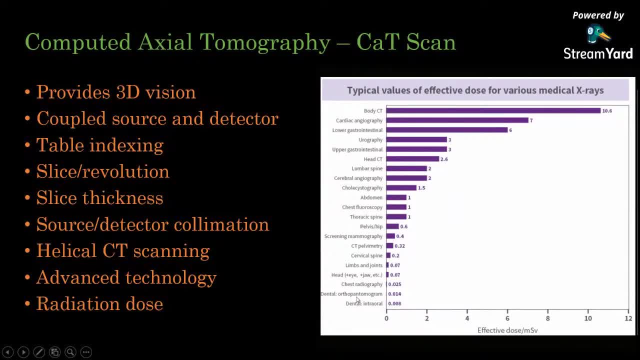 You can see dental X-rays and dental ortho pantomimogram that I showed you before, which was the whole the picture of the entire jaw and teeth. it's really really low compared to a cervical spine or a head CT scan. this is sort of the range of doses. 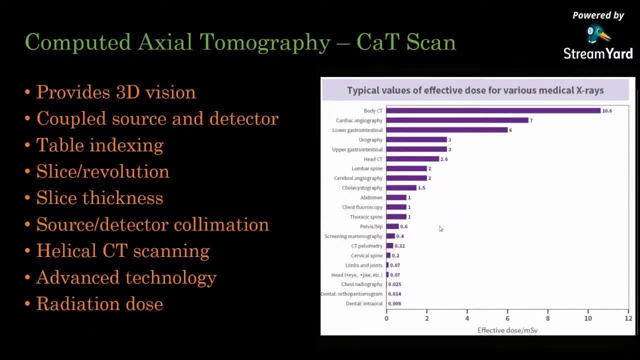 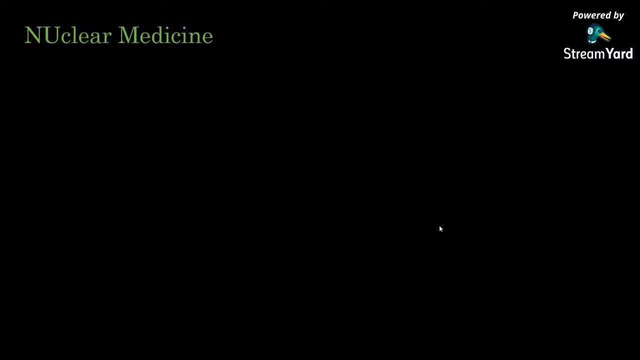 that the subject receives while undergoing such procedure. Now, as I've gone through almost my bulk of my time, I will now move on to some of the most common diagnostic- radio diagnostic- procedures that we use in our daily life. Now, moving to nuclear medicine, as you can see, this compared to radio diagnosis. 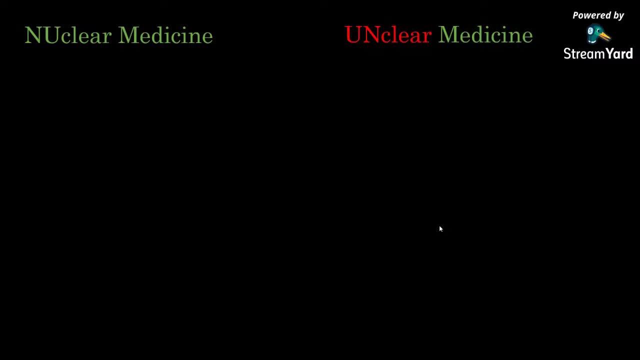 this is a very unclear medicine. at least when I was a student This was a bit of a confusing topic, But with some of the guidelines from, or teaching from, some of the great, eminent professors from BARC, this is one of the fascinating. 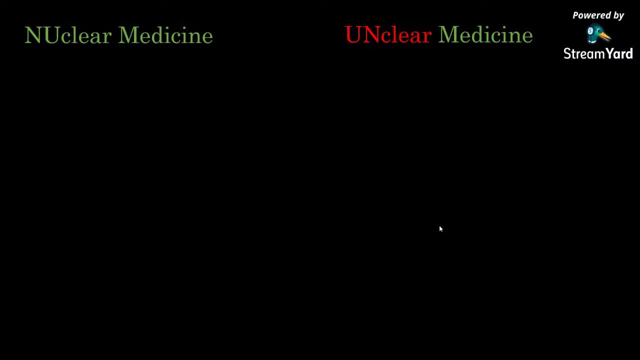 fields of medicine that I've or use of radiation that I've seen. The amount of clinical information that you can derive from using nuclear medicine is is phenomenal. You can see it's a medical specialty that use the application of radioactive substances in the diagnosis and treatment. 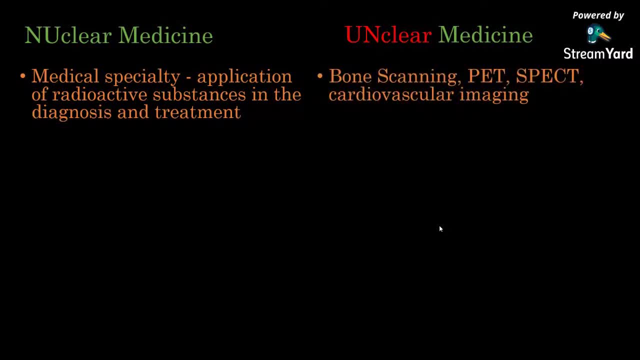 But today I will focus only on the diagnostic part. Some of the very common procedures used are bone scanning, PET scanning, SPECT scanning, cardiovascular imaging, renal imaging. So there are quite a number of nuclear medicine procedures that we use on a daily basis. So what it does is small amounts of 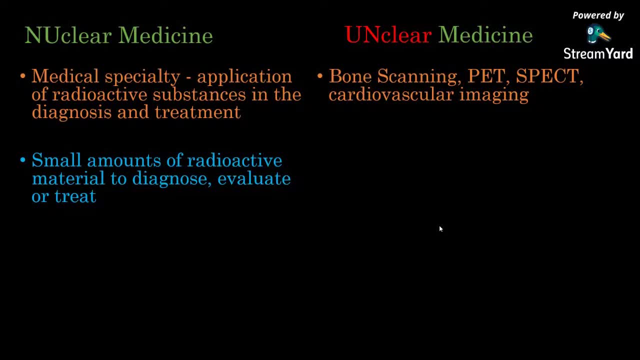 radioactive material is used to diagnose, evaluate and treat, So it uses radioactive material that goes into the body. So clearly the first difference is a diagnostic, radio diagnostic procedure using an X-ray machine. The source of radiation sits outside the person, So you have an X-ray source that 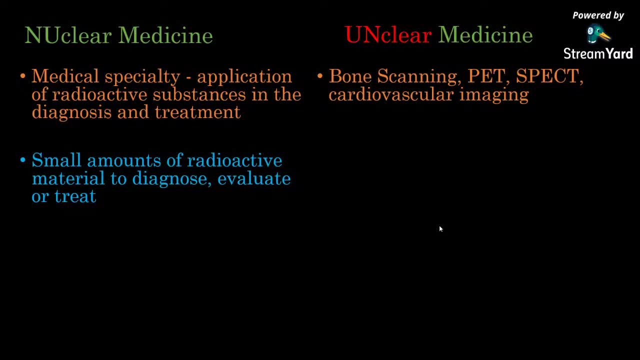 is outside the person and X-ray comes into, Whereas in nuclear medicine small amounts of radioactive material is actually administered into the person being examined And that person act as the source of radiation, And then detectors are around that that person, detecting the radiation coming out. 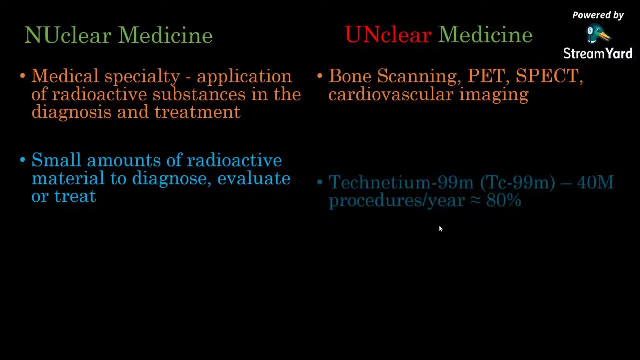 of the person and images are developed based on that. The most common radioactive material used, the workhorse of nuclear medicine, is technetium-99M, the isotope 99M of technetium. Around 40 million procedures are performed every year around the world. 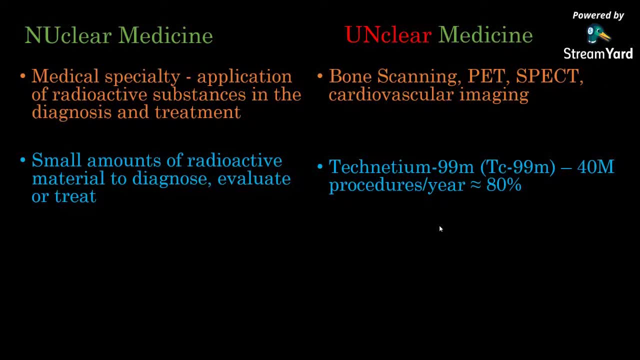 out of which, which actually is about 80% of the total nuclear medicine procedures. that is done, So you can see how important technetium-99M is in the field of nuclear medicine. So radioactive traces, which are called radiopharmaceuticals, are used to assess the bodily functions. 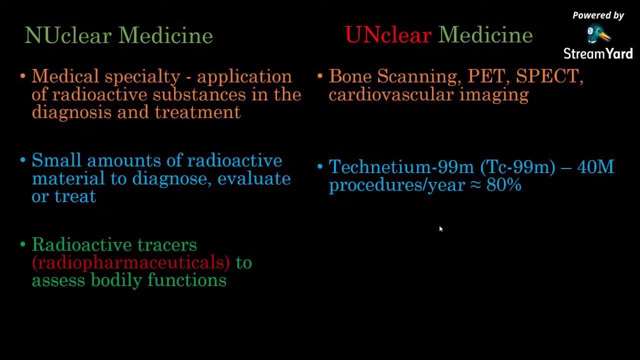 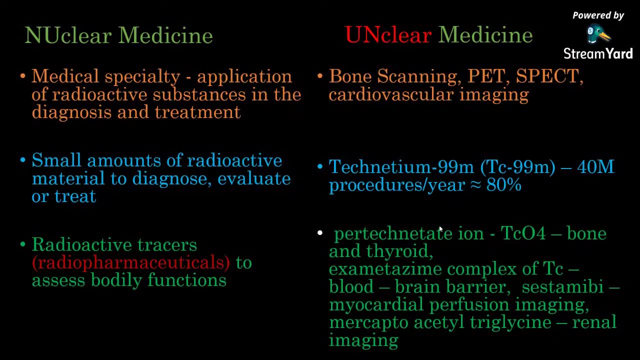 You can see it is not interested in the body anatomy, It is more in the functioning of the body. Some of the some of the techniques used is with technetium-99M. Technetium-99M is a radioactive tracer, but when it is mixed with or tagged, 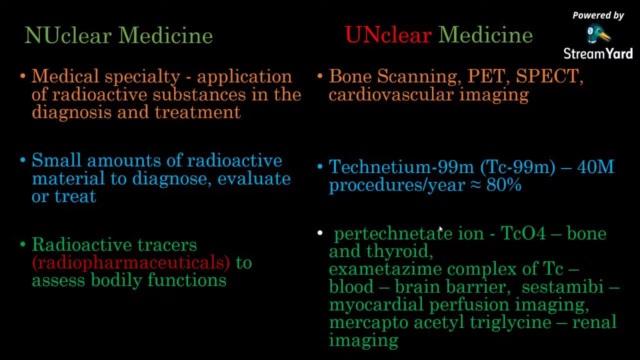 with certain other chemicals which the body can absorb. it is called a radiopharmaceutical. So radiopharmaceutical is what is administered into the body, whereas radioactive tracer is the. is is a core radioactive material. The pharmaceutical is is actually made from the radioactive tracer that is administered into the body. 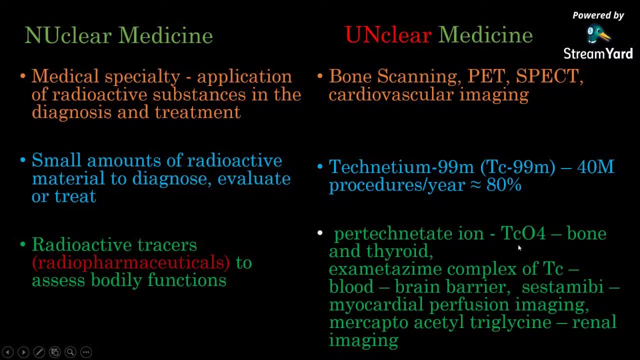 You can see. the pertechnate ion of technetium is used for bone and thyroid scanning. Eczematosome complex of technetium is used is it has got a property of breaking the blood brain barrier, because we know that there is a huge 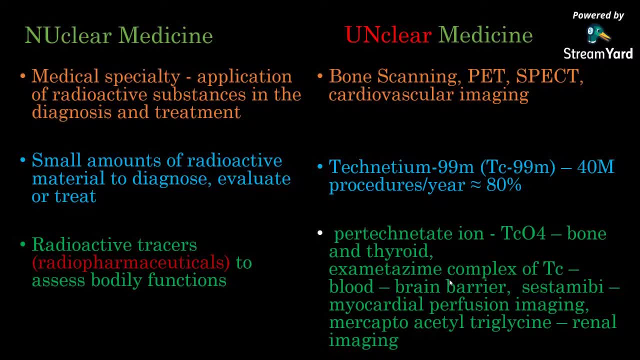 barrier between the rest of the body and the brain, called the blood brain barrier, whereby brain doesn't allow toxic substance to get into the brain and using its mechanism called the blood brain barrier, But in order to scan the functioning of the brain, this eczematosome complex. 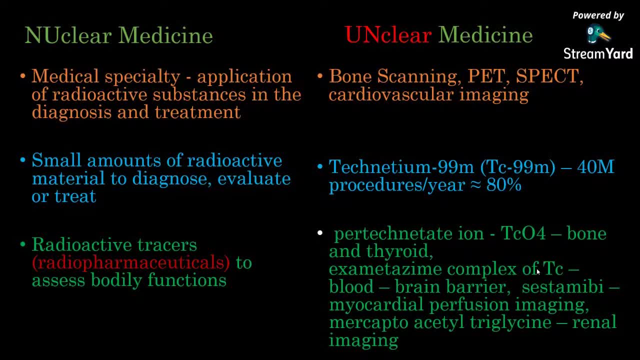 of technetium, has the ability to break the blood brain barrier and get into the brain, which helps in imaging brain. Another radiopharmaceutical used for myocardial perfusion imaging, which is imaging the heart and the the ability of the heart muscles to function. 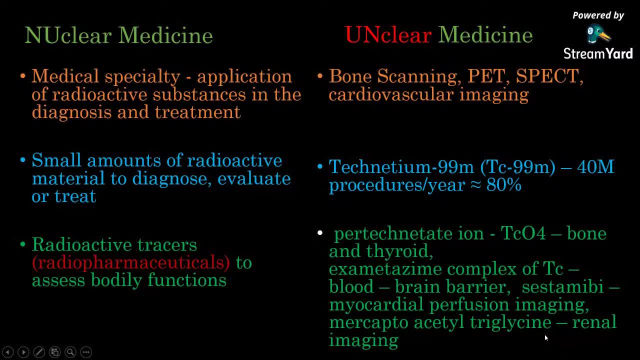 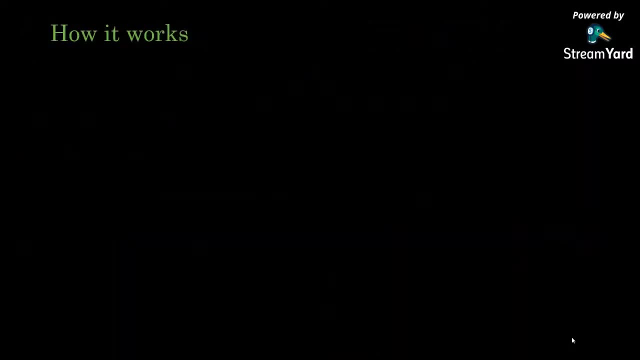 And mercaptoacetyltriglycine is another ligand that is used for renal imaging, which is imaging the kidneys. So these are some of the very common procedures used in nuclear medicine using technetium 99M. So to give a bit of 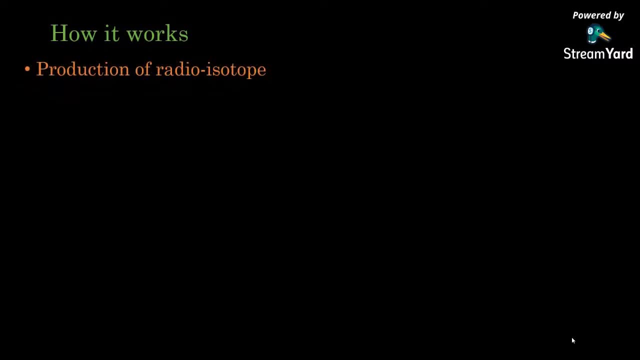 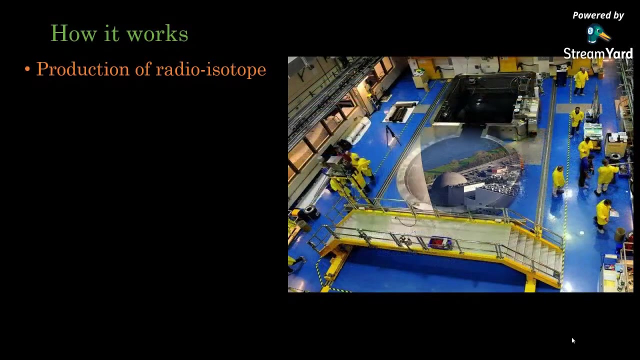 detail of how it works. first is the production of radioisotopes. So these, these, most of these radioisotopes used in nuclear medicine are not naturally occurring. They have to be manufactured, either in a, in a nuclear reactor like this one in leukocytes in Sydney, which provides about 25 percent of the of 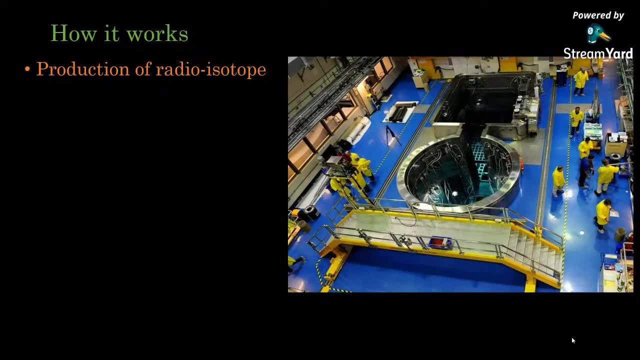 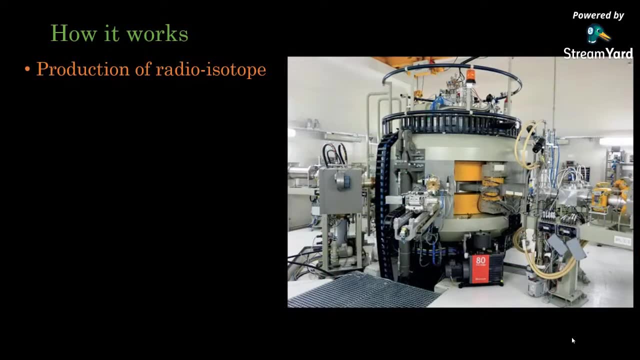 the global demand of nuclear medicine isotopes are met by this reactor in Sydney or by using something called a medical cyclotron, which is is not as big a device as a nuclear reactor. is This? these are? this can be mounted or can be housed inside a hospital itself. 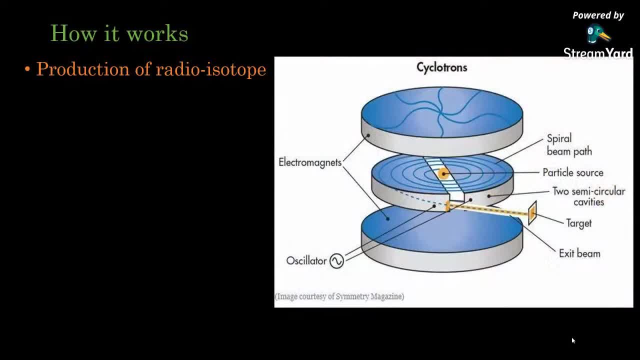 And there are many hospitals in and around the world which does that. In physics we know cyclotrons have got a central portion which has got two D's and electromagnetics on magnets on either sides. when the, the, the particle source, a charged particle, is left in this, in the middle or in between the two D's, 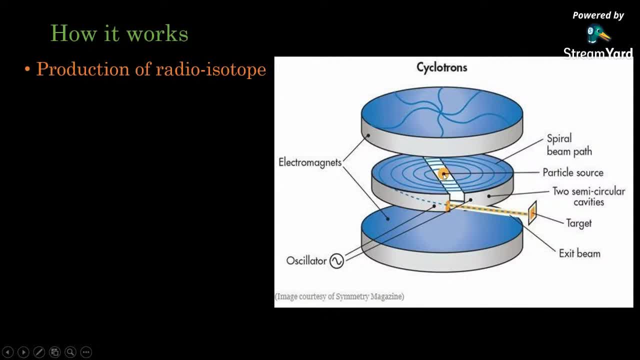 And when magnetic field is applied, when magnetic field is applied on a charged particle, we know it takes a circular path, It goes in circles and as it moves in circle it keeps acquiring the energy And when it comes out with high energy, it is bombarded with a target. 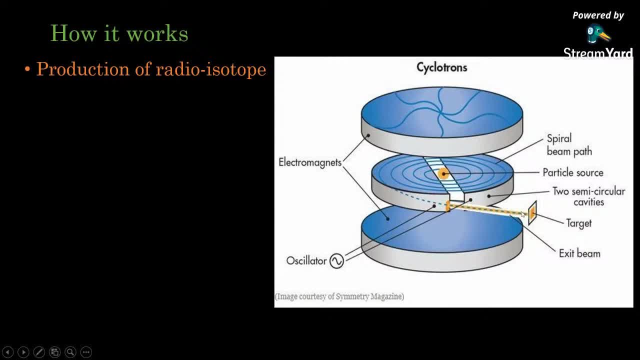 So when the particle, like proton, comes out and hits with a suitable target, that leads to a nuclear reaction, that is leading to the production of suitable isotope. So this is the basis of a medical cyclotron. So once the the these radioisotopes are generated, the reason why it has to be 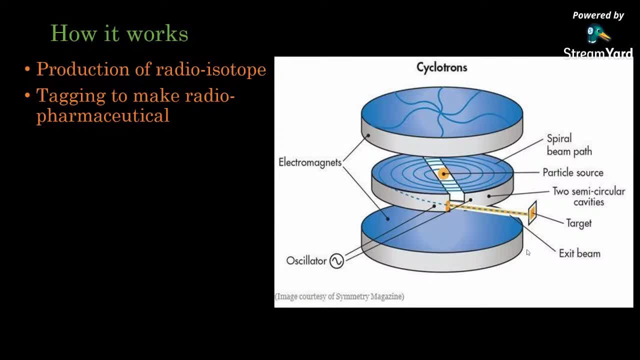 in in some of the closer to the medical facility where the scanning is done is because these are quite a number of these isotopes are short half life. The technician 99M has got only six hours of half life. Fluorine 18,, which is another very common isotope used in PET scanning. 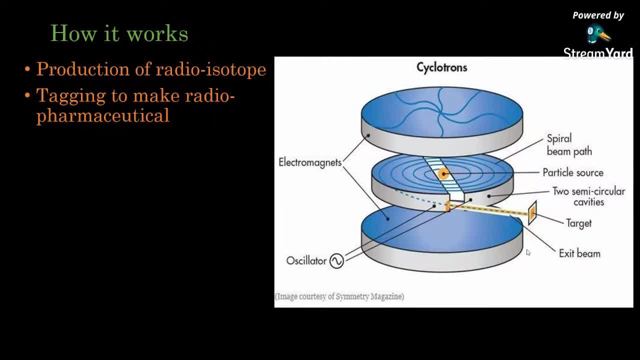 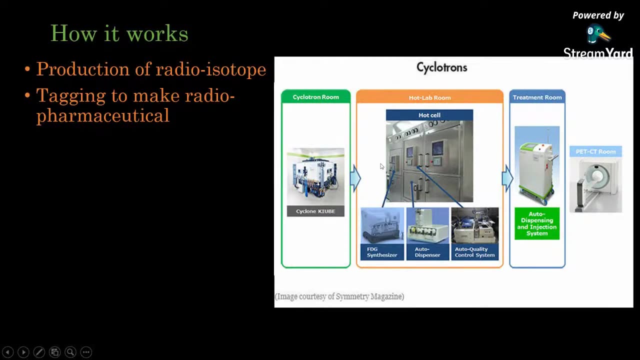 has got only 120 minutes, which is just over two hours of half life. So half life being really low. for these radioisotopes, they have to be very close to where the imaging procedure is done. So once the radioisotope gets to a place called the hot lab, you can see from the cyclotron room. 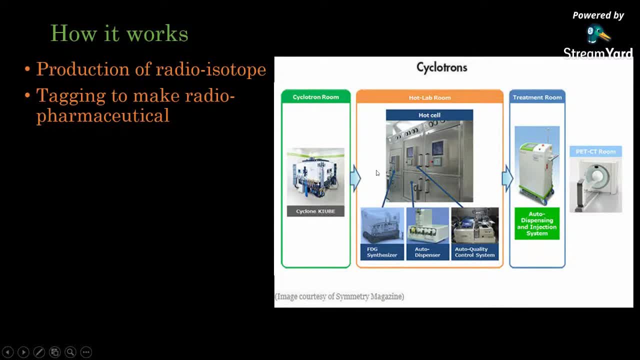 it's the radiopharmacy. the radioisotope is pushed into the hot lab where it generates the radiopharmaceutical and that is using the autodispenser and the quality control is all done and then that is pushed into the treatment room. 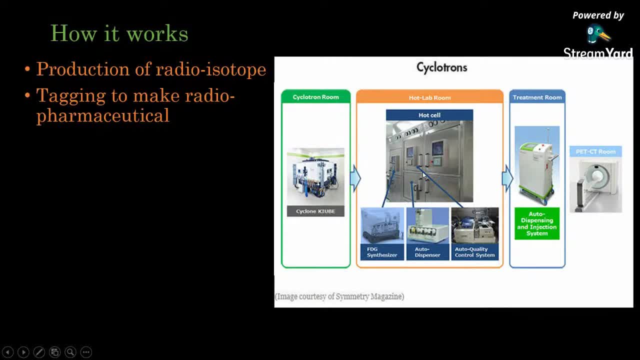 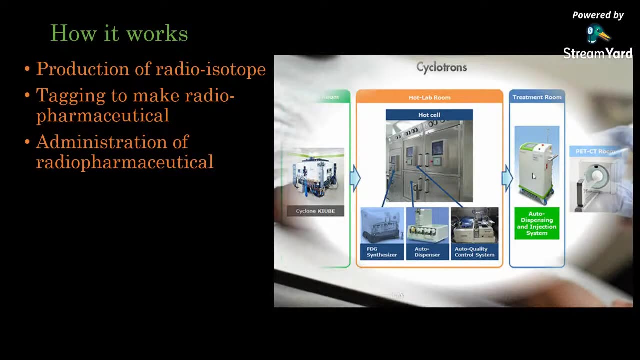 So from cyclotron the radioisotope comes, from the hot cell, It is converted into the radiopharmaceutical and then it is given to the treatment room or to the imaging room. So administration of the radiopharmaceutical happens, And then this is done either intravenously or orally. 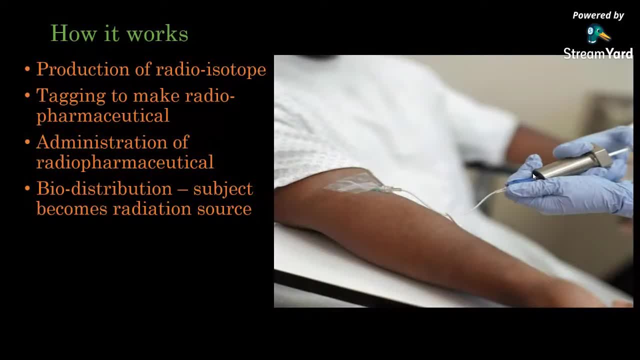 And then the subject waits for a biodistribution to form. So this particular material, along with the radioisotope or the radiopharmaceutical. the speciality is that the material that is tagged with has got properties whereby it will be selectively absorbed in different organs of the body. 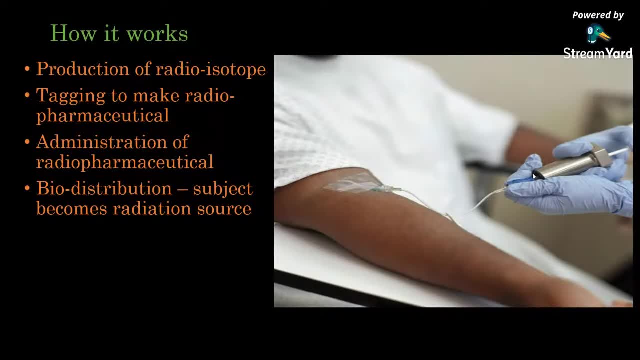 So, as I said, technetium 99M, when it is tagged with different materials, it targets different organs. You can see. it can target bone, It can target thyroid, It can target heart, It can target kidneys. So, based on what is the tagging agent used, it goes into different organs of the body. 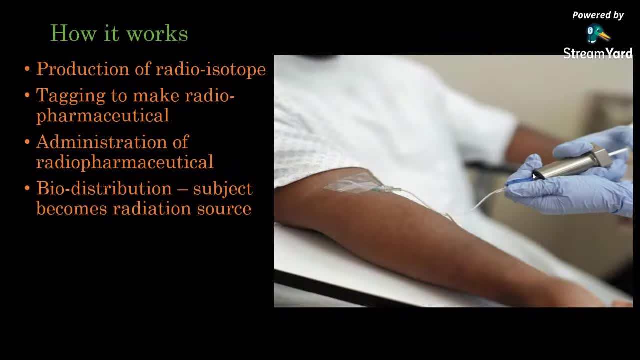 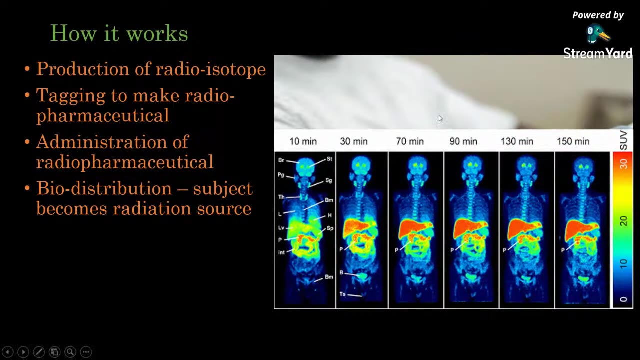 And after a while waiting- for maybe 30 minutes or so, depending on the tracer used- it generates a biodistribution Within the body And then the subject becomes the radiation source. So this is how, what, what happens when a particular radioactive tracer is. 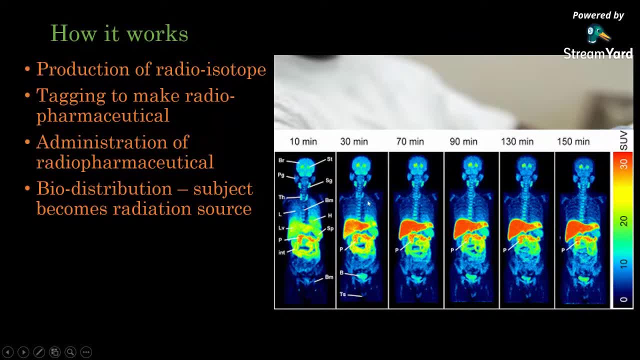 injected or administered into the body in 10 minutes. This is what happens in 30 minutes, So you can see the biodistribution changes as time pass. And then imaging is done, which is collecting and processing of the radiation data that comes out of the body. 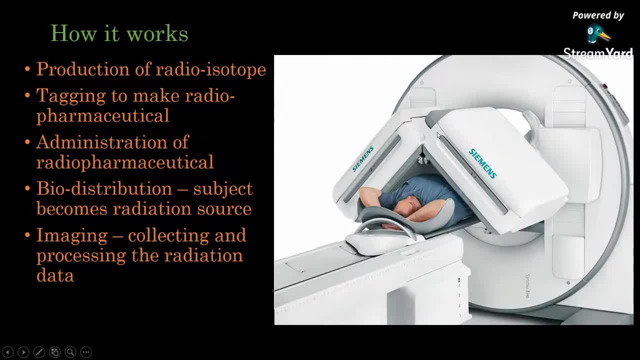 So you can see that is this is a. this is what is called a gamma camera, whereby it detects the gamma photons. So Technetium 99M emits gamma photons of 140 keV And these has got these detectors that is sitting at 90 degree to each other. 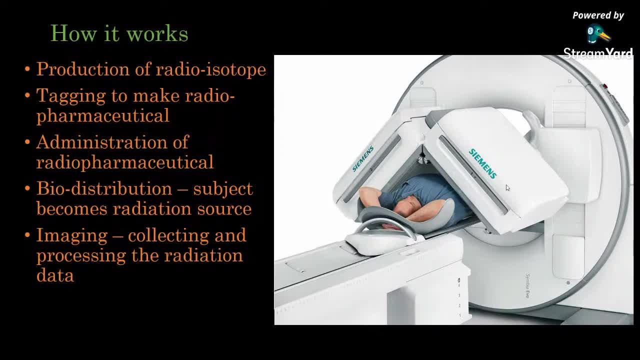 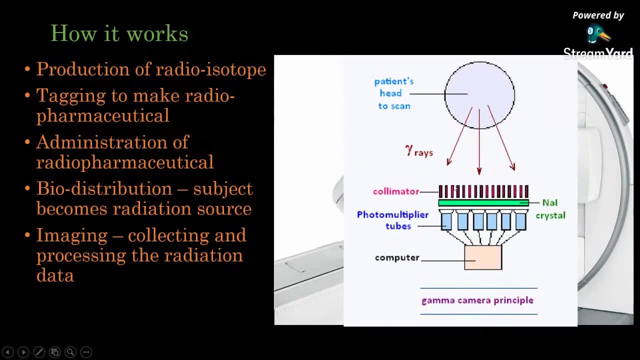 has got detectors that can pick up the 140 keV gamma that comes out of the patient's body and that ultimately generates the image. So those X-rays that comes out are collimated And you can see that is a sodium iodide crystal that is acting as the detector. 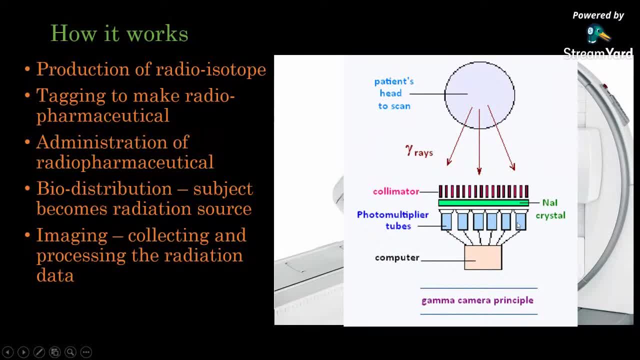 of the gamma photons. that is then fed to photomultiplier tubes, which then is fed into the computer that is generating the image. So once that imaging is completed, the person that has undergone the examination waits for the decay or flushing out of the radioactive material from the body. 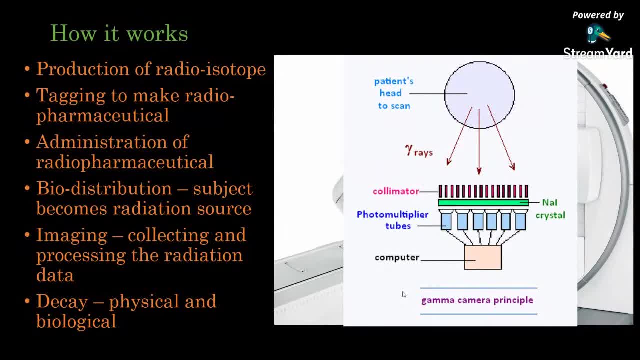 We know that radioactive materials have got a physical decay Based on their half life, And then there is a biological decay as well, which is either the material will be absorbed within the body or it will be flushed out through our fecal matter or through urine or sweat or any of these. 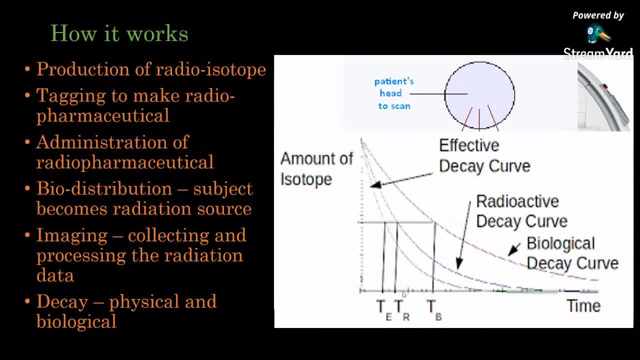 And that comes out of the body. So when you look at that- the amount of isotope comes or decreases as time pass- You can see that is a biological decay curve which is in red. The radioactive decay curve Is in purple. 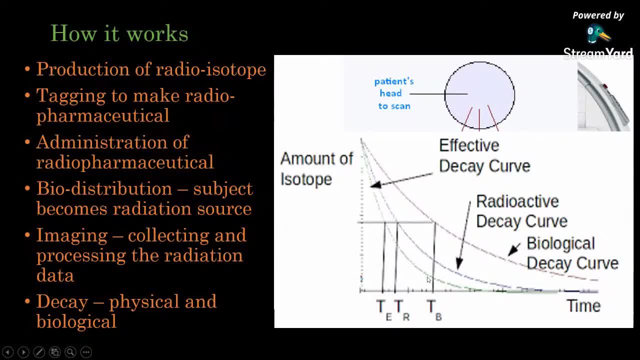 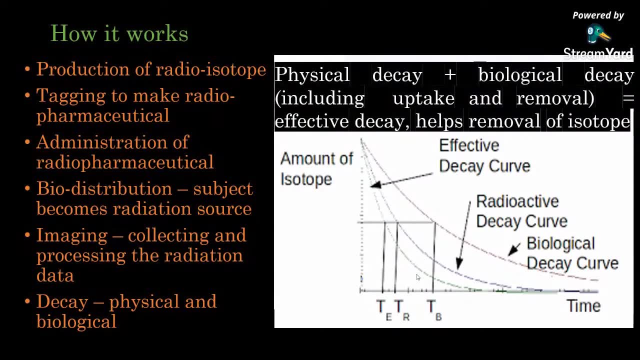 And then there is an effective half life or the effective decay, which is a combination of the radioactive decay and the biological decay. So the physical decay plus biological decay. It leads to the effective decay which helps in the removal of the isotope from the from the body, once the imaging procedure is completed. 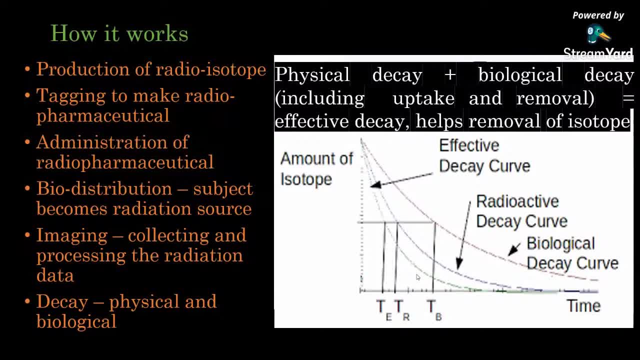 Whereas in therapy we do not expect the the isotope to be flushed out of the body quickly, because we want that isotope to be absorbed by the particular organ having cancer And then we want it to treat. So that is the aim, Whereas in imaging we want as soon as imaging is completed. 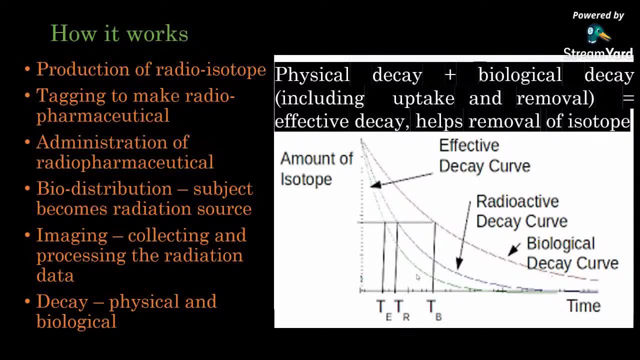 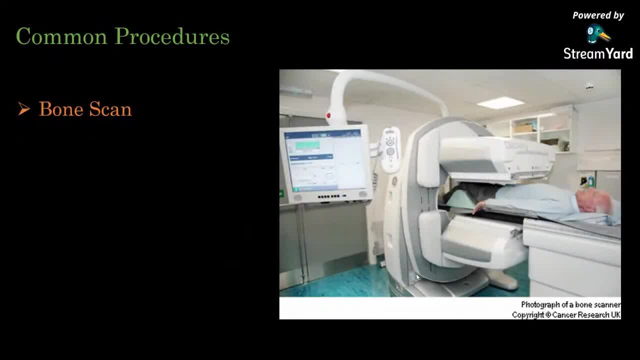 we want the isotope to be flushed out of the body to reduce the dose to the body. Some of the common procedures used are: bone scan. We can. that is a very simple scan whereby usually technetium 99 M is administered and to a gamma camera is used to create. 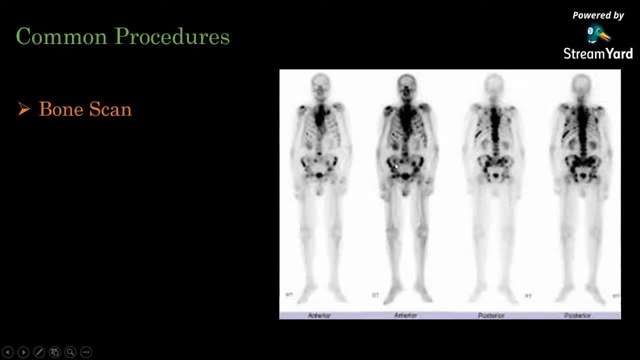 A something called or something called a bone scan image. You can see what is in in in black spots. here are all where the radio sort of went, So some of the absorption is very common. You can see in and around this region where the heart is. 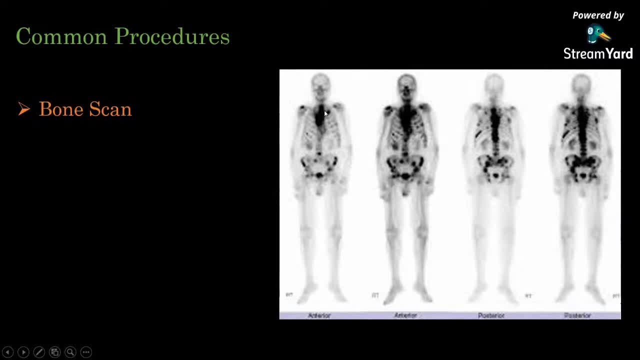 There is more absorption because, as we know, there is a lot of blood that is going in and coming out of the heart. So there will be a lot of radioactive isotope in the heart region, in the bladder region, because of urine collection. 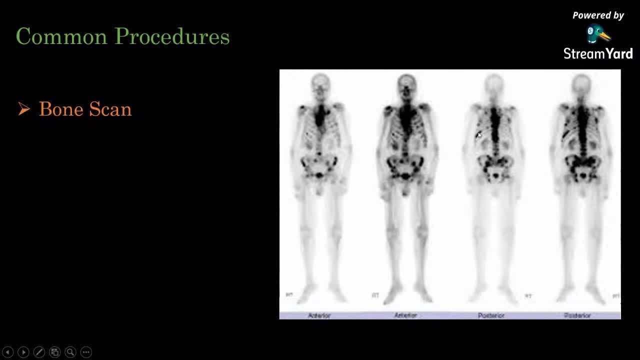 Whereas there There are some uncommon areas. you can see around the rib region here That is not a very common area where the you would find the radioactive isotope uptake. So if you find uptake in uncommon areas, that could be due to the presence of a cancer cell, because cancer cells are 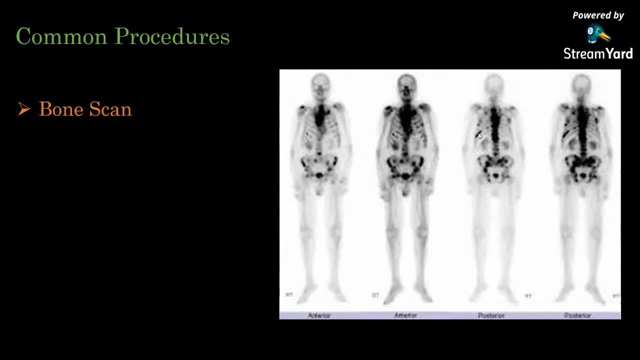 hyperactive and they take up a lot of blood and glucose and all that for their growth. So along with the blood that is being pumped into the cell, the radioactive isotope goes into the cell And that leads to The collection of radioactive isotope in there. 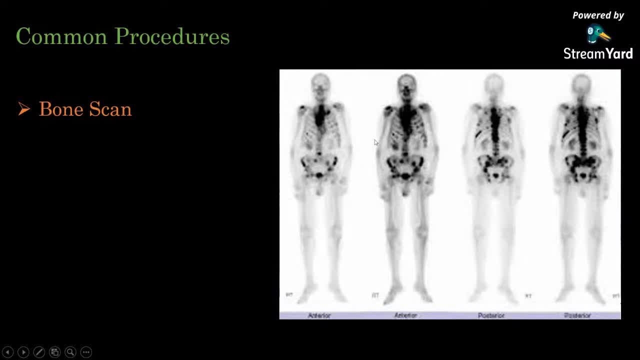 And this is. this is a patient having metastatic bone cancer from a prostate cancer. So he initially had prostate cancer and then that spread into bone and eventually leading into the cancer being spread into the, into the thorax and the ribs region. You can see. 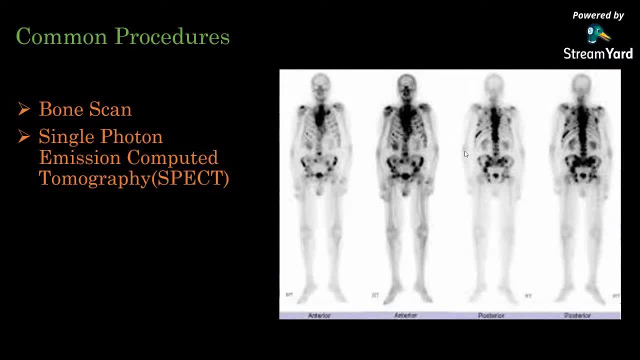 So another common technique is a single photon emission computer tomography. So this is called a SPECT scan. It is slightly different, because bone scan is more like a projectional radiography. It gives you a squashed projected image, just like our X-ray. 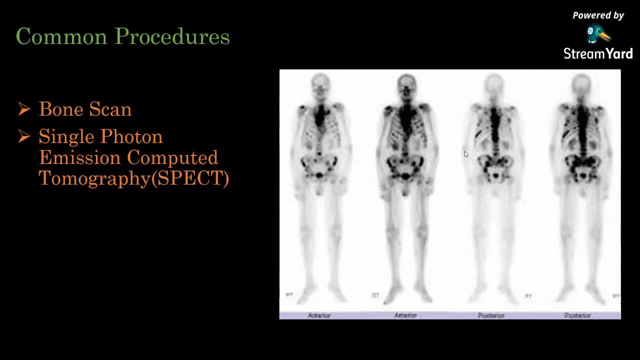 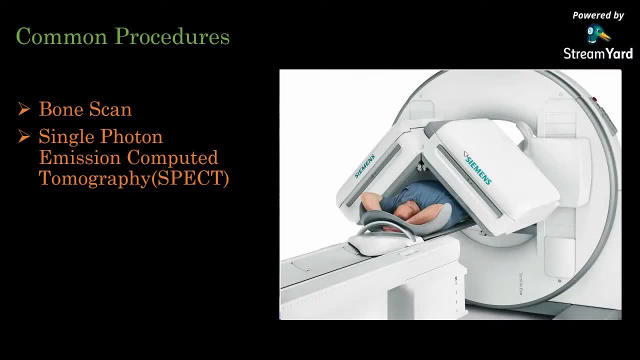 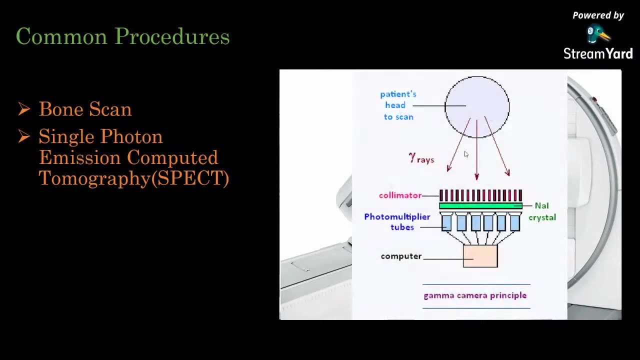 But this is more functional, whereas a SPECT scan is more like. that is why it is called a computer tomography. It it is. it is a three dimensional imaging and it uses a dual gamma camera, and the gamma camera system actually can spin around the subject being examined and it uses the same technique. 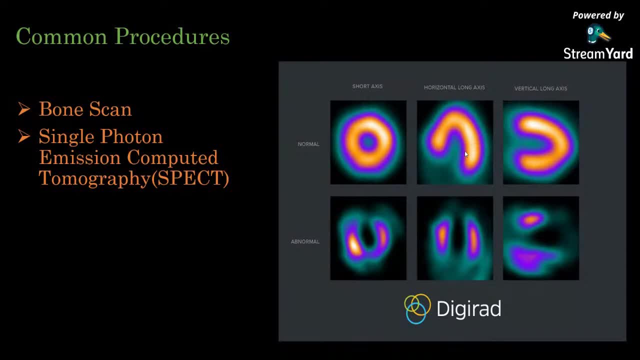 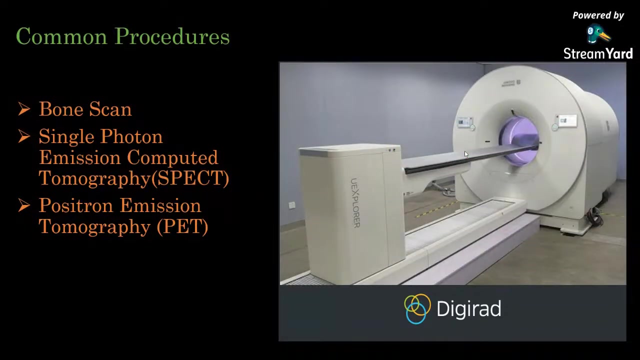 And Comes up with a three dimensional image which is an axial slice, and you can go through slice by slice and see what is going on. The other most common technique is called a positron emission tomography- PET scanning- which uses this is a total body PET scanner. 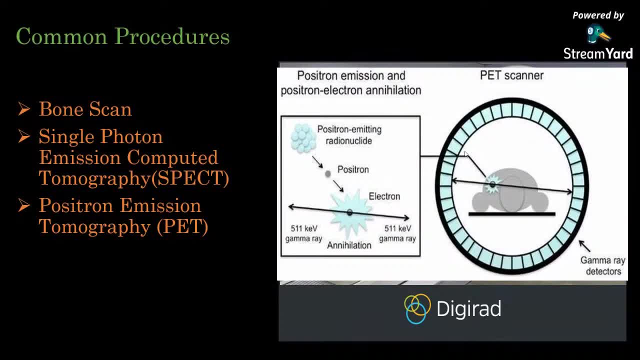 So the physics behind positron emission tomography is that the subject being examined will be administered with something called fluorine 18.. It is a positron emitter, So fluorine 18 is a radioactive material. Then that is tagged with deoxyglucose to form what is called the FDG fluorodeoxyglucose. 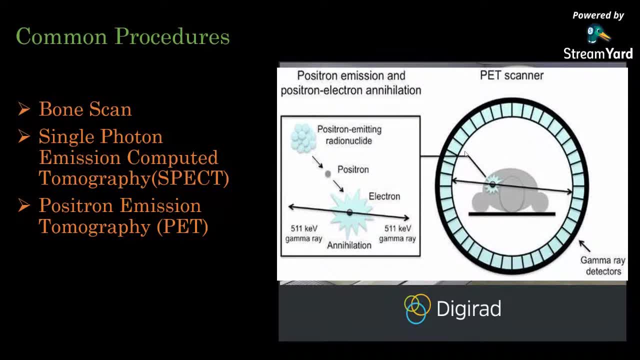 It has got glucose in it. So once that is administered into the body, every cell loves glucose. So the cells that are more active needs more glucose And hence all the cells in the body that is hyperactive actually absorbs the fluorodeoxyglucose. 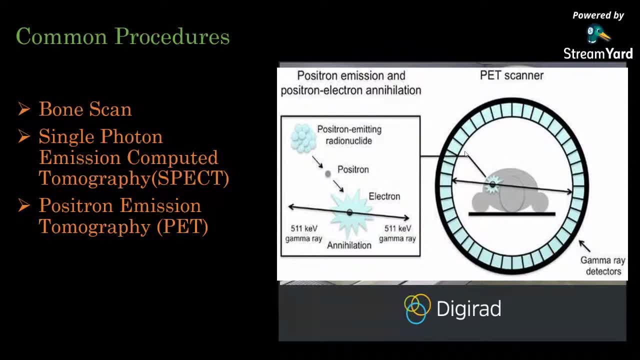 And then the fluorine 18,. once it gets to the cell, the fluorine 18 starts to emit positrons. And when we know that positron is the counter particle of electron, whereby it has got the same amount of charge and mass of that of an electron, but it is positive in nature. 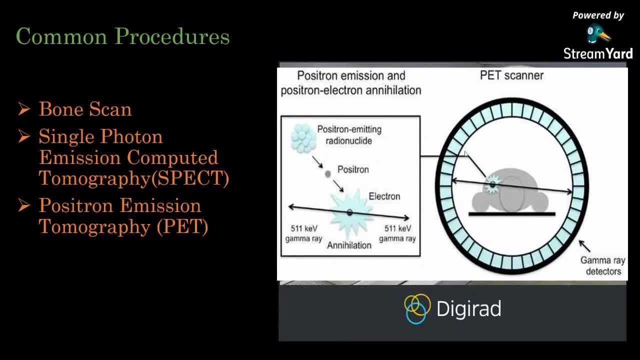 So that is a classic case. when a positron combines with an electron. being antiparticles, The mass of the positron and mass of electron converts into energy as per E equal to MC square, as per the Einstein's famous equation. So mass is converted into energy. 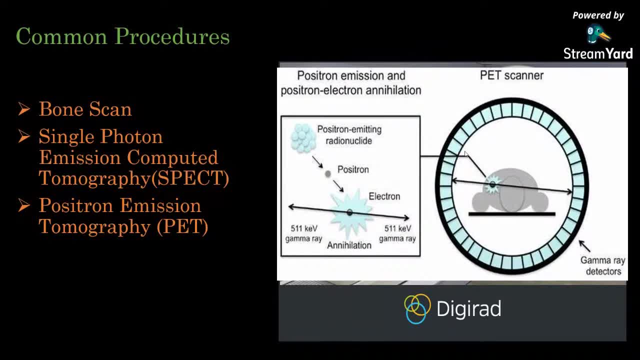 So the rest mass of positron and rest mass of electron is converted into energy And we know that the total rest mass is 1.02 MeV. So it eventually becomes a pair of 511 KeV gamma-ray. So at the end what happened is, within the cell, a positron and an electron annihilate. 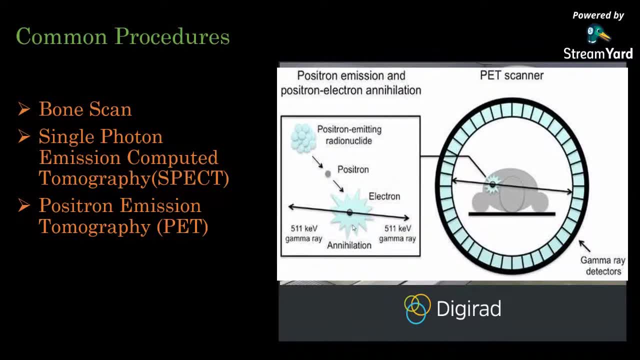 It leads to pair annihilation And the production of two gamma rays, each having energy 511 KeV, and they will be emitted in 180 degree direction. And then that is detected. Those 511 KeV photons are detected by special detectors and it is converted into image leading to positron emission. tomographic images. 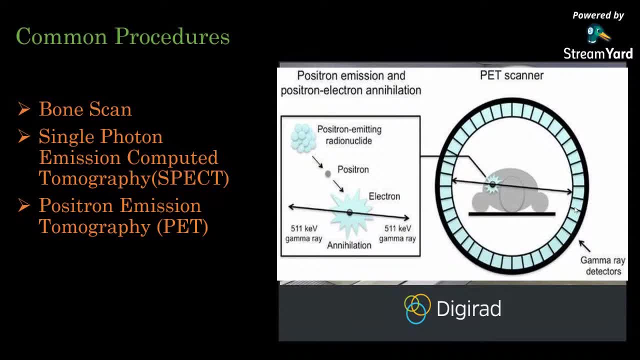 The advantage is this is highly effective in cancer imaging because we know cancer cells are hyperactive and they selectively absorb the FDG or the fluorodeoxy glucose, And hence this is very, very, very sensitive to cancer imaging or cancer cells And we can pick up cancer cells way more than what CT scans and MRI scans can. 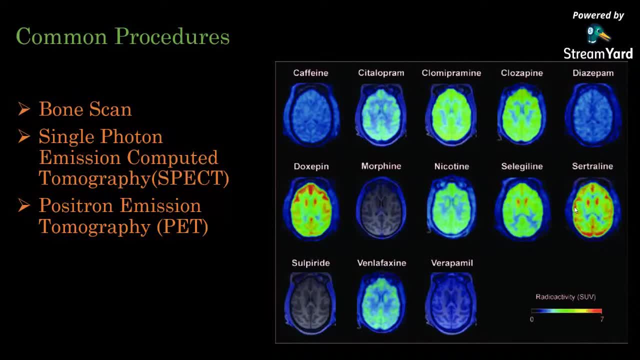 So this is how a PET image will look like, depending on the the material that you have taken or depending on different chemicals that people use. So if you use caffeine, this is how your brain look. If you take other medications, you know, you can see the amount of. 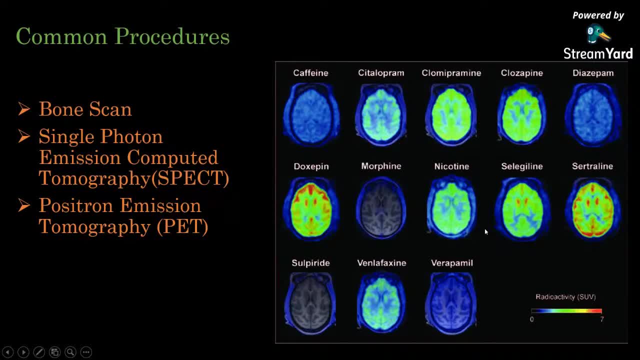 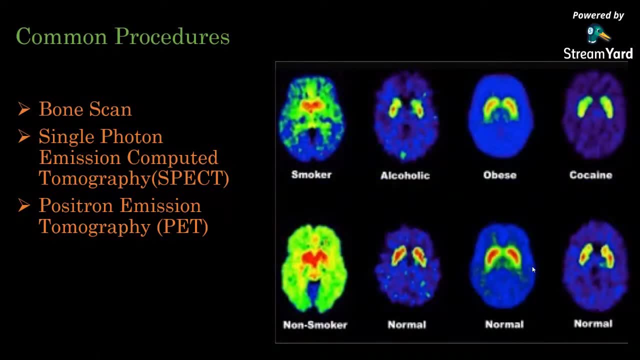 glucose that goes into the body changes And this is how. this is a classic example of how the uptake is different based on how your brain works. And this is how the brain works, depending on your habit. These are all PET images you can see between a nonsmoker and a smoker. 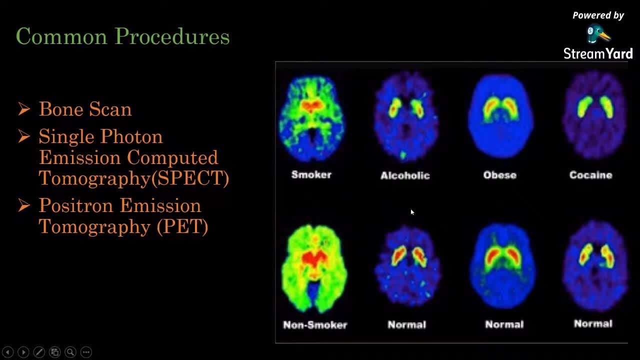 In a smoker's brain the blood flow is actually less between an alcoholic and a normal person. You can see between an obese and a normal person, between someone who has been in the influence of cocaine and a normal. So this is not just for oncology. 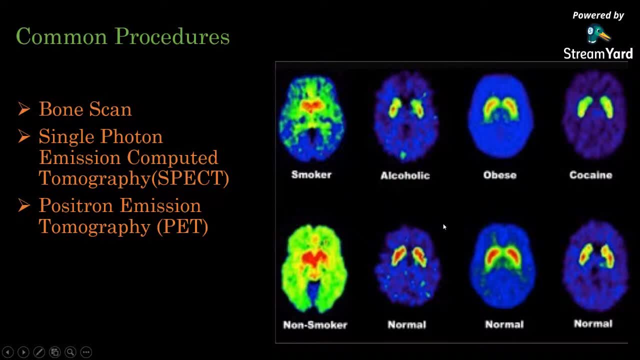 This can be used for brain function studies as well. Hence I said this is more to do with functional imaging. Other I would- I'm almost towards the end of my talk. Other very, very common and interesting technique is myocardial perfusion scan. 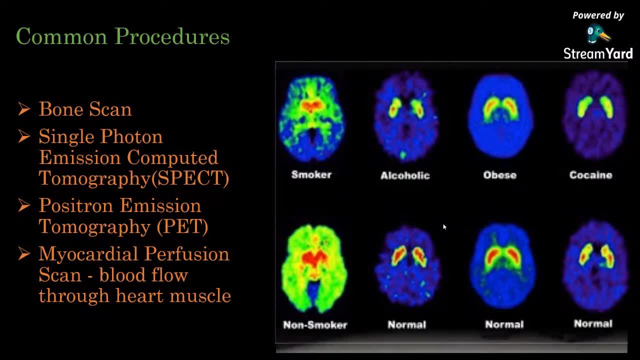 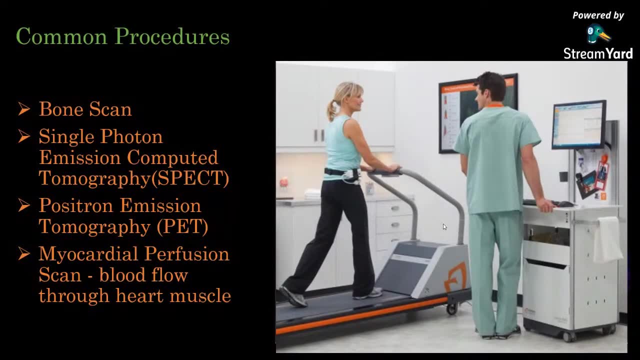 Which study the blood flow through the heart muscle, And this is whereby the subject being examined will be on a machine like a treadmill, And then they will have system, maybe the radioactive radiopharmaceutical administered into their body, and then myocardial perfusion scan is done. 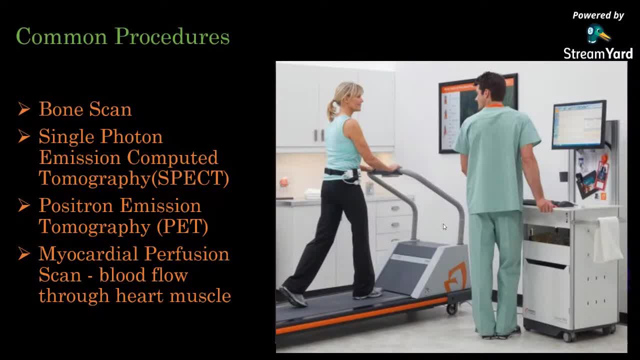 which is more the imaging of the heart, to see how the blood flow is inside the heart, And this will help in identifying possible heart attack or how the cells work after a heart attack has happened, If there is any potential for a subsequent heart attack to happen. 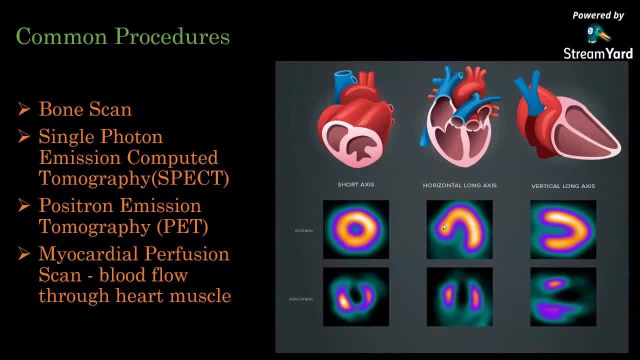 So these are all some of the very common imaging technology used And you can see these are some of the. this is what happens when the heart is normal. This is how the blood flow. This is an abnormal heart in different axis, you can see. 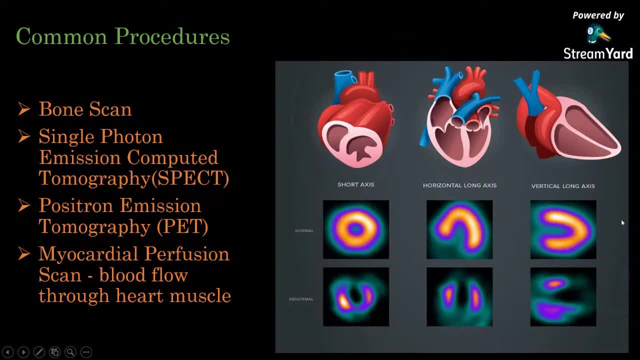 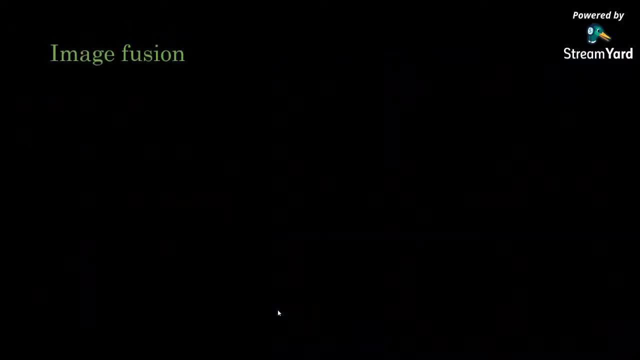 So the blood flow is clearly different in an abnormal heart compared to a normal heart. So this gives a good indication of the health of the heart and a potential myocardial infarction. We use image fusion to better understand, as I said: CT and X-rays and MRI scans- all 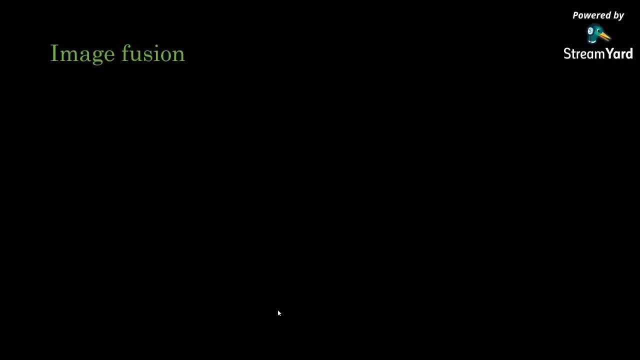 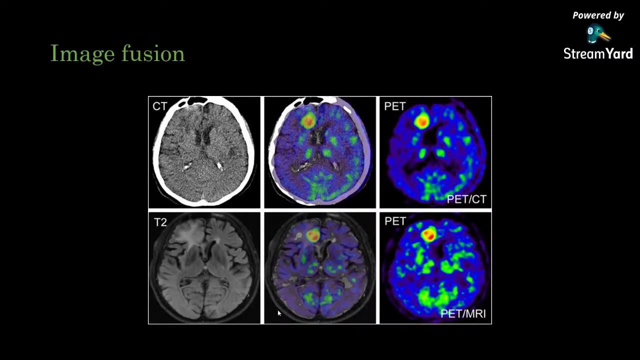 give anatomical imaging, whereas nuclear medicine provides more of a functional imaging. But if we fuse the images we get a much better idea, because nuclear medicine scans doesn't give any indication of the anatomy, It just gives about indications of the functional aspect of the organ. 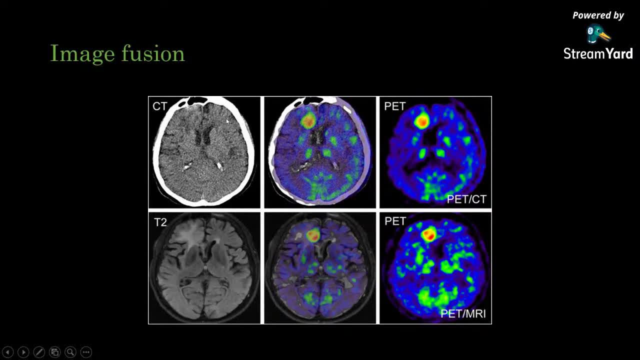 So when we fuse the images together, you can see that's a CT image, That is a PET image and that's a PET CT image. So this is a PET CT image and that's a PET only image When you fuse them together functionally and anatomically. 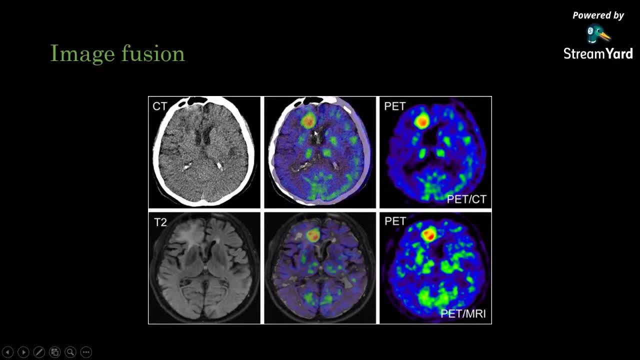 you can find out what is happening in the brain and where is happening in the brain. That is an MR image And that is a PET image. When you fuse them together, you get an MR PET. You can do MR PET, you can do CT PET. you can do MR CT PET. 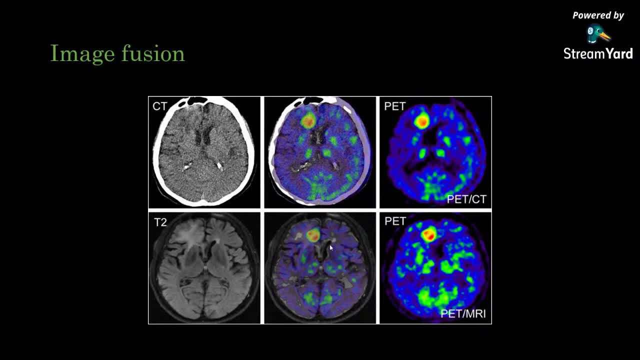 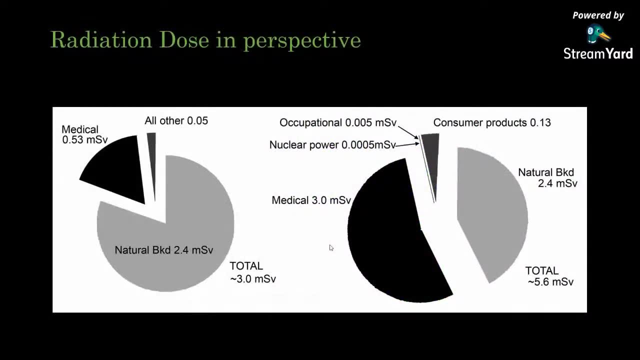 So all sorts of image fusion is possible. That gives an extremely good clinical indication of what's happening with different parts of the body. But this does not come for free. It is at the expense of some radiation dose. If you are not careful when I say you, not the person being examined, the people who are 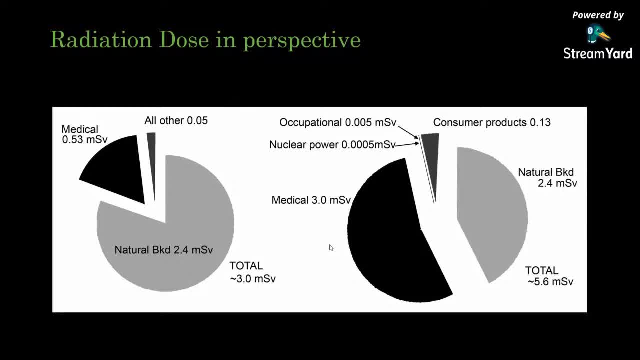 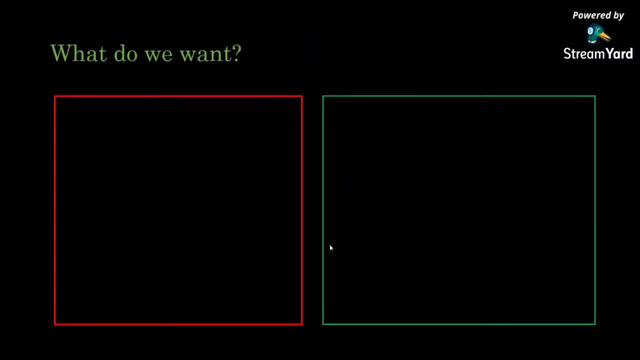 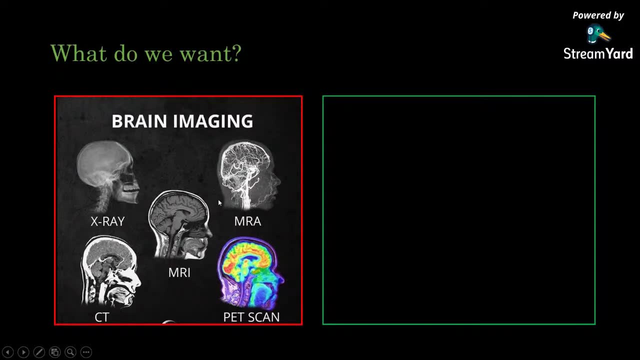 working in this area is if they are not careful about the the use of the technology, then that can lead to very hazardous effects. Something like we actually want, this Like this, is the X-ray image, CT image, MR image. This is an angiogram. This is PET scan. 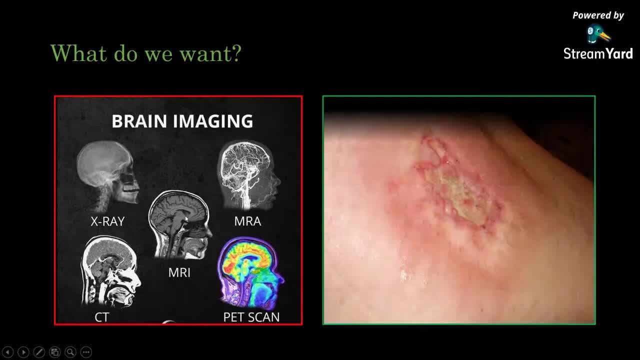 You can see all this. This is all really good, but it should not be at the expense of this. This is what happens: if you're not careful and if excessive radiation gets into the body, it can lead to damaging effects. So we don't want what is in the in the green box. 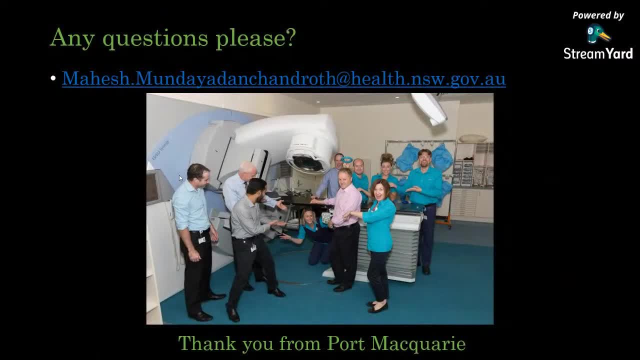 We rather want what is in the red box. And with that, thank you so much. I think I have taken a few extra minutes. Apologies, And that's all from me for today. Thank you, Thank you, sir. Thank you so much. 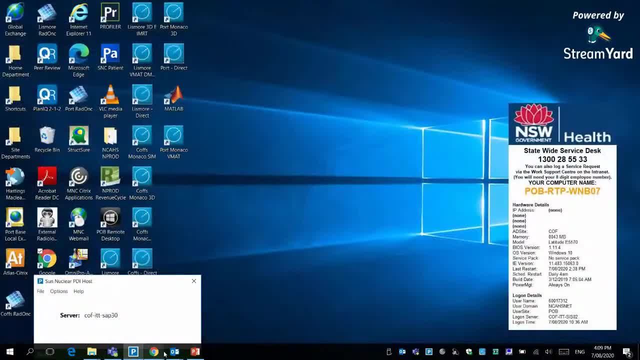 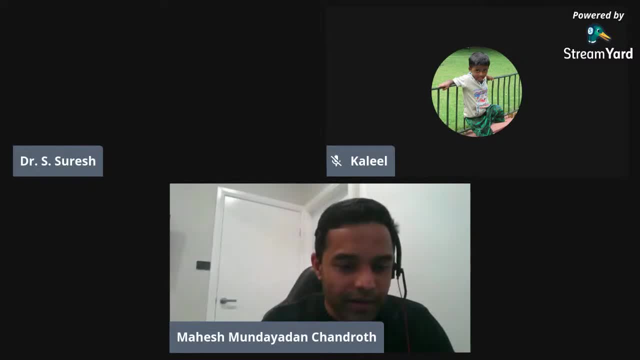 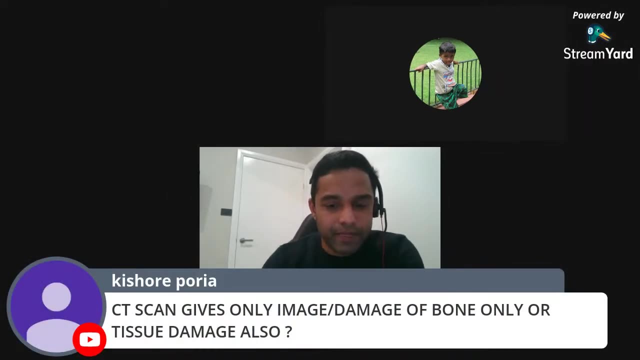 And now Hello, Yeah, fine sir. Now, Hello, sir, Can you hear me sharing the screen? Yeah, I can hear you. Can you answer a few questions? Oh, yeah, Oh, for sure. So Kishore Puria has asked a question on. 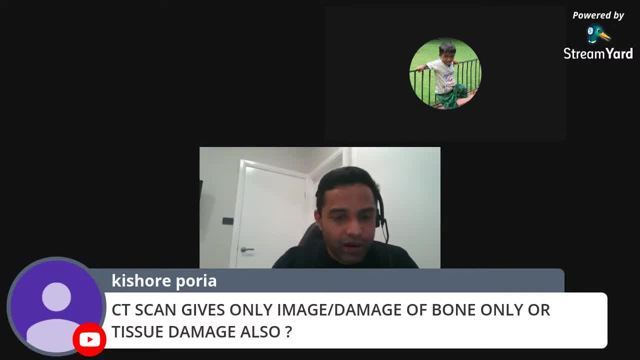 PET scan gives only image or damage of bone only, or tissue damage. Also, as I said before, PET scan can give only image or damage of bone only, or tissue damage. Also, as I said before, CT scans can provide a comprehensive image of bone as well as normal tissue. 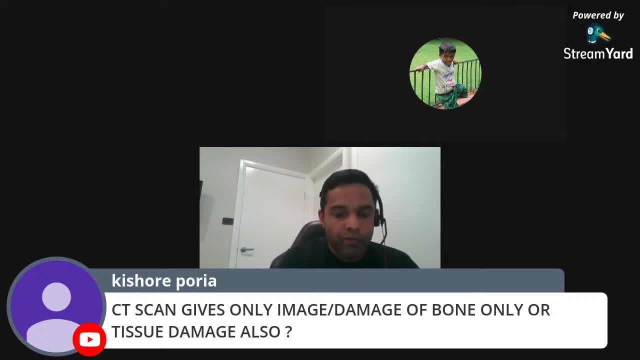 So When, as I alluded to in the in the session, you can see that when X-rays- planar X-rays- are used, it actually gives a good contrast for the bone And soft tissue contrast is actually very, very low. 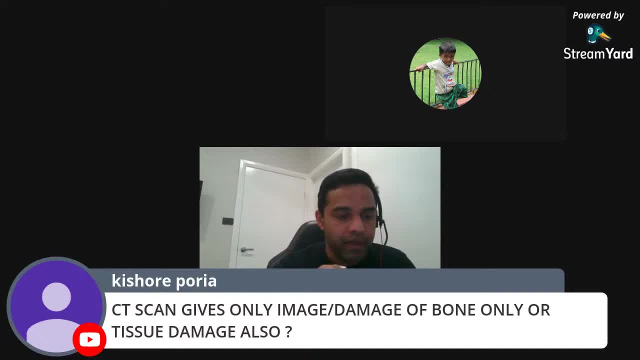 You cannot see all the other normal organ very clearly. You can to some extent, but not as much as the CT scans give. CT scans are axial slices which gives a good indication of bony anatomy, including, like the spine and and all the ribs and all that. 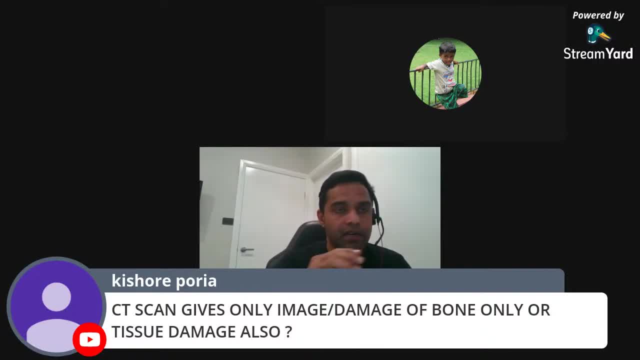 And if you're doing around the pelvic region, it gives you a good indication of your femur, the pelvic bone, the leg bone and the whole pelvic anatomy. It gives a good indication, but not just the bone, It can show you everything, all the organ that is in the pelvic region. 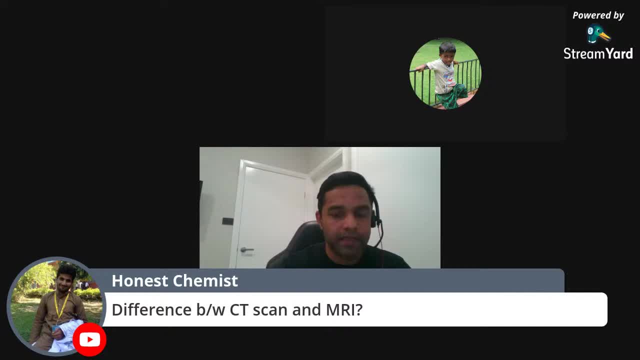 So, yes, it can provide clear image of the of the normal tissue and as well as if there is any tissue damage. but, as I said, it is limited. That is why functional imaging, like nuclear medicine imaging, is helpful in better understanding what is happening with the functioning of these. organs. So difference between CT scan and MRI scan. Yeah, that's a really good question from a from a simple point of view. CT scans use radiation, whereas MRI scans do not use radiation. It instead use the magnetic resonance imaging technique. So it is the magnetic resonance property of materials within the body. 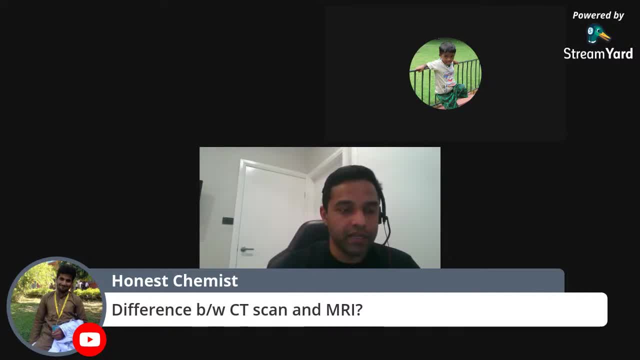 especially the hydrogen that is in the body is utilized in coming up with MRI scans. So the advantage is: with MRI scan, things like or organs like brain can be imaged with a very, very, very good contrast. You can see a much better picture of the brain or other organs in the body using 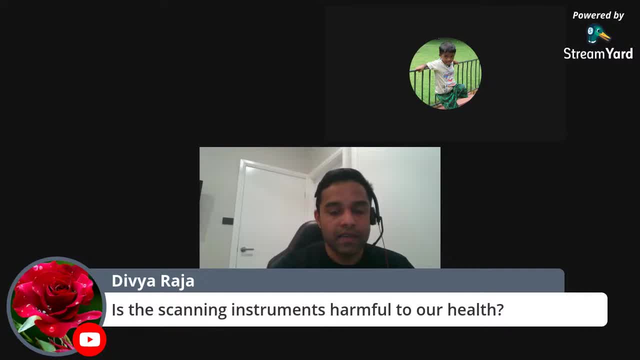 MRI scans and then CT scans. So MRI images are actually better quality image than CT images and they do not have radiation risk, which CT scans do have. So that is the basic, very fundamental difference between the two scanning technique. TVR Raja has asked another question. 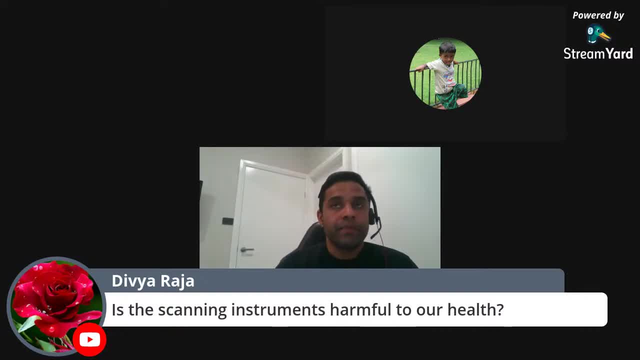 Is the scanning instruments harmful to our health. So, as I said, every precaution is taken before such procedures are done in medical facility. There are from the time these equipment is manufactured To when it is installed in hospitals or scanning centers and for day to day. 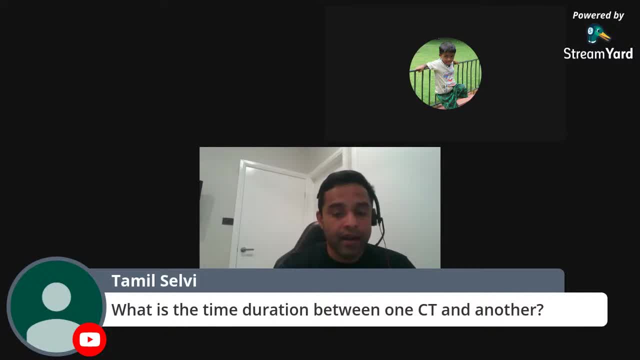 procedures. there are strict protocols and guidelines to reduce the dose and radiation damage. So in medicine what we always look for is the comparison between risk versus advantage. So if by taking a very, very small risk of having a very, very low radiation dose, for example, 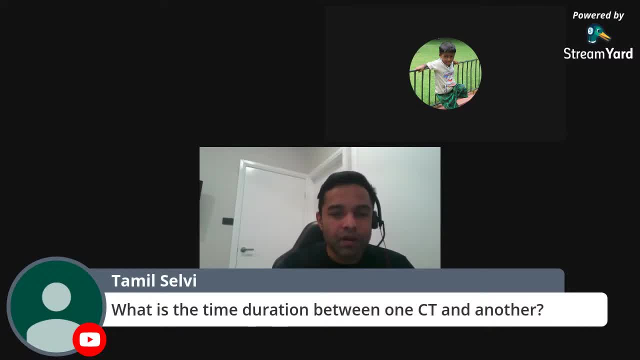 someone present to the hospital with a possible fracture of the bone. someone fell down and thinks that the bone could be fractured. The patient is in real pain. Would you actually want to be undergoing a CT scan or an X-ray to see what exactly happened and undergo 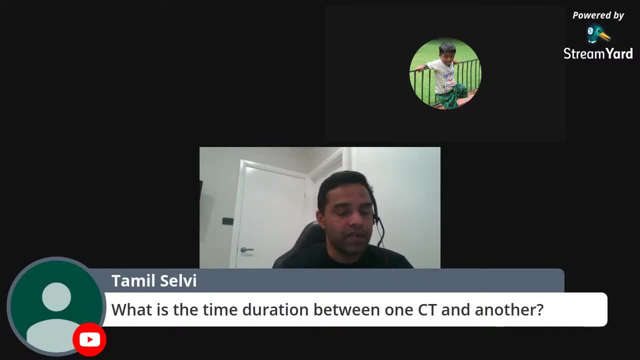 a surgery and fix it, or worried about the radiation dose and not to do any procedure and end up in complication. So the practice should be justified whereby the clinical benefit should always be higher than the risk. Then only we do the procedure. What is the time duration between one CT and another? 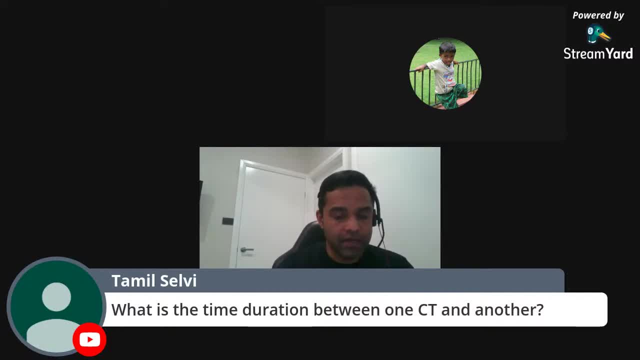 You mean for the same? I understand Tamil Selvi has asked the question. I understand the question is for the same person: how long you should wait before two CT scans are done. Actually, the amount of radiation dose in a CT scan is actually very, very low. 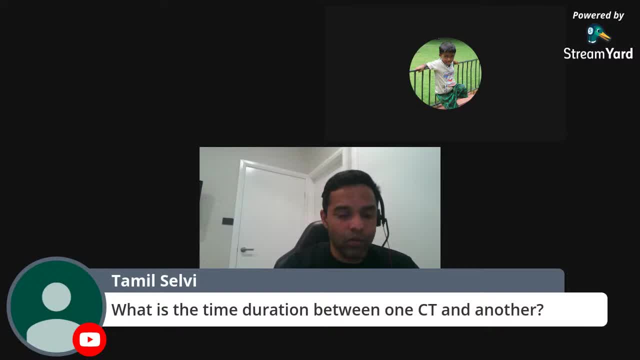 It is not as high as we think, or we think in terms of radiation treatment for cancers. It's an extremely high dose compared to the scanning dose or the imaging dose. So, again, a CT scan was done today and the radiologist or the doctor who looks 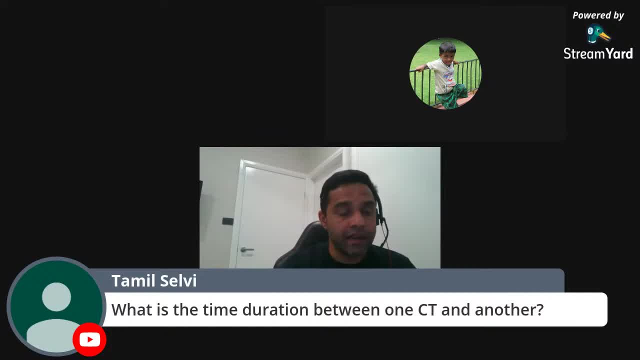 through the images have got some doubt and the patient is in some pain or is in some in complicated condition or have to have a repeat scan tomorrow or on the same day, It doesn't matter. We do re-scan our patients quite often to get a better understanding of what's happening. 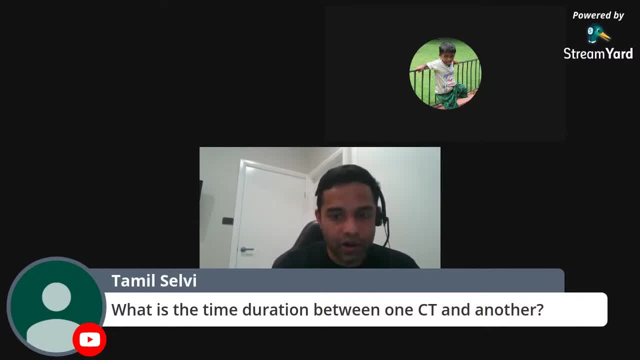 So two scans on a day is not is not a big deal, But that doesn't mean you want to go and do two scans every day for a week. Now. that is probably not quite quite beneficial, but a couple of scans a day is. 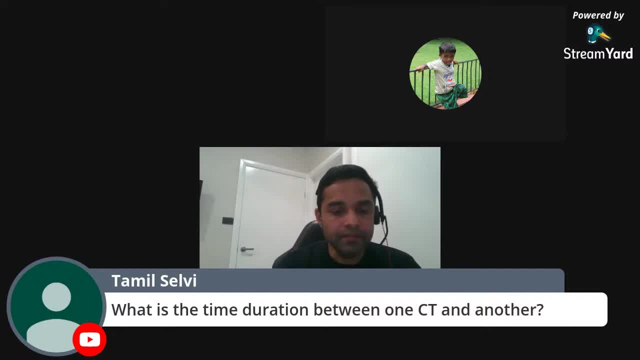 OK, OK, so there is another question from Lalan Kumari. I have asked: MRI gives only anatomy information or physiology as well. So conventional MRI provides anatomy only, But there are new technology which is called the functional MRI. They can provide functional imaging or physiological imaging as well. 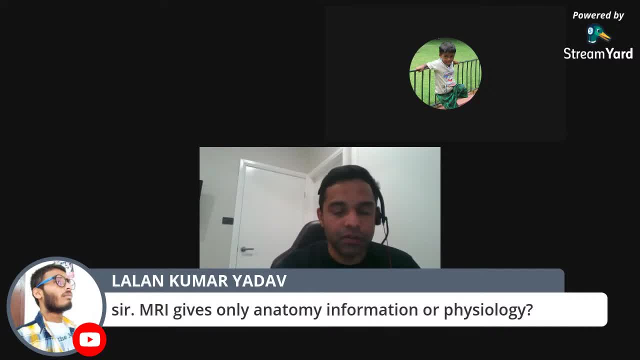 So, yes, modern day technology Actually gives indication of the brain functioning or function of the organ. Yes, Thank you, sir. I call upon Mr Khalil Muhammad Ibrahim to give a word of thanks. Thank you, Thank you. Good morning to everyone. 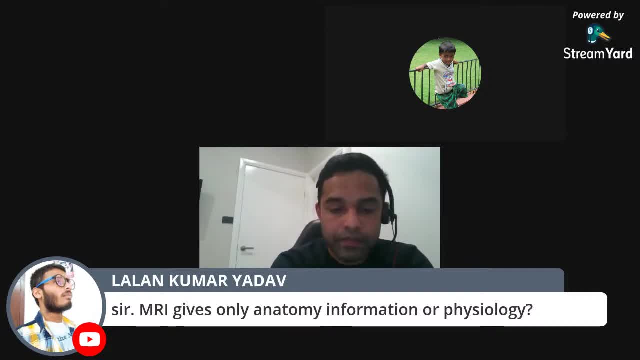 I am honored to have the opportunity to give a word of thanks on the end of a successful webinar. on behalf of the Department of Science, St Joseph Engineering College. I take this opportunity to deliver the word of thanks. first and foremost, We would like to express my profound gratitude and very special thanks to our 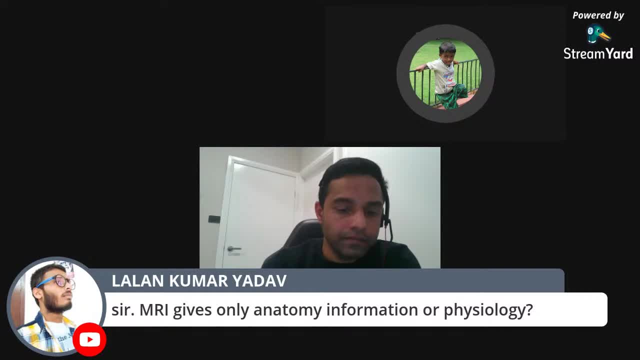 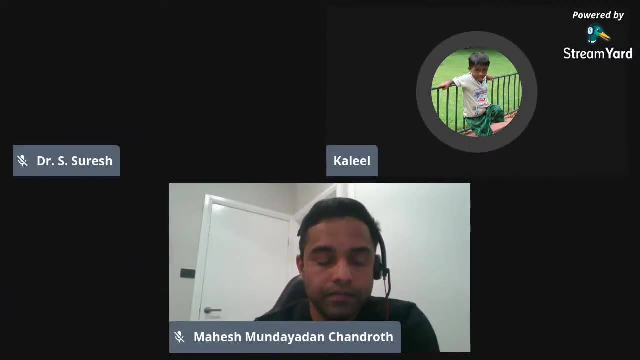 most respectable chairman, Dr B Bob Monoran, St Joseph Group of Institution for his constant encouragement and providing an inspiring environment for such educational developments. I would like to express my deep appreciation and sincere gratitude to Mrs B Desipriya, Madam Managing Director and Mr. 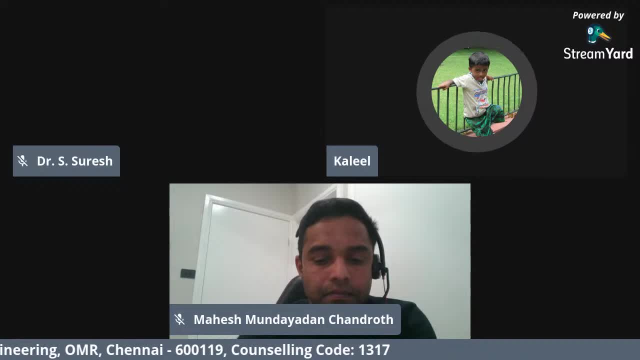 B Sasegri Rao, Principal, Dr B Parvada, Vatanim Dean, for their support towards this event. At the outset, I thank our chief guest and resource person, Dr MC Makesh, who has readily accepted our invitation in spite of his busy